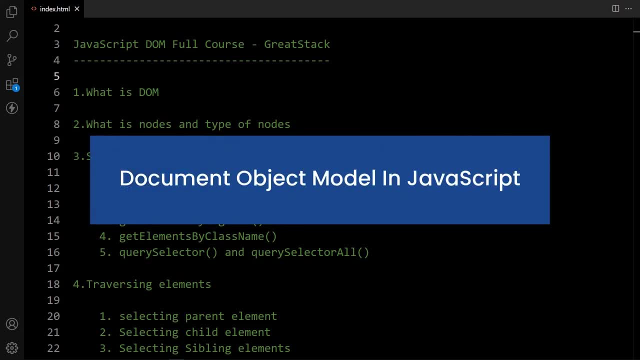 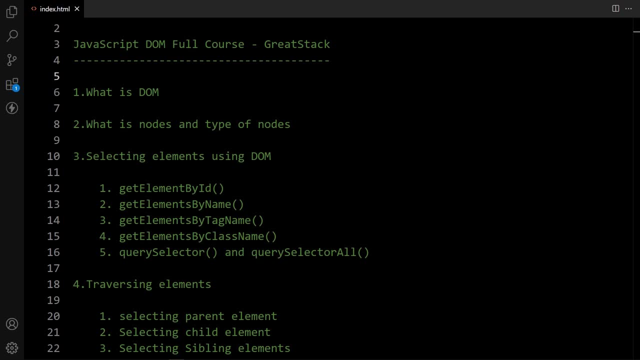 In this video we will learn about Document Object Model in JavaScript. You will learn all concepts of JavaScript DOM with example. Here are all JavaScript DOM topics that we will learn in this single tutorial. We will learn about what is DOM, what is nodes and type of nodes. Then we will 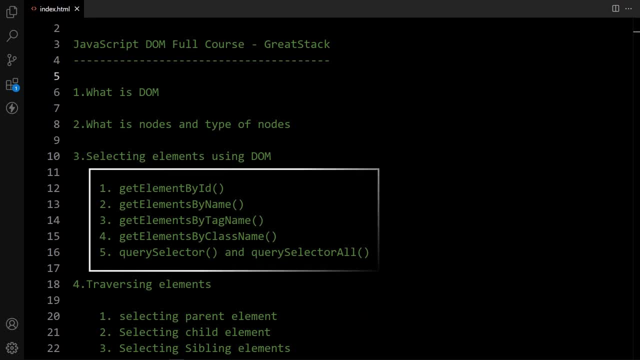 learn selecting elements using these methods, which is getElementById, getElementsByClassName, getElementsByTagName, getElementsByClassName, then querySelector and querySelectorAll. After that, we will learn about traversing element, where we will learn about selecting parent element, child element and sibling element. After that, we will learn about manipulating the HTML. 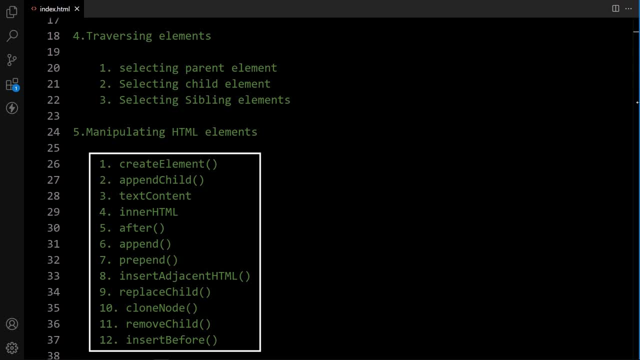 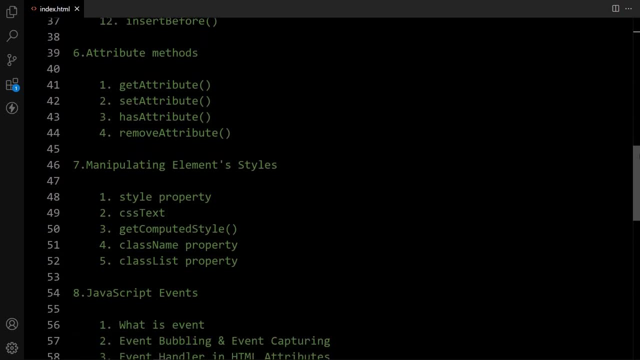 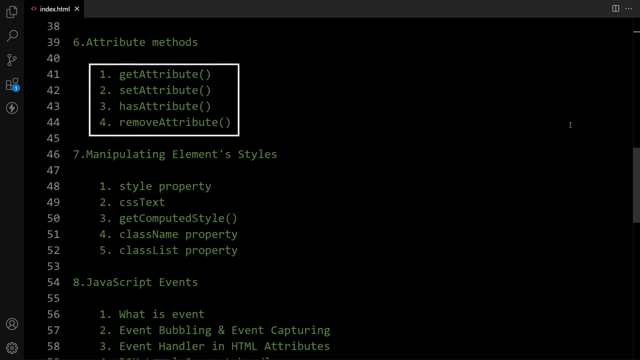 elements, where we will learn to create an element using createElement method, Then append child text content and all these methods. After that we will learn about attribute methods, where we will learn about get attribute, set attribute has attribute and remove attribute. After that we will learn about manipulating. 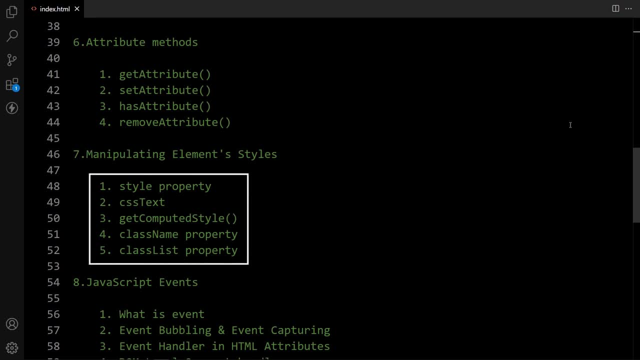 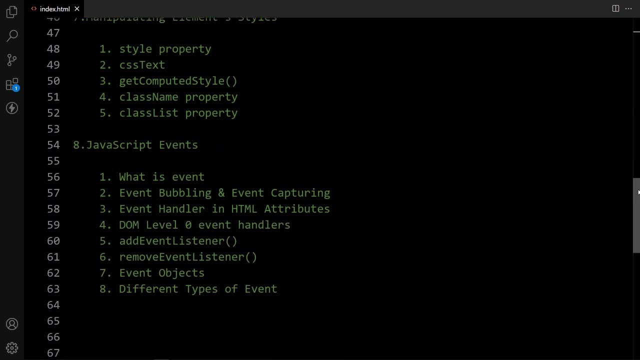 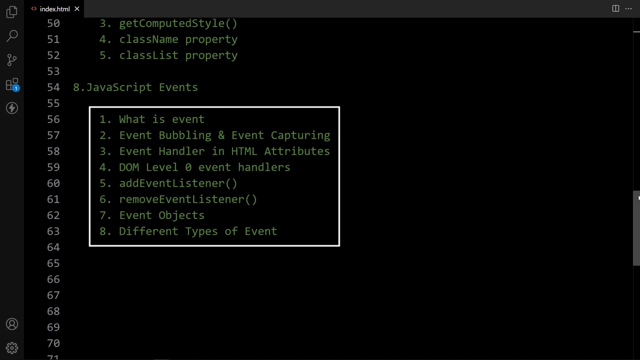 elements. style using style property, CSS text, getComputedStyle, className property and classList property. After that, we will learn about JavaScript events, where we will learn about what is event, what is event bubbling and event capturing. how to handle the event using event handler attribute. 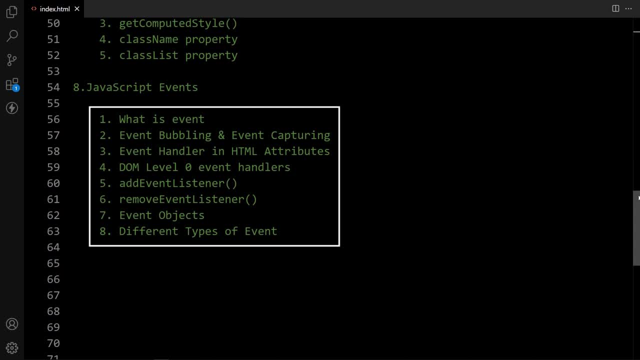 Then we will learn about DOM level 0 event handler. Then we will learn about add event listener and remove event listener. Then we will learn event objects and different type of events. So before starting this tutorial, please hit the like button and also subscribe my channel. 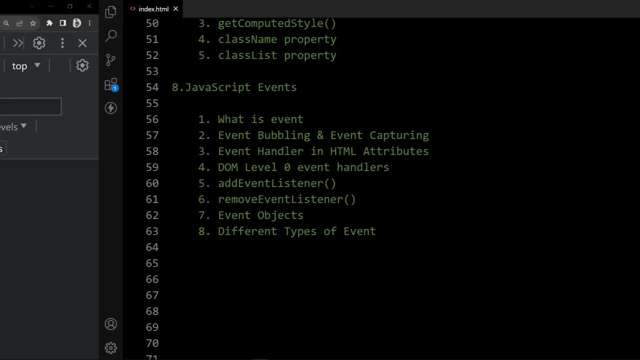 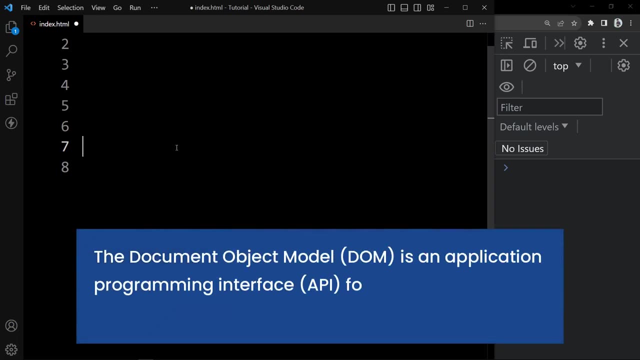 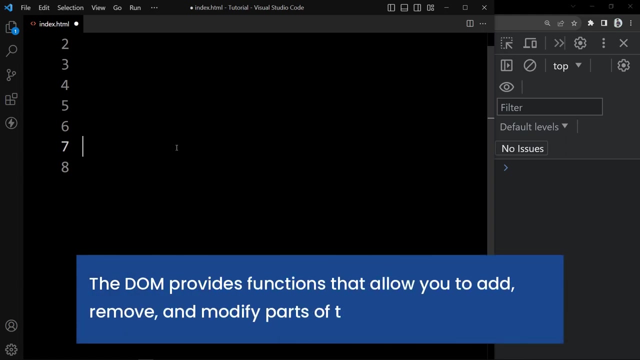 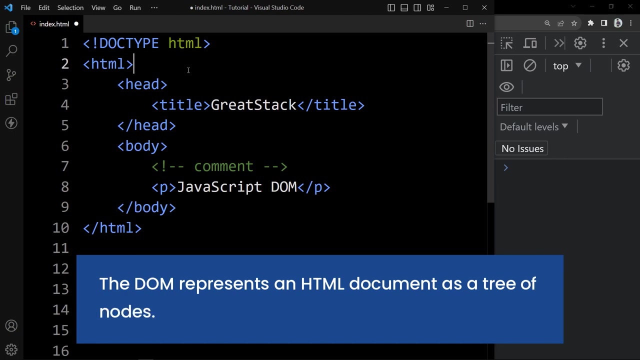 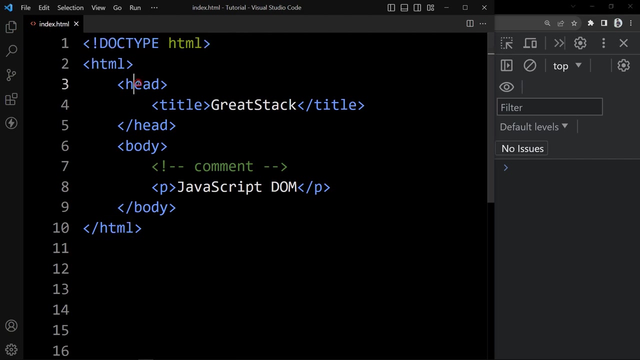 GreatStack. Now let's start the video. However, I want to use something which is document object module to make JavaScript easier for้, So we will learn about document object model. The document object model is an API for manipulating HTML documents. The DOM provide functions that allow you to add, remove and modify part of the document effectively. The DOM represents an HTML document as a tree of nodes. 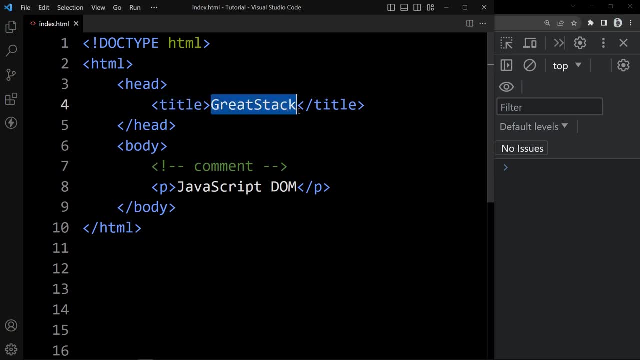 In this HTML code you can see: this is the node. This HTML tag is a node. This head tag is also one node. This title tag is a node. this text greatest tag is also one node. this body tag is a node, this comment is a node and this p tag is also a node. 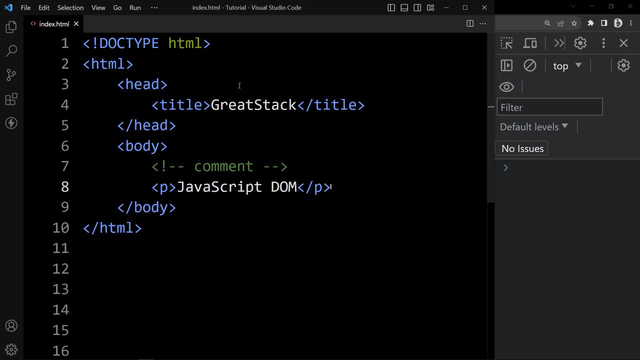 Now let's understand about the node type. So this one is the document type node. These HTML head, title body, these are the element type node and these texts are the text node And this is the comment node. Now let's learn about node relationship. 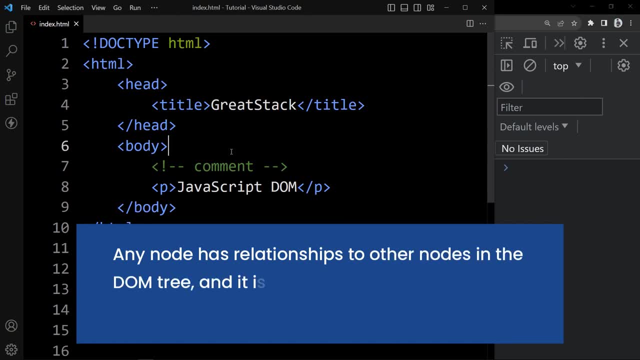 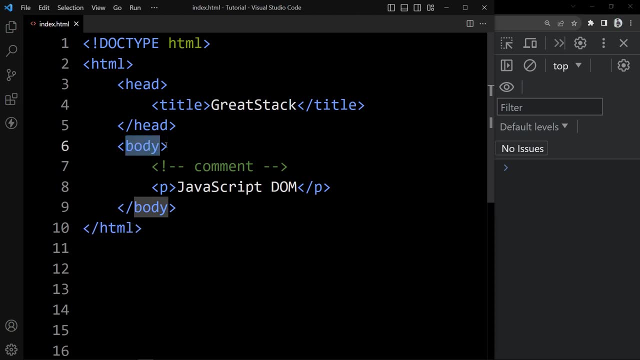 Any node has relationship to another nodes in the DOM tree and it is same as described in the traditional family tree. For example, this body is the child node of this HTML node And this HTML node is the parent node of this body node. This body node is the sibling of this head node. 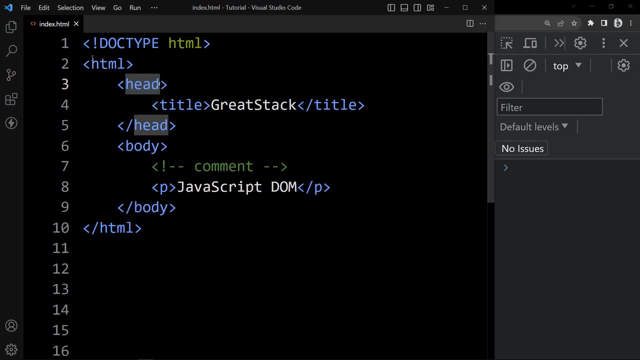 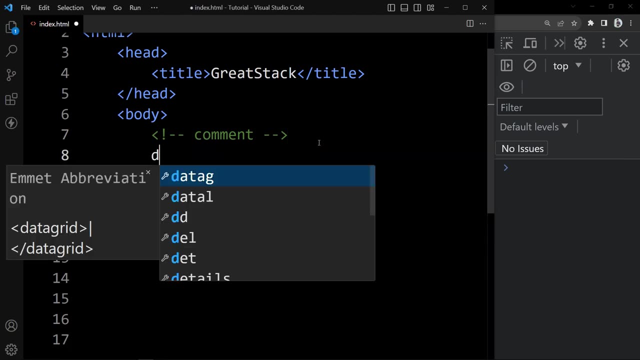 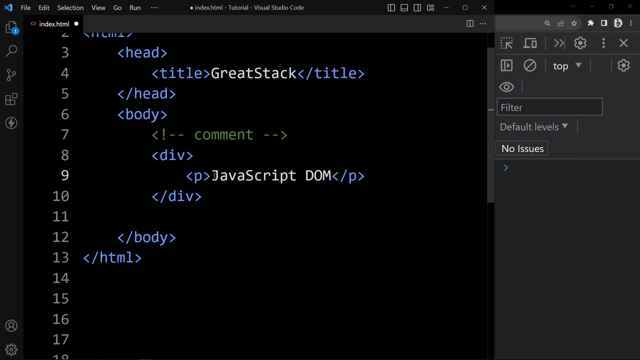 Because they share the same immediate parent, which is HTML element. Now let's add some other content within this body. Here we will add one div And add this p tag within this div. Let's duplicate this, So we have four p tags in this div. 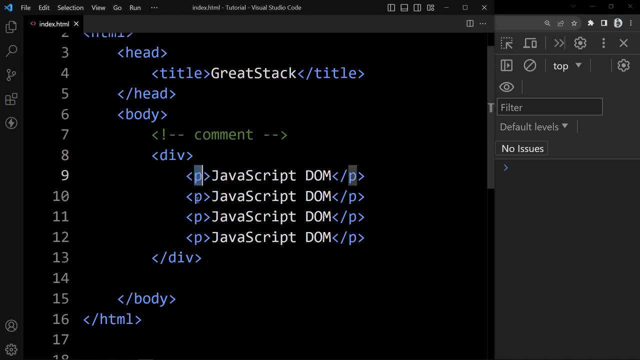 So this div element is the parent node of these p tags And the p tag is the text And this p tag is the child node of this div. This one is the first child And this one is the last child. This second p is the next sibling of the first one. 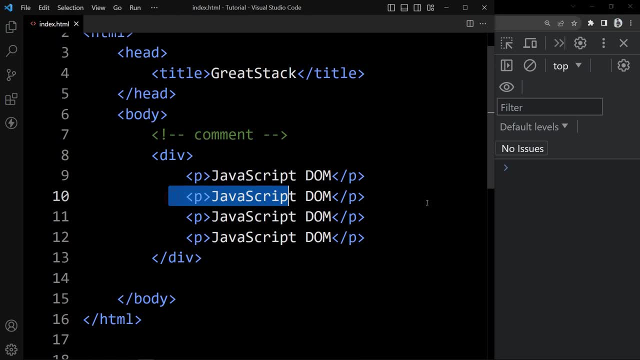 This third p is the next sibling of the second one, And the fourth one is the next sibling of the third one. In same way, you can say: the first one is the previous sibling of this second p. This second p is the previous sibling of third p. 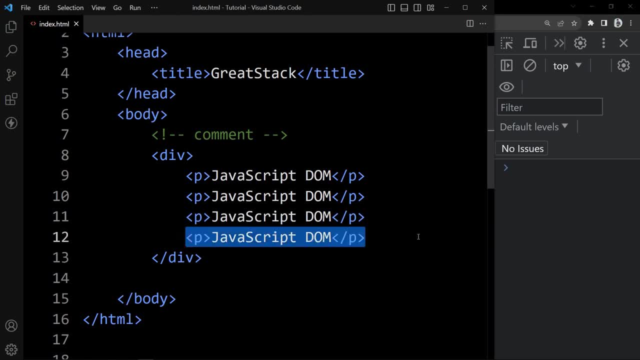 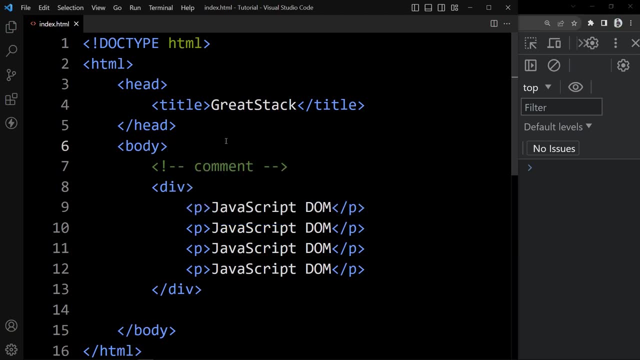 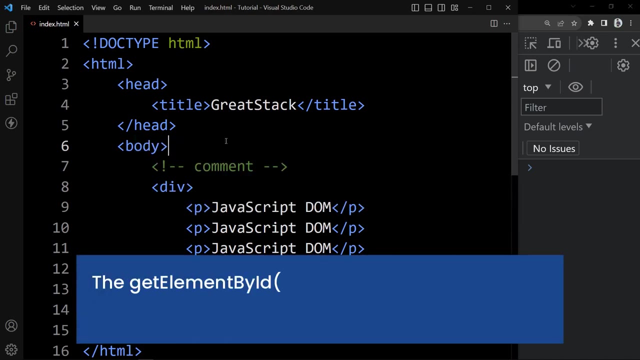 And the third p is the previous sibling of fourth p. Now let's learn about selecting elements using DOM. To get elements in JavaScript, there are various methods in DOM, So the first one is GetElementById method. GetElementById method returns an element object that represents an HTML element. 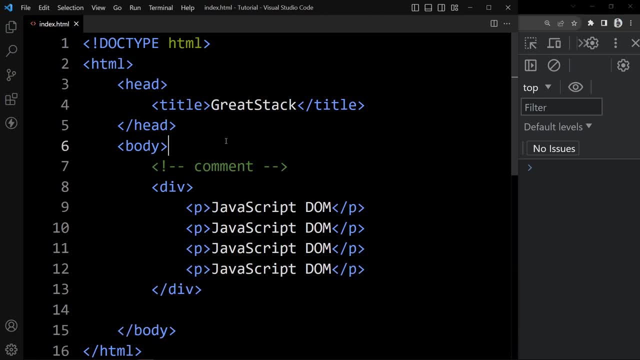 The GetElementById is only available on the DOM. This is the document object. Let's understand this with one example Here. I will remove this comment And I will add only one text in p tag. And for this p let's add one id. 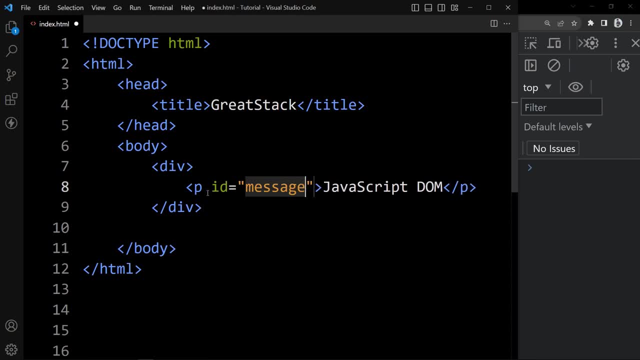 So I am adding the id message And in this p we have the text javascript DOM. Now let's add the JavaScript in this HTML page using the script tag. Within this script tag can add our javascript code. here we will add one variable with the name msg, which is message. 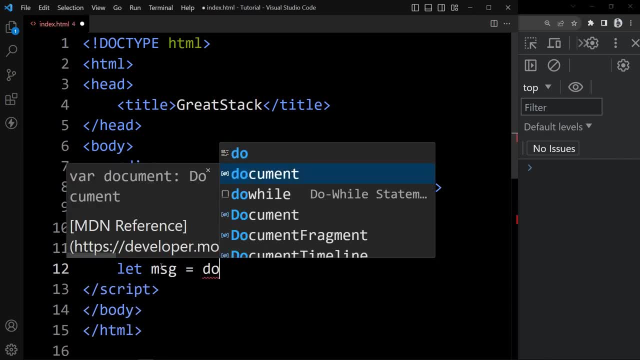 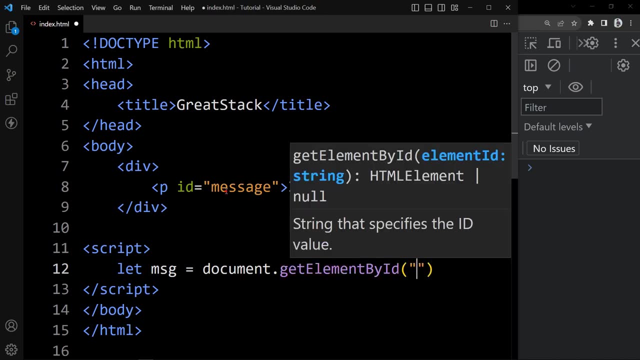 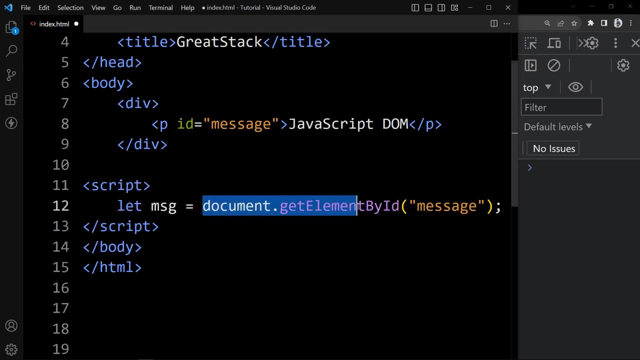 and we can write document dot get element by id, and here we have to add the id of this element, which is message. so this document dot get element by id will select this element and it will be stored in this message variable. now we can print it. let's add console dot log msg. 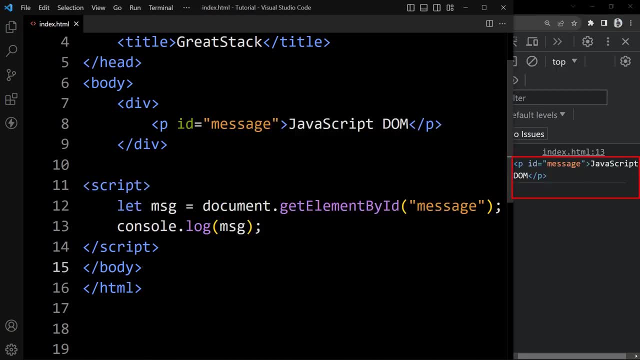 here you can see the output in console tab: pid message, javascript DOM. so this element is printed in this console because I am adding console dot log msg. so in this msg variable we have stored this element which is in the p tag. if the document has no element with the 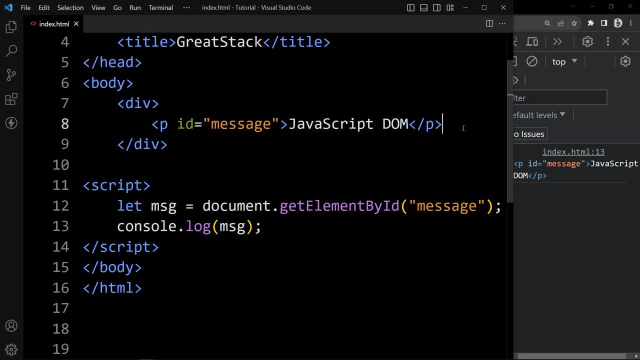 specification. let's say that now we will bring it in. we will bring it in מפ. so in this msg variable we have stored this element which is in the p database between the ID. then it will return null. suppose there is no element with this ID on the web page. 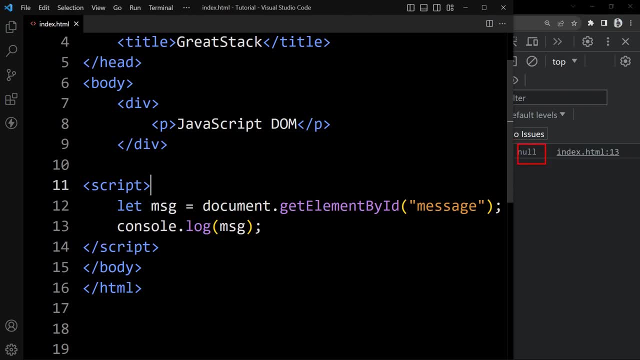 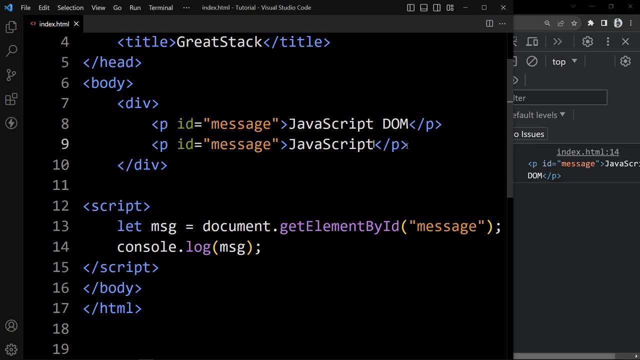 then it will return null. you can see null, and if there is multiple element with the same ID, it will return only first element. let's duplicate it and in this one we will only write javascript. now you can see the output in console. it is still printing ID message: javascript DOM. 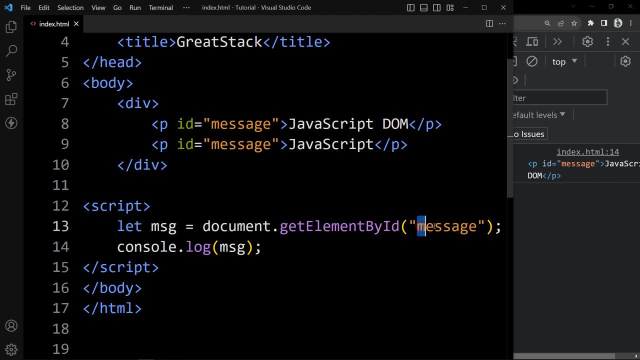 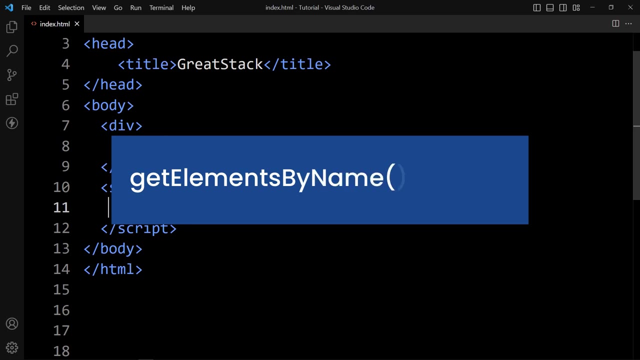 so it will select the first element with this message ID, because the ID of element is unique with the HTML document. the documentgetElementById is a quick way to access an element. now we will learn about getElementsByName method. every element on HTML document may have a name. 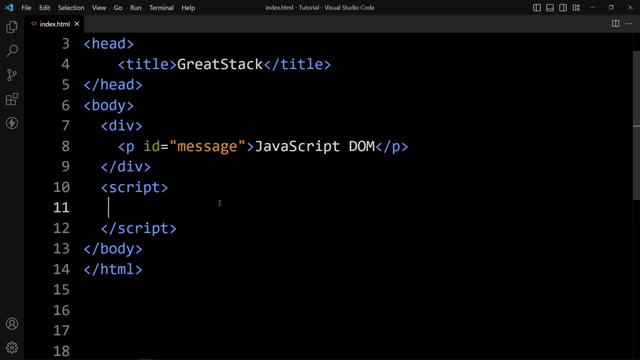 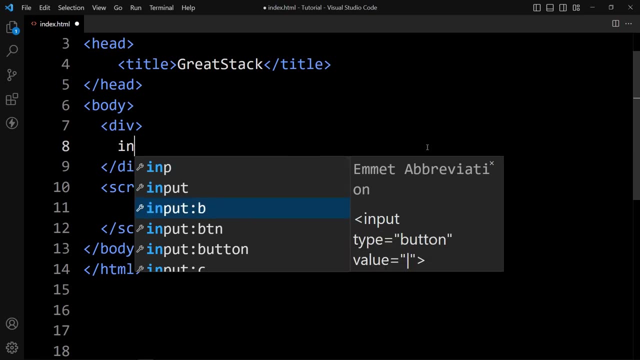 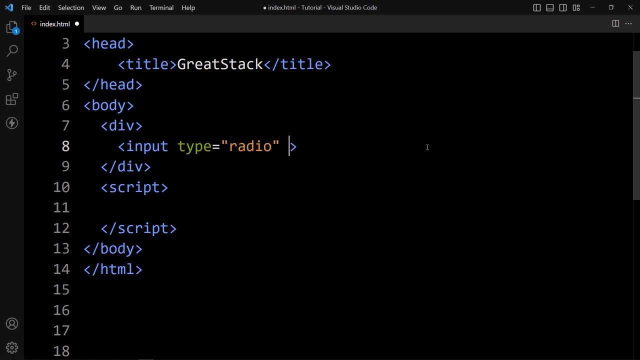 attribute. multiple HTML elements can share the same value of the name attribute. let's take one example here. we will create one input field and in this input field I will add the type radio and we will add one name attribute. name will be language and value will be JavaScript. we. 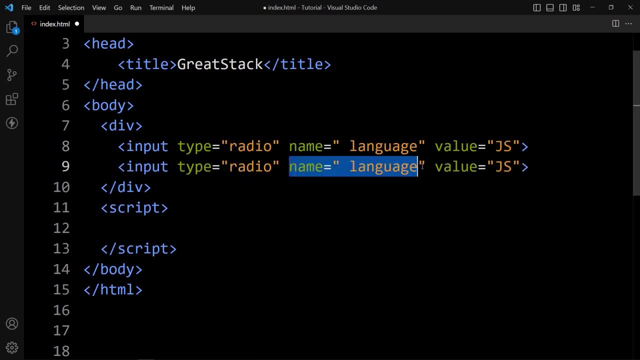 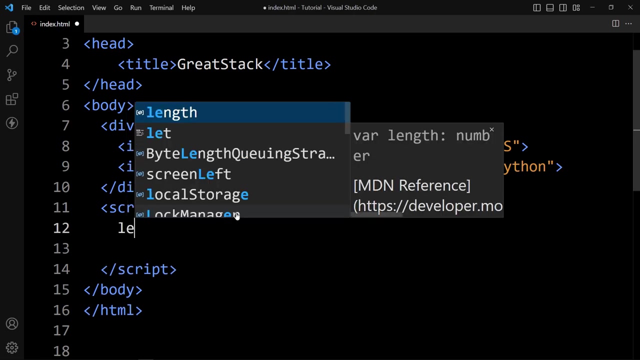 can add another input field with the same name attribute and value will be something else. Python in this HTML code. you can see we have two elements with the name attribute and we can select this element using this name. so in the subscript we will add: let btn is equal to documentgetElementsByName. 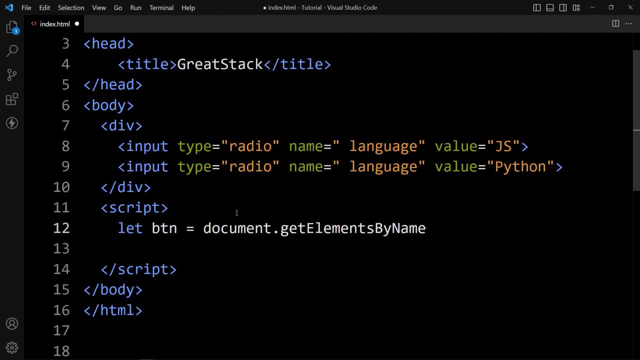 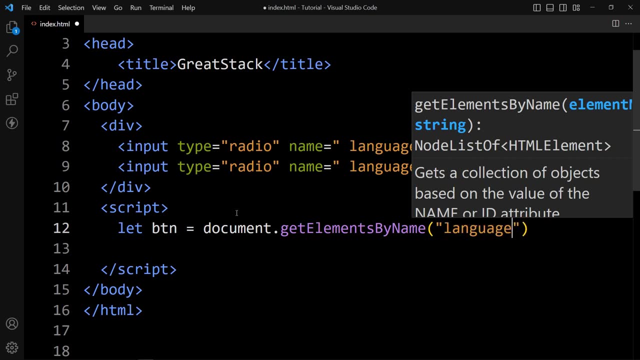 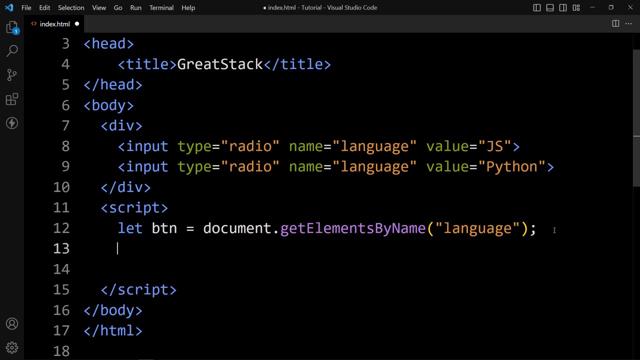 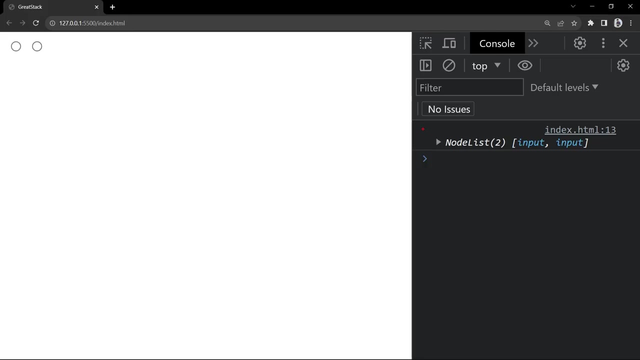 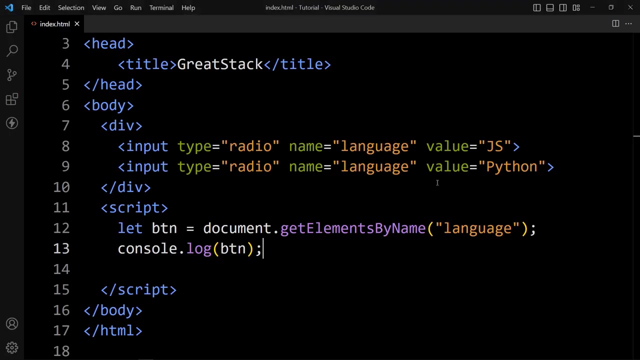 let btn is equal to documentgetElementsByName and in this one we will add language, because the name value is language. now we can print this: let us add consolelog btn and you can see the output in the console tab. here we have the node list that contains two input field. you can see input and input, so getElementsByName. 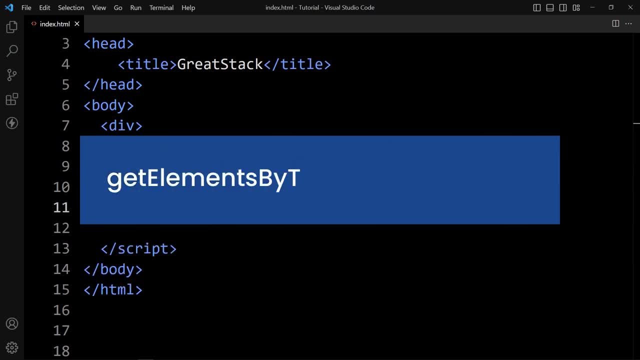 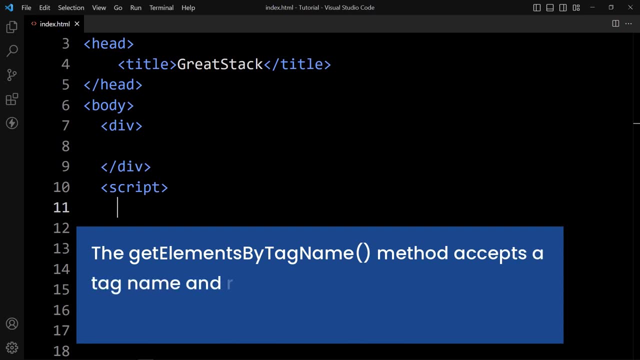 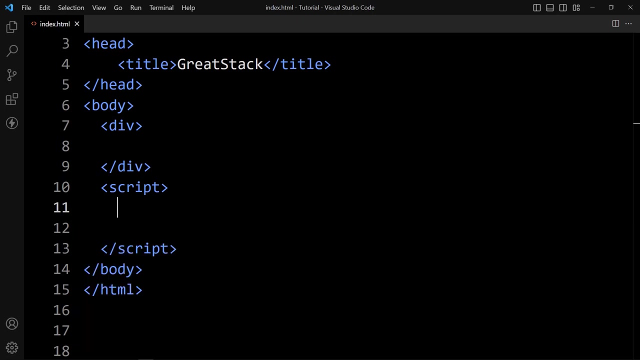 returns one list of nodes. now we will learn about getElementsByTagName. the getElementsByTagName method accepts a tag name and return a live HTML collection of elements. so let's understand it with one example. in this HTML, we will add one title in h1, so the text is first heading. let's duplicate it. this is second. this is third. 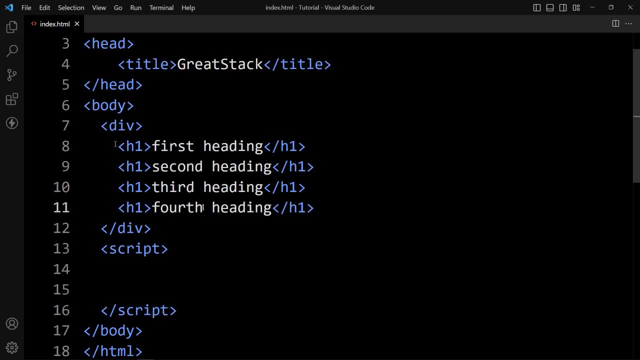 this is fourth. we have four text here in the heading tag. now we can select the element using the tag name, which is h1. so here in the subscript we will add one variable with the name. heading is equal to document dot. getElementsByTagName, and here we will add the tag name, which is: 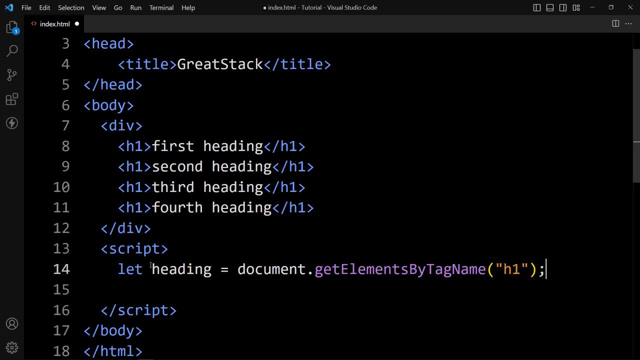 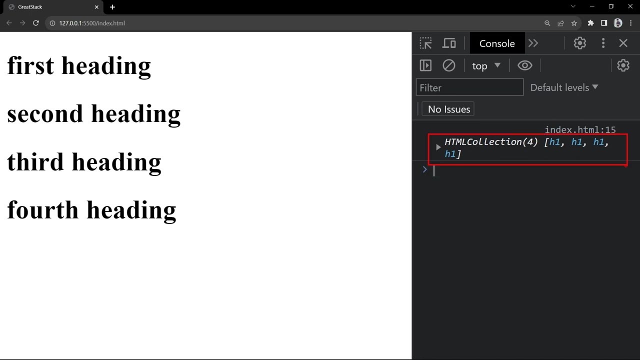 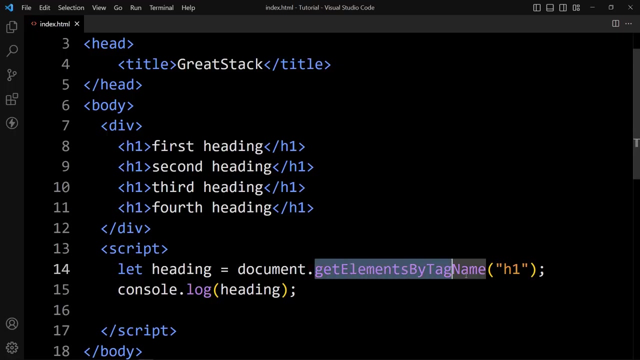 h1. now we will print it using console log heading so you can see the output on the console tab. it is returning the collection of four HTML elements. you can see h1, h1, h1 four times. so this getElementsByTagName return the collection of HTML elements. 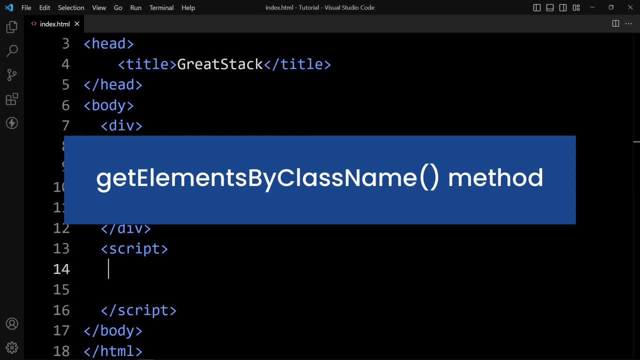 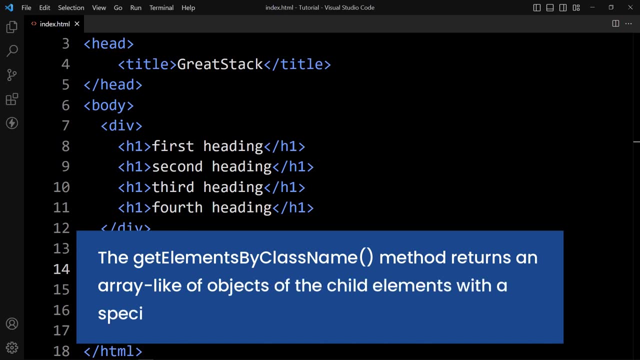 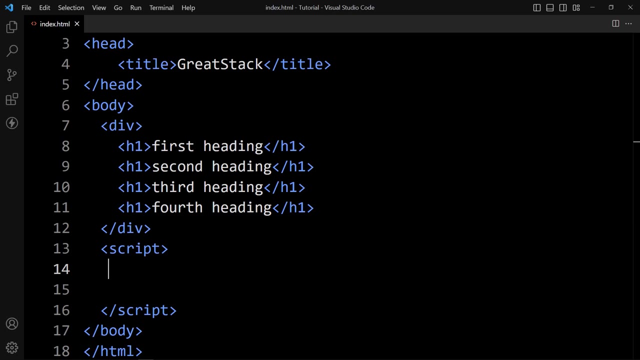 now we will learn about getElementsByClassName. the getElementsByClassName method returns an array, like of object, of the child elements with a specified class name. the getElementsByClassName method is available on the document element or any other element also, so let's understand it with one example here. we will add one class name in the first title, so the class name. 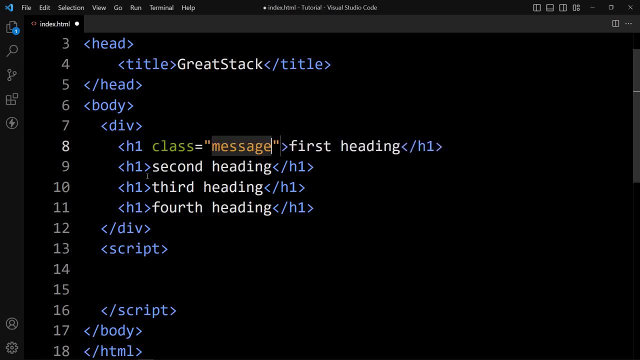 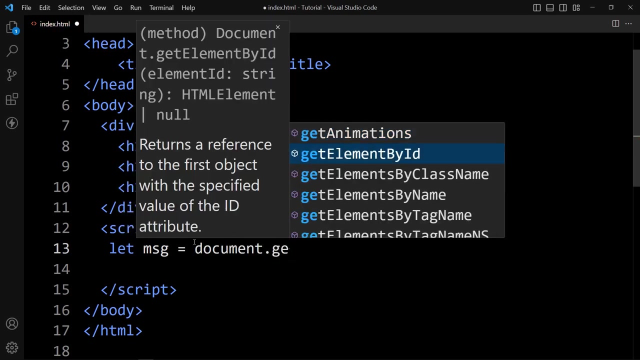 is message. in the second one we will add the class name message and in the third one also, we will add the same class name message. let's delete the fourth one. now we can select these elements with the class name in this script. let's add: let msg is equal to document dot getElementsByClassName. and here we will. 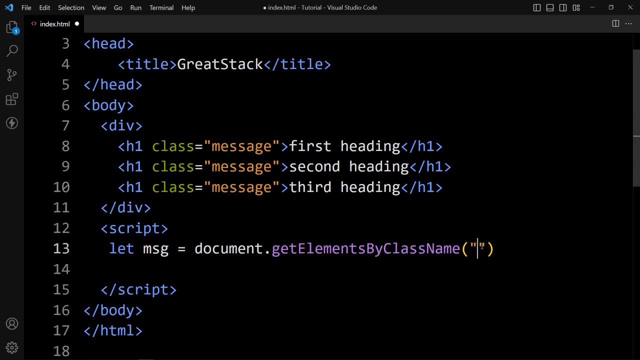 add that class name, which is message. now we will check the output in console. msg is equal to document dot. getElementsByClassName and here we will add that class name, which is msg, and you can see the output here. it is returning the collection of three html element. 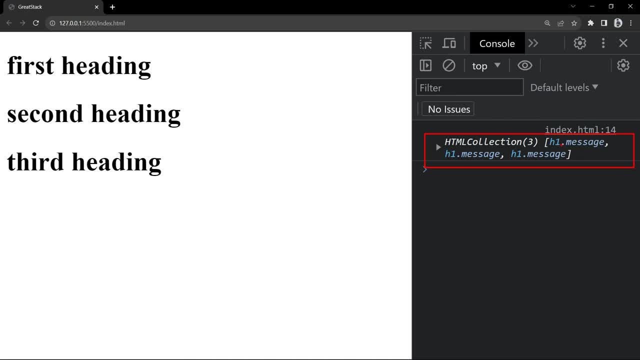 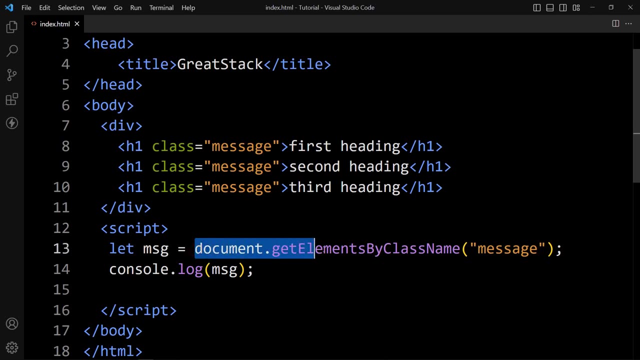 with the class name message. you can see h1 dot message. h1 dot message. h1 dot message. so it is returning all the html elements with the same class name. now let's come back to the code and here we have added document dot: getElementsByClassName. we can add this: getElementsByClassName. 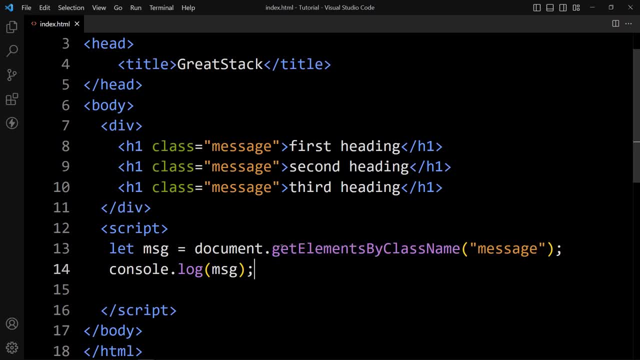 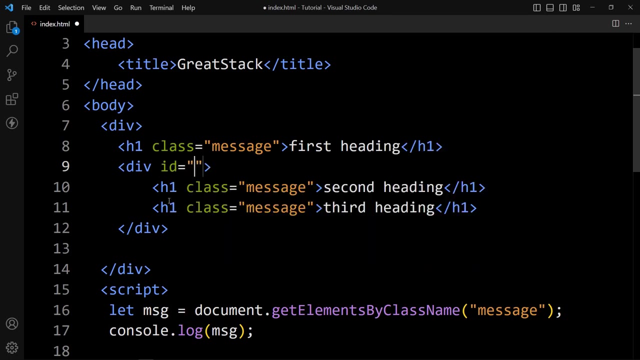 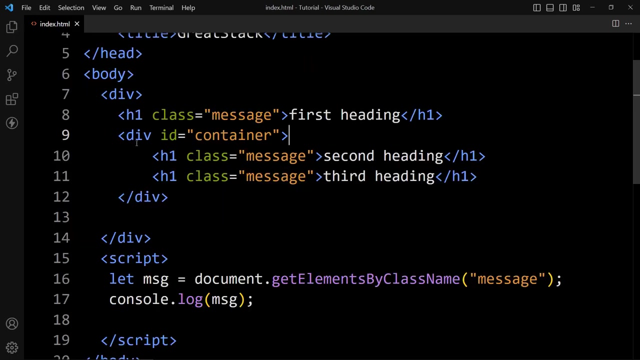 with the same class name on any element also. so let's see the example here. I will add one div and insert these two title in this div. and for this div we will add one id. let's add the id container. so, total, we have three headings with the class name message. but these: 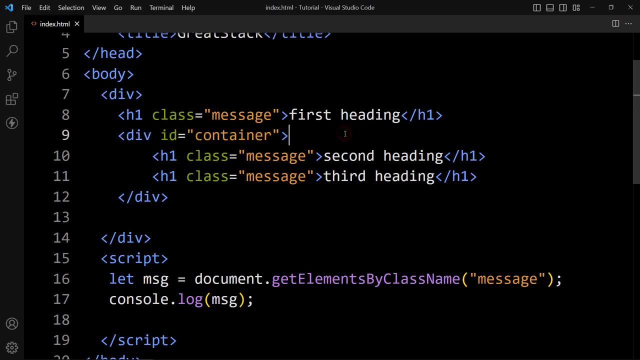 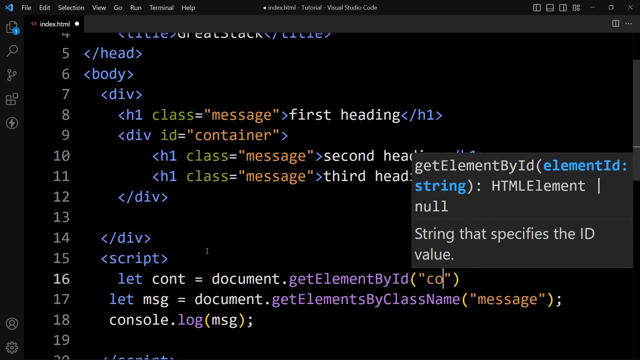 two headings are included in this div with the id container. now we will add the get elements by class name over this container. so we have to store this container in one variable. so let's add: let cont is equal to document dot. get element by id and the id is container. 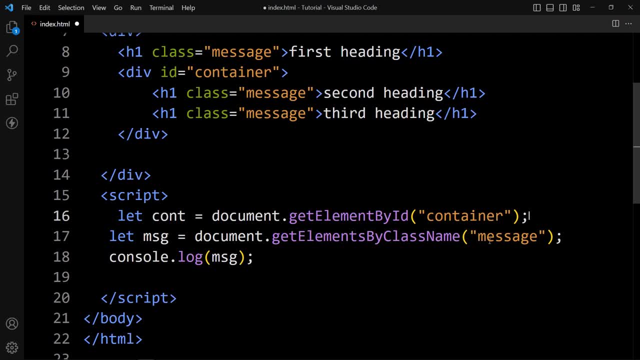 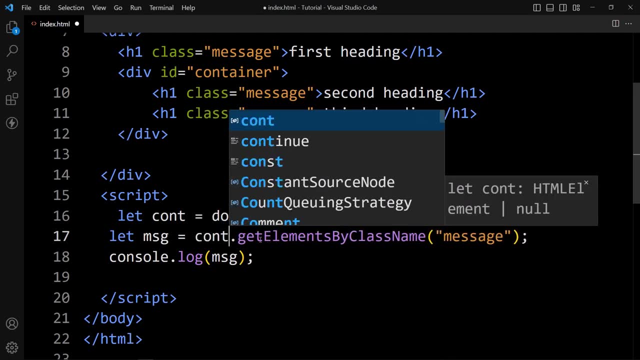 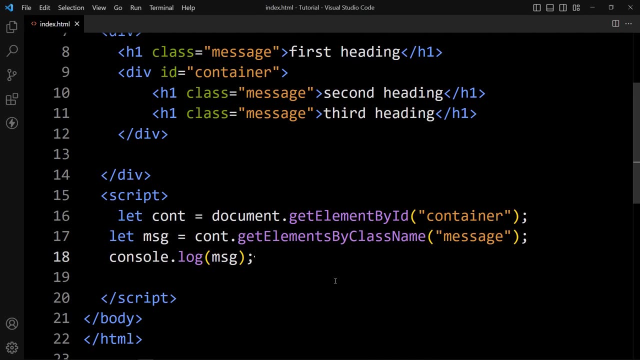 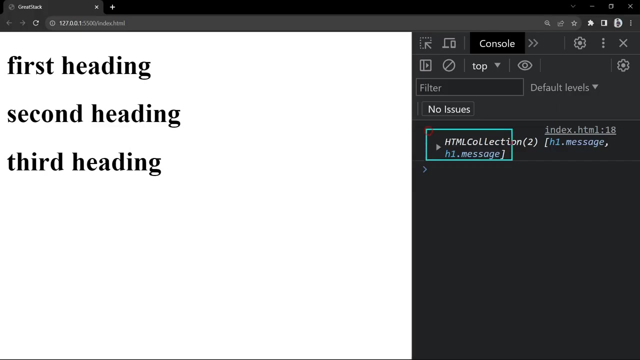 now we can write cont here in sheet of document. we will add cont, which is container, and get elements by class name. now it will only give the elements within this container. you can see the output here. we have only two elements. this is html collection 2. we have two html elements in this collection. you can see that we have only one element here. we have only one element here: edible AwayFresh and Sarla Neylont and Aslysh common. here's the output of these two elements. we cannot add additional elements to get basicize the HTML block, just the other elements. 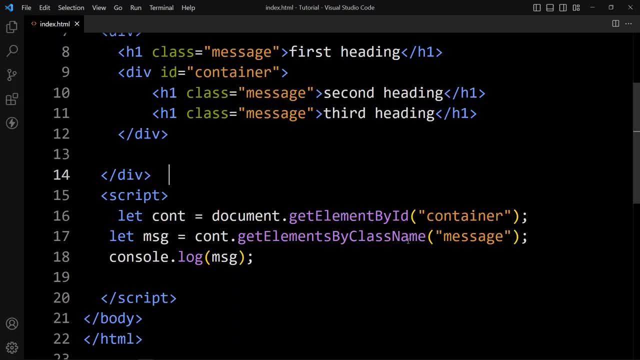 and we have only one element here and we have here. we have two elements to get complex and h1.message. h1.message. so this get elements by class name will return the collection of html elements with the same class name on the document or within the element. now let's learn. 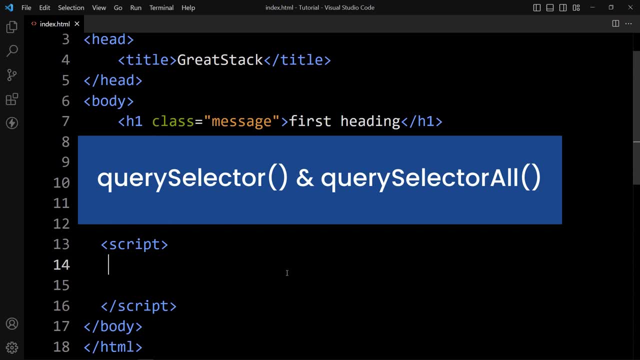 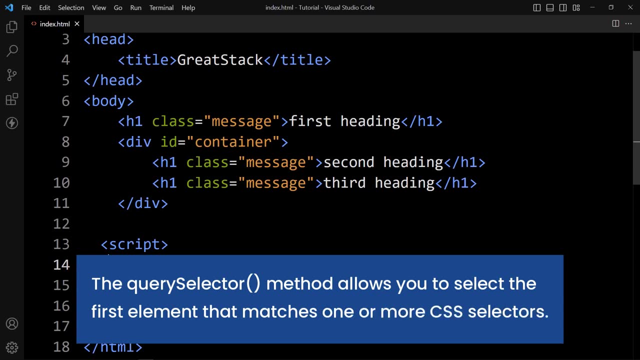 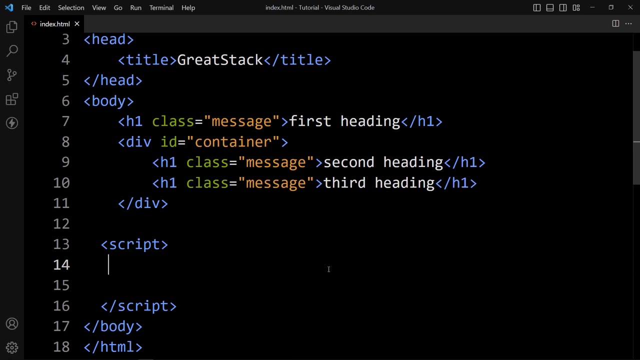 about query selector and query selector all method. the query selector method allow you to select the first element that matches one or more css selector. the query selector is a method of element interface. we can apply this on element also. here we will add one variable. let msg is: 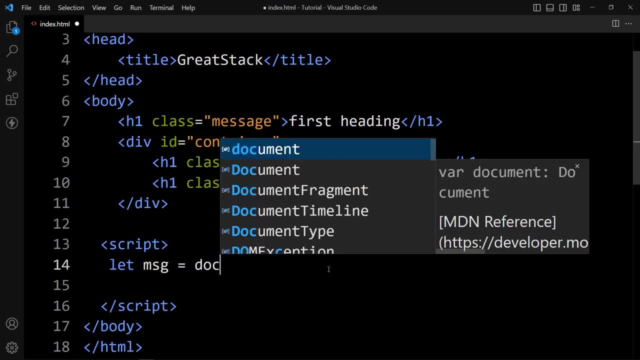 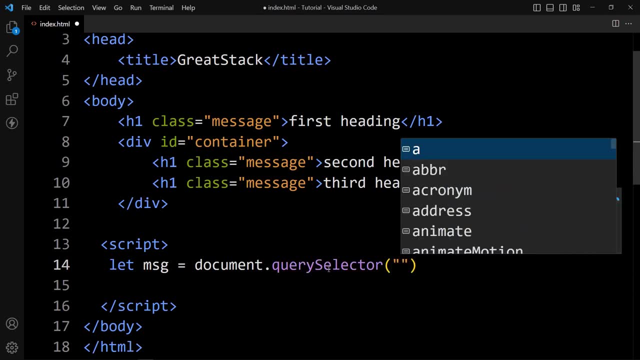 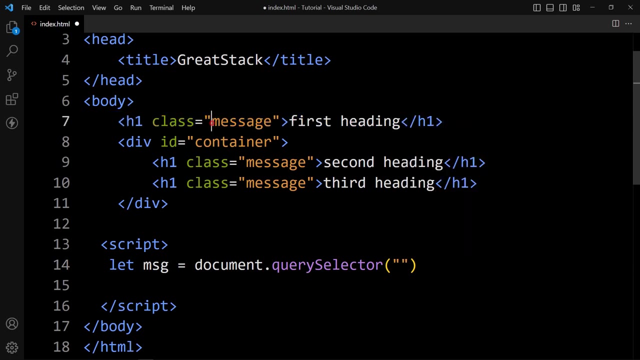 equal to document dot query selector and in this query selector we have to add the css selector. so in css to select this title we used to write dot message because it's a class name. so we used to write dot message to select the dot message. so we can write dot message to select the dot message. 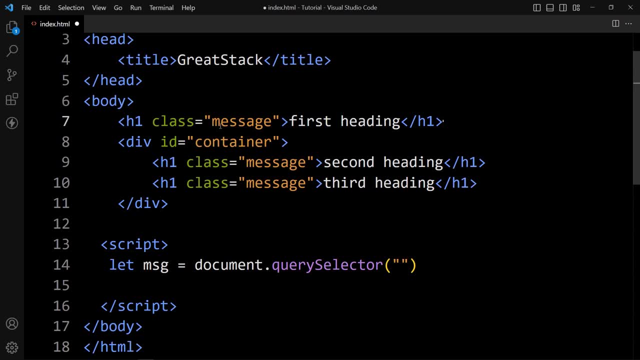 select this element in the css file. so we have to add the same thing here. we have to add the css selector in this query selector. that's it. so here we will print console dot log msg. so first let's see the html code. here we have one title with this message another. 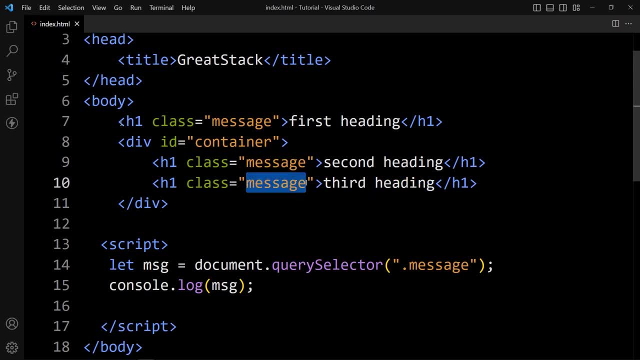 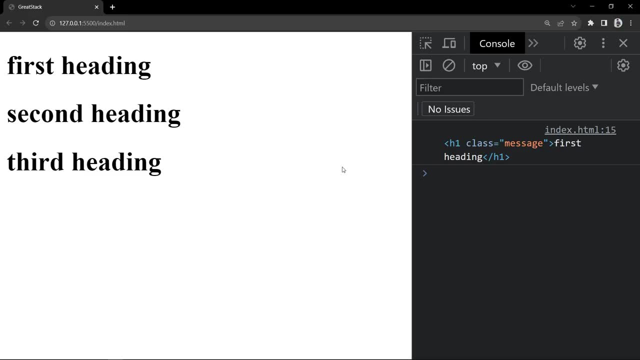 title with this message and third title with this message. so total: we have three title with this message: class name. now let's see the output in console tab. here it is displaying only first element, h1, class name message, first heading. so let's come back here. you can see. 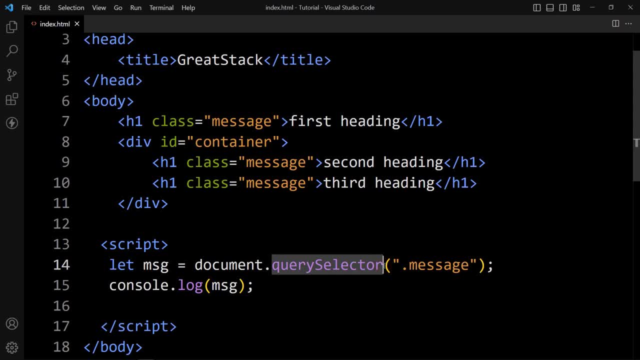 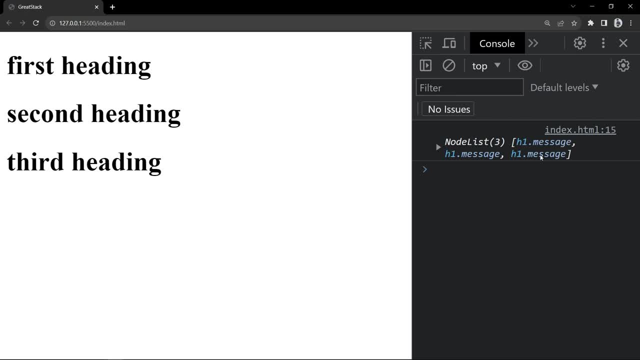 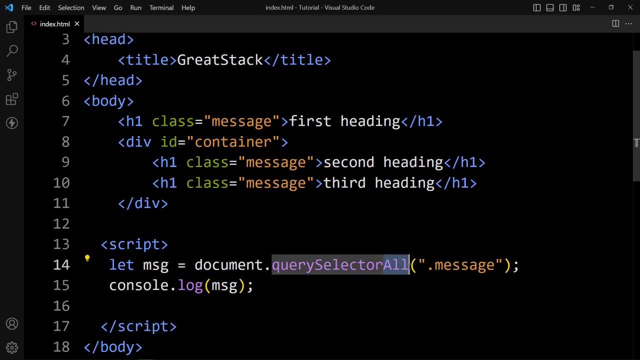 here we have added query selector all on document. we can use the query selector all on any element also. so let's addemberg, for container is equal to document, dot. get element by id. here we will add this id container. now we will add this query selector over this container, so just add. 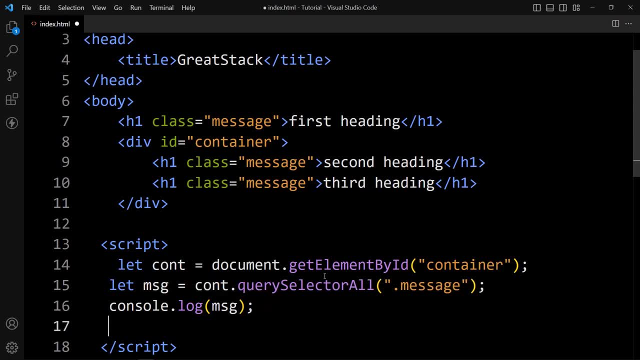 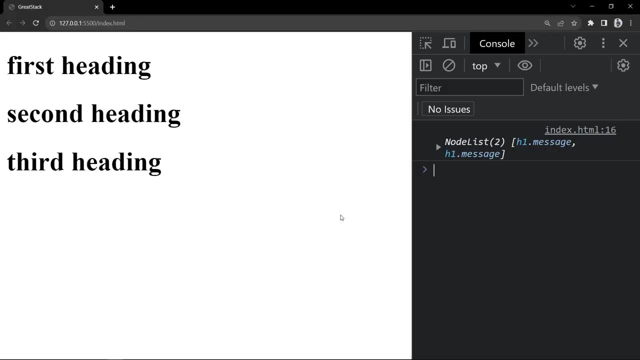 container dot query selector. so it will give only two elements, which is here second heading and third heading. now you can see the output in console tab. it is displaying node list 2. it is displaying two element. so it is selecting only two elements, which is in the container with the class name message. now let's come back to the previous example. 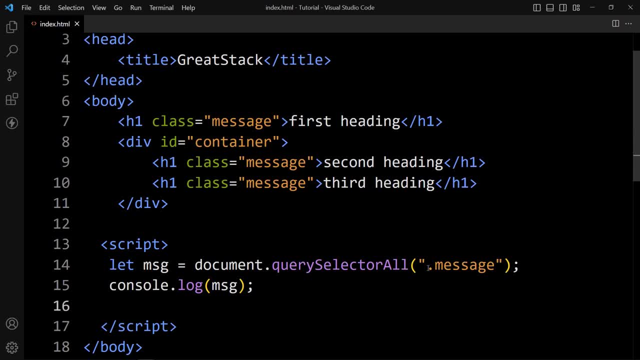 document: dot query selector. all now let's see what we can add in this query selector. so we can add the class name using dot, so we can add the id. also we will add the id and we can write this container. we will add hashtag and this container because we used to write like this for css: selector, hashtag container. because here we 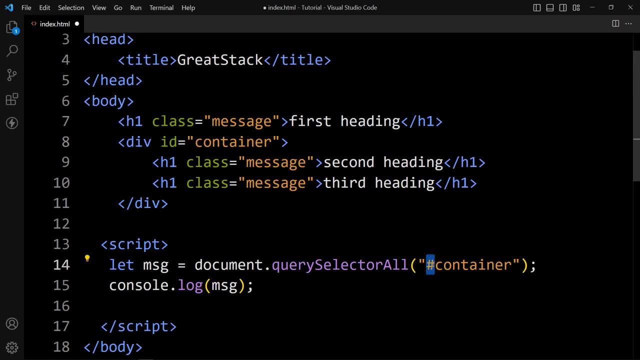 have the id container so we can add the hashtag to select the element with the id. now we can add like this directly: div, so it will select this div element. if we just write h1, so it will select the heading element with h1 tag, we can write like this also: div and h1 so it will select the 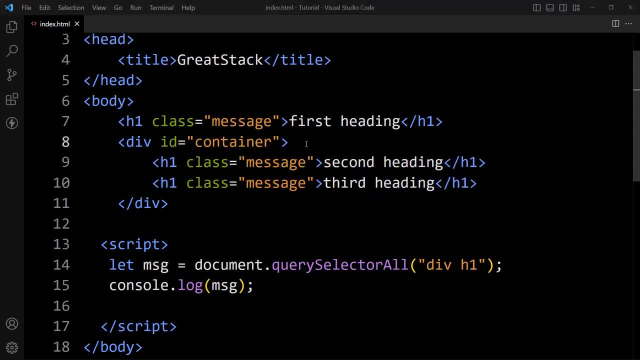 heading within this div. you can see the output here. we have 2 h1 only now come back and we can select the multiple element, like this div also and h1 also. so it will select all the div element and all the h1 element by adding h1 and h2. so it will select all the div element and all the h1 element. 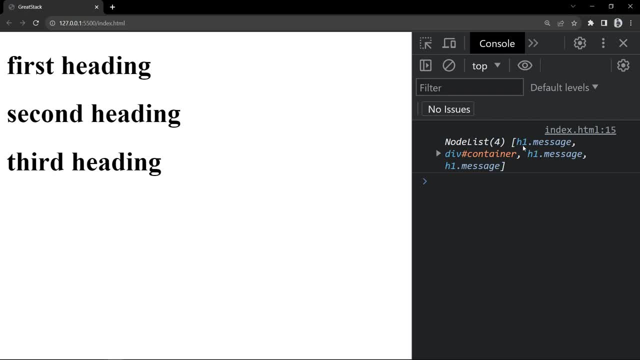 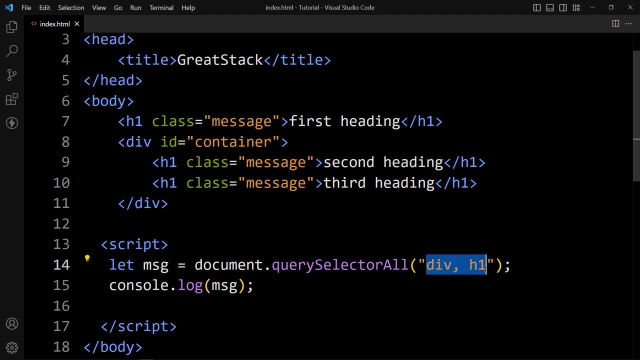 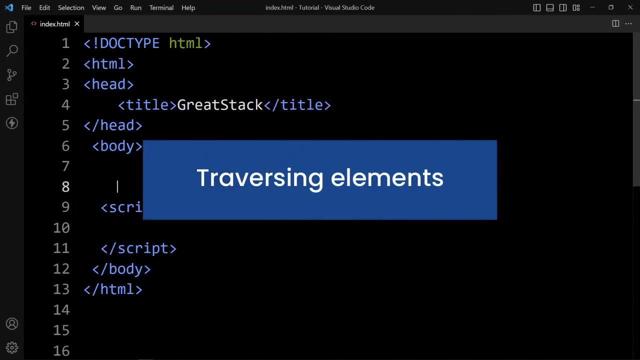 adding one comma. you can see here we have four element node list. four: one is div with the container id and three h1 tag with the class name message. so basically we can add all the css selector in this query selector and query selector all method. now we will learn about traversing. 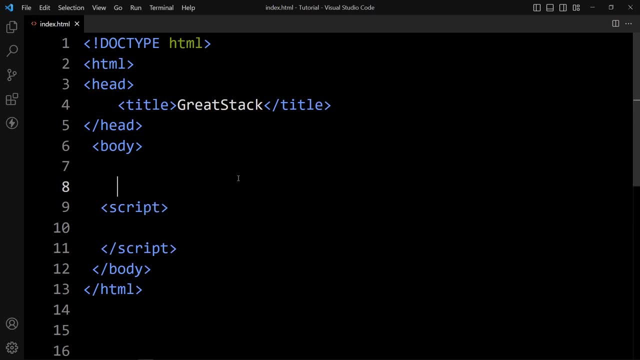 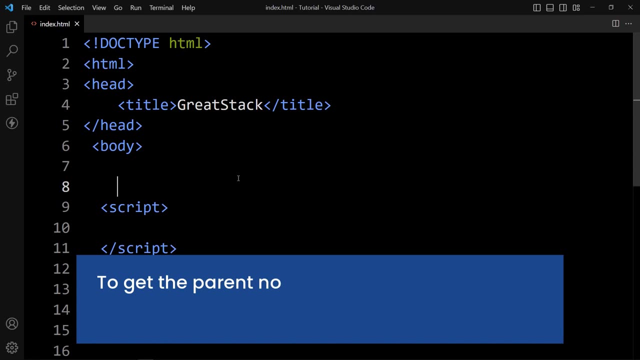 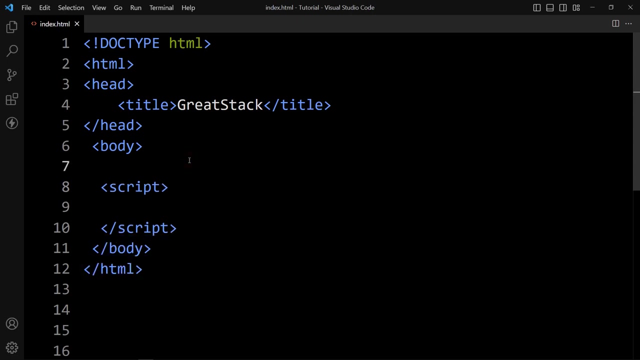 elements. to understand how to get the parent element, how to get child elements and how to get the siblings of an element. to get the parent node of the specified node in the dom tree, we can use the parent node property in this body. let's create some html elements we will add. 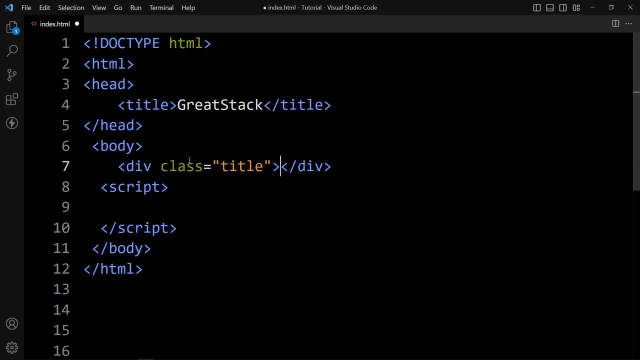 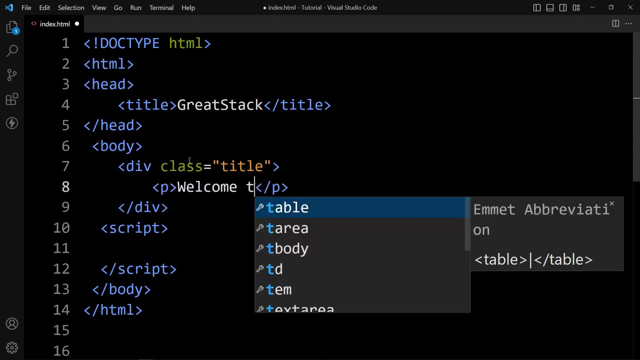 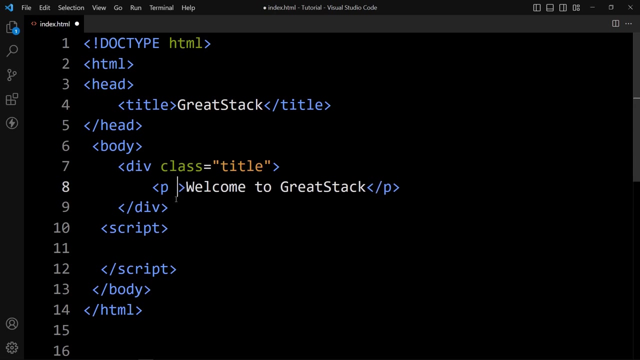 one div with the id title and within this div we'll add one text in p tag- welcome to great stack. and for this p let's add one class name text. so we have one parent element and one child element. now we will try to get the parent element using this child element. so here in this script we will 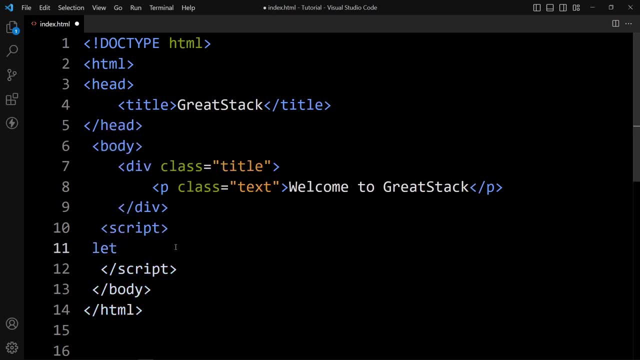 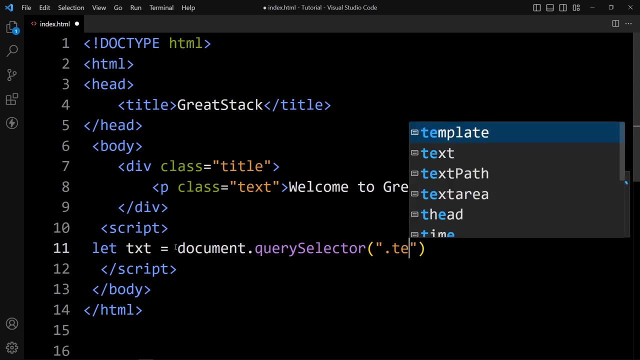 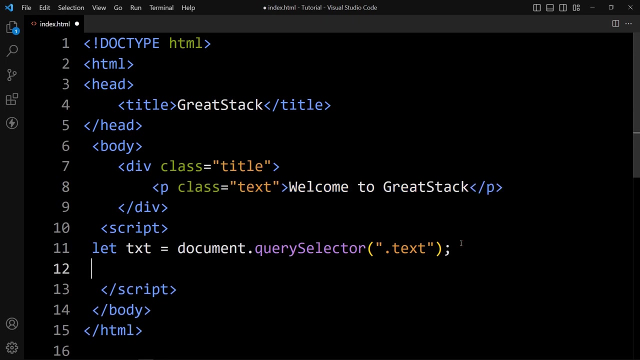 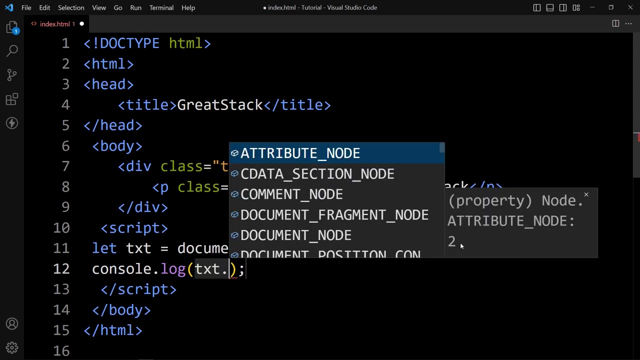 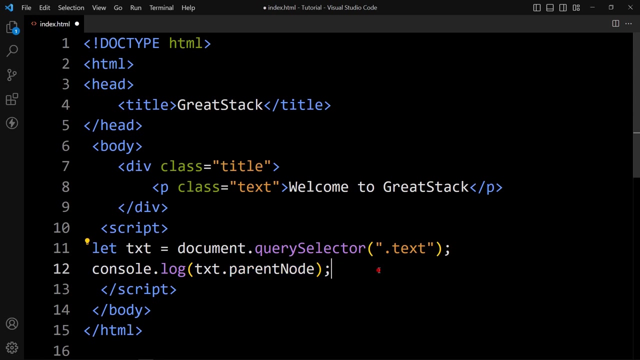 add let. txt is equal to document dot query selector and we will add dot t text so it will select this p element. now we have to get the parent, so we will add consolelog, then txt, which is the child element: dot parent node- this one. just add this parent node and it will display the parent element of this child. 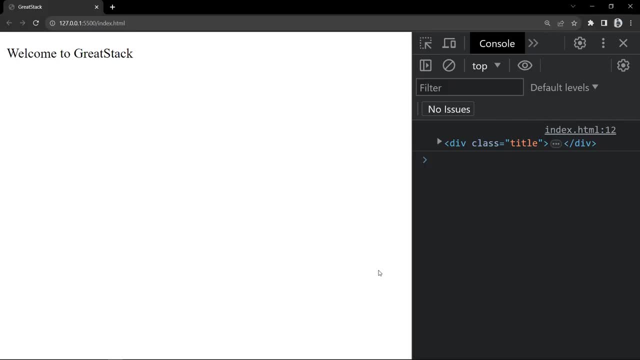 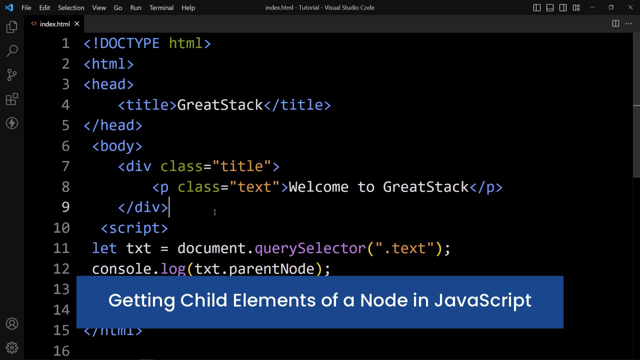 element. so now let's see the output in the console tab. here you can see it is displaying div class title, which is the parent element. now let's learn how to get the child elements. we will learn about how to get the first child element, last child element and all children of the specified element. 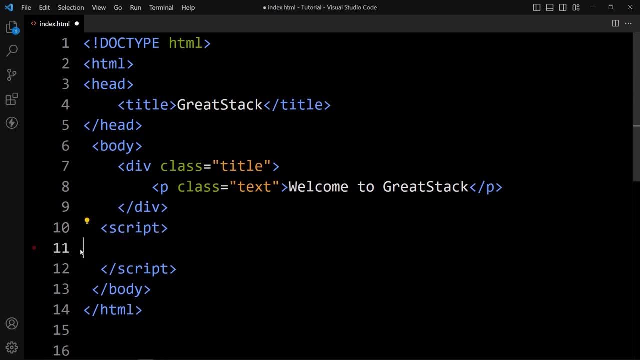 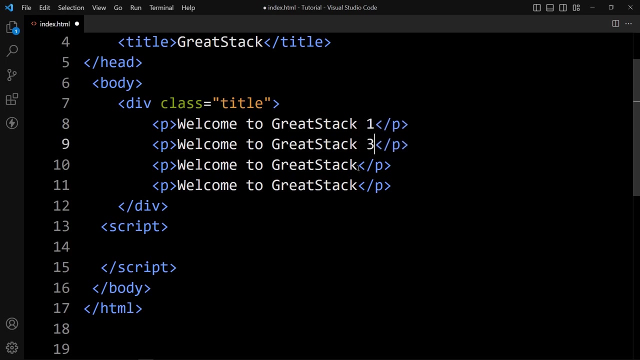 so here we will add another example. just remove it and within this let's create multiple p tag. we have four text here: greater stack one, two, three and four. so we have four title. welcome to greater stack one, two, three, four. so now we'll get the child element using this parent element now within this script. first we'll 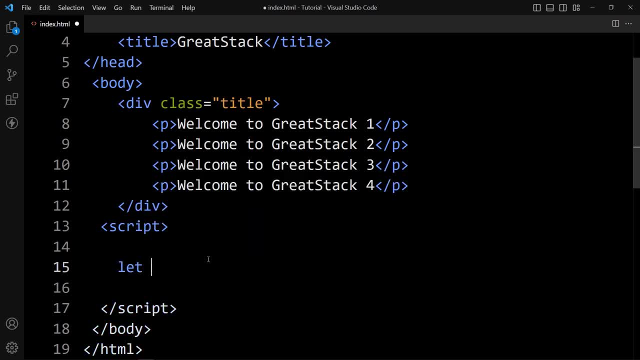 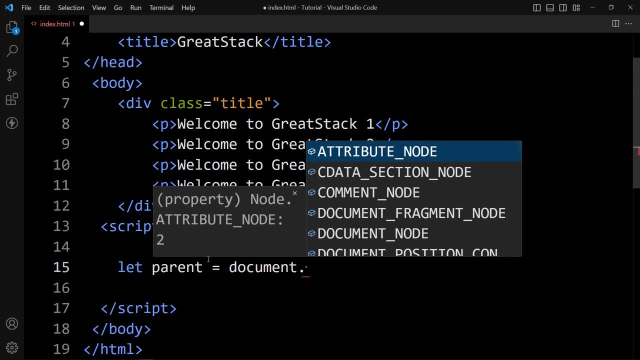 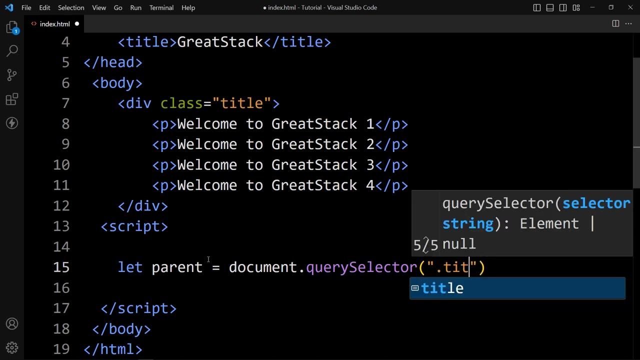 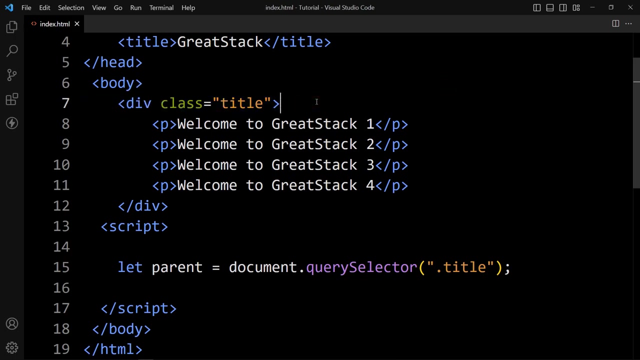 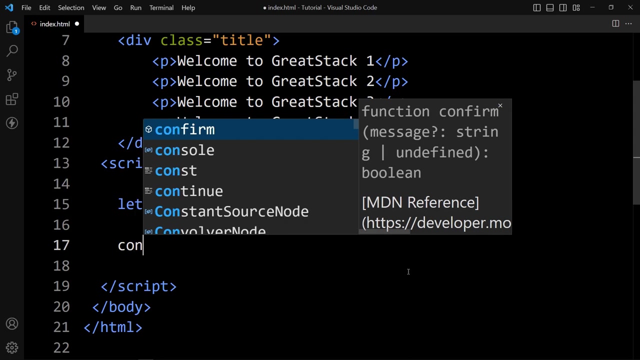 select this parent element. so let parent is equal to document dot query selector and write the query selector title. so it will select the div. now we have to get the first child, last child and all the children of this div. so here we will add console dot log and this parent. 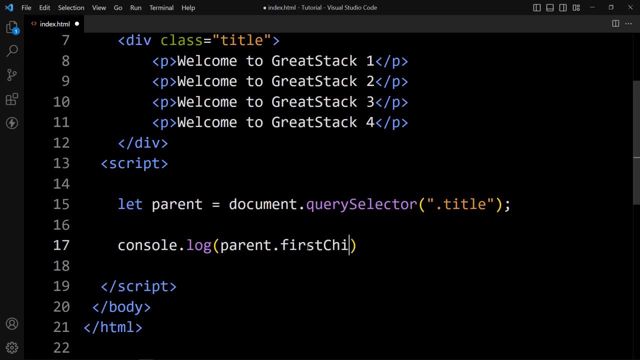 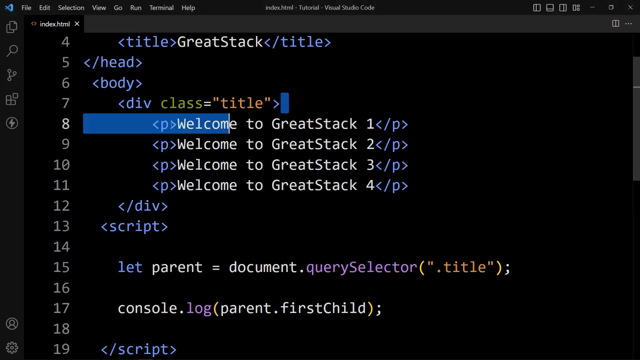 then we will add first child. now you can see the output in console tab. here it is displaying hashtag text because here we have some space. so this space is also one of the great elements we just created. actually we can see. I will do a whole section and see that. 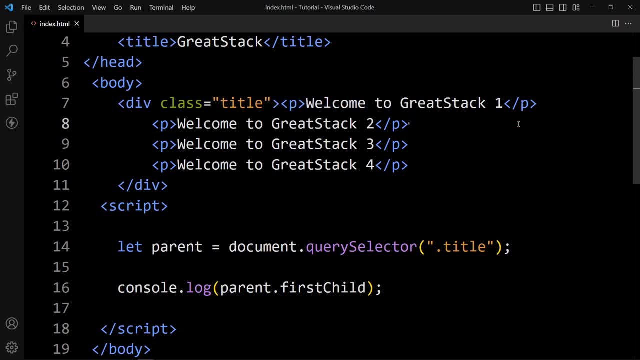 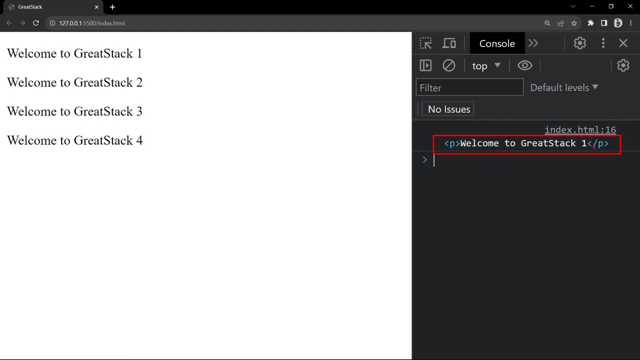 we've only got one empty text node. if we remove this and write it in the same line. now you can see the output in console tab. it is displaying the first title, which is welcome to greater stack 1, and if I add a space here it will display: 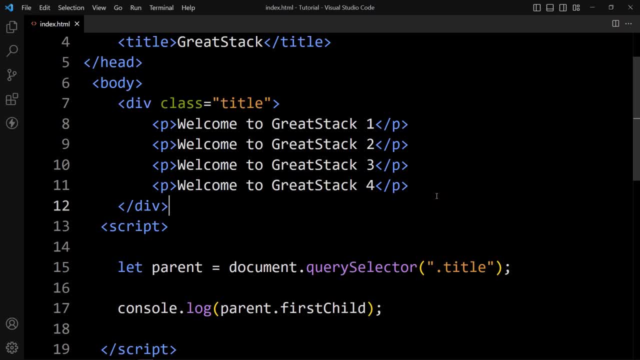 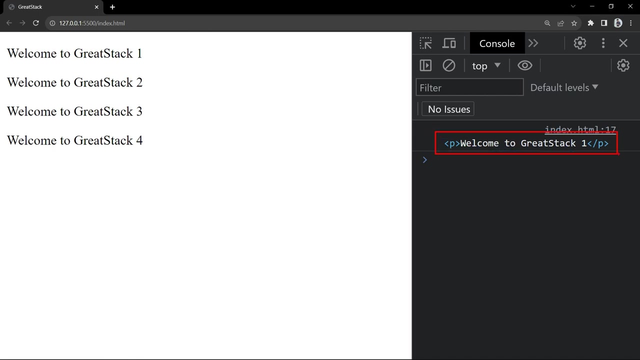 one text node. now I want my text like this and I want to display the first element. so here we will just add firstElementChild like this: parentfirstElementChild. now you can see the output. it will display the first element. welcome to greatest tag one, the first title in p tag. similarly we 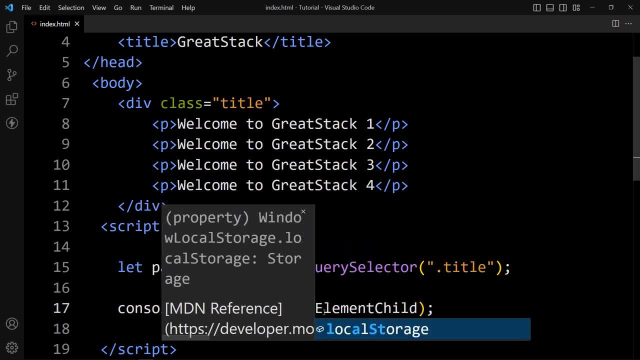 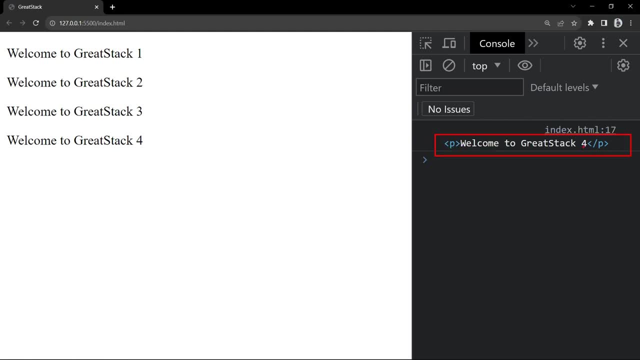 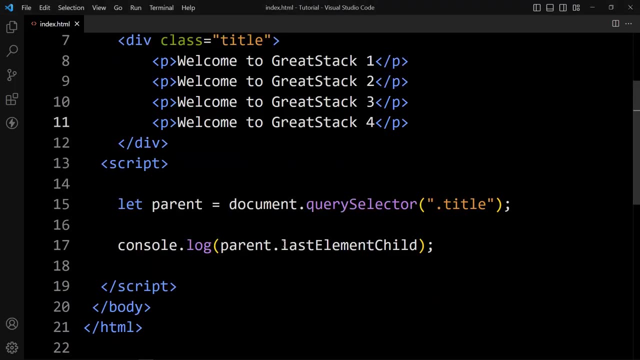 can add lastElementChild like this and see the output. it is displaying welcome to greatest tag four. right, so it is giving the lastElement, which is welcome to greatest tag four. now, if you want to get all the child elements, just add child nodes. that's it. after adding: 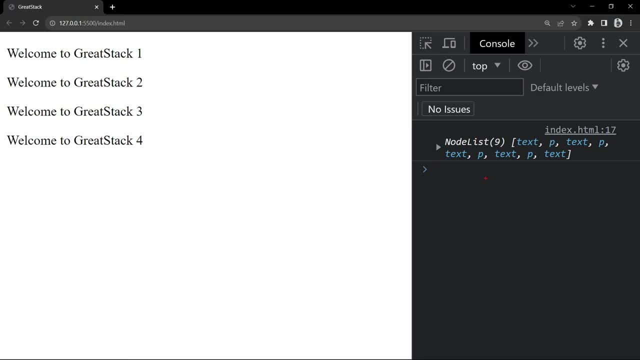 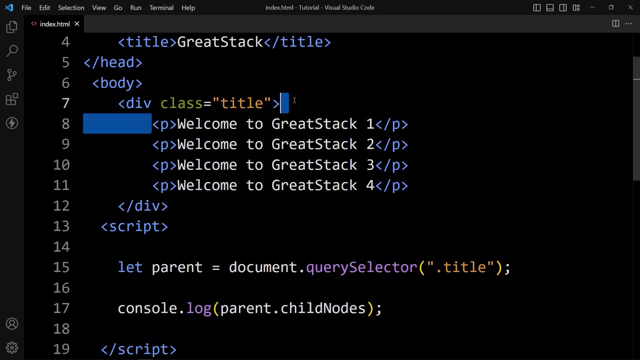 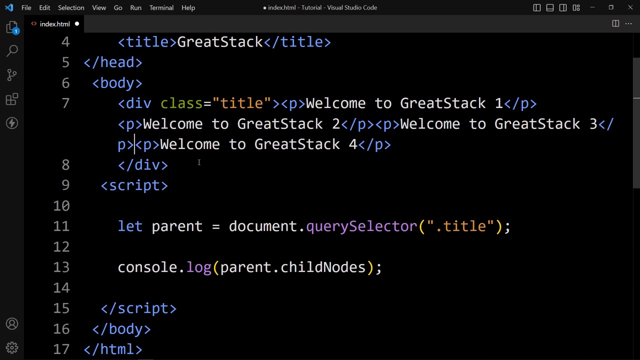 this. come back to the web page and here you can see we have node list text, again p, again one text, again p. so we have the empty text node, then p tag. let's come back and let's add child nodes. and here, if i remove this space and write everything in the same line, 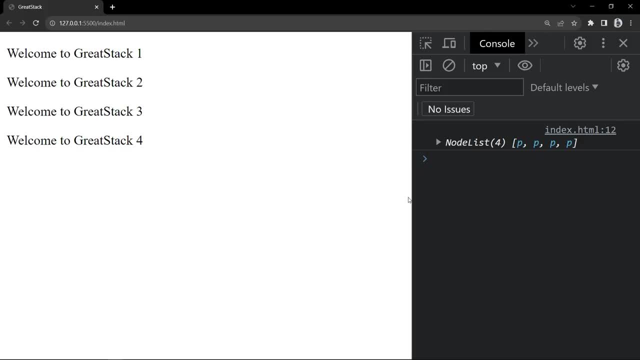 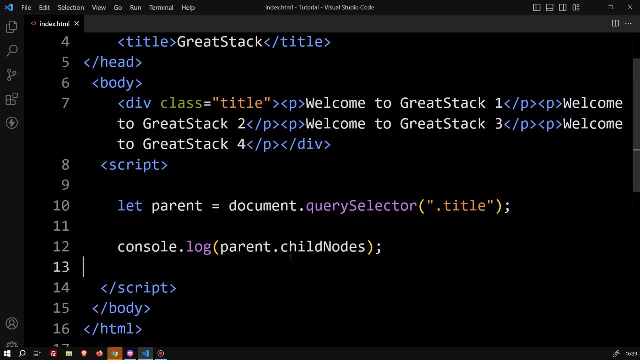 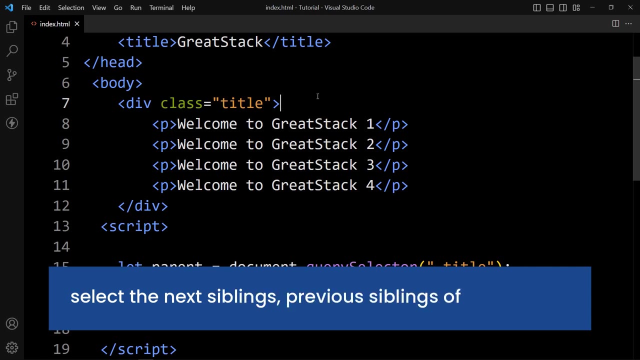 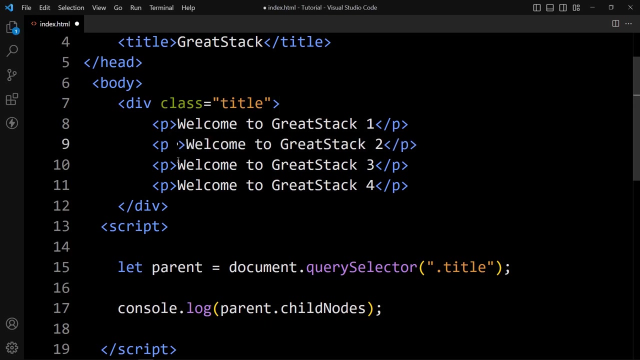 like this. now you can see, it will only display four element, which is four p element. so we got the child nodes of this div. now we will learn about how to select the next sibling and previous siblings of an element. so in this example, in this second p tag, we will add one class name. let's add class name. 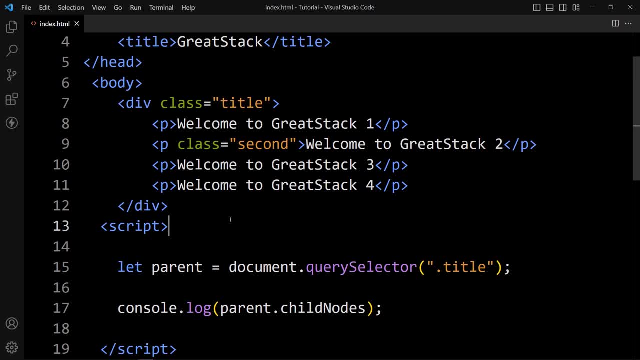 second like this. so it's easy to select this element and according to this element we will find the previous siblings and next siblings. so here we will add cut echo second. here also second. so it will select this: welcome to greatest tag two. now to get the previous sibling, here we will add this element, then dot and write previous. 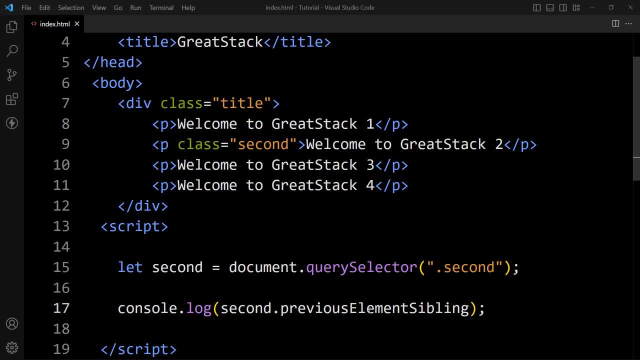 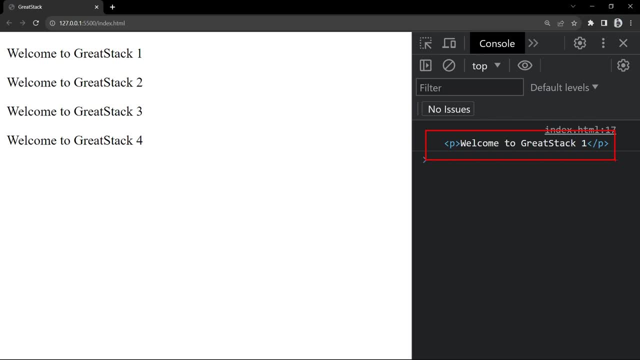 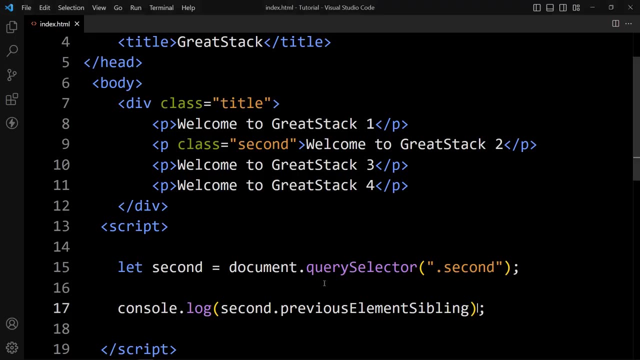 element sibling. that's it. you can see the output. it is displaying Welcome to GreatestTag4.. greater stack one. So we are finding the previous sibling of welcome to greater stack two. Now just come back and here we will add next. So it should give this: welcome to greater. 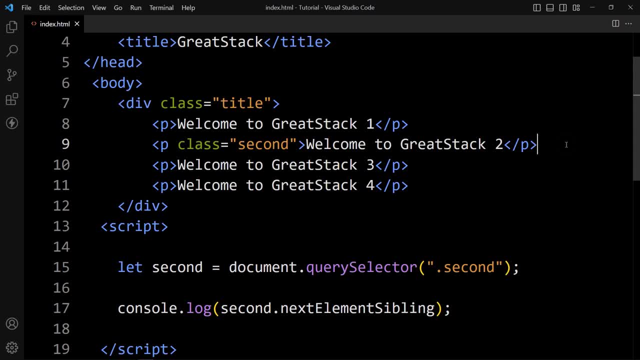 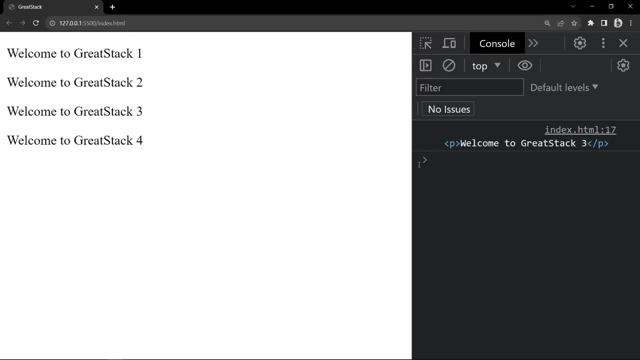 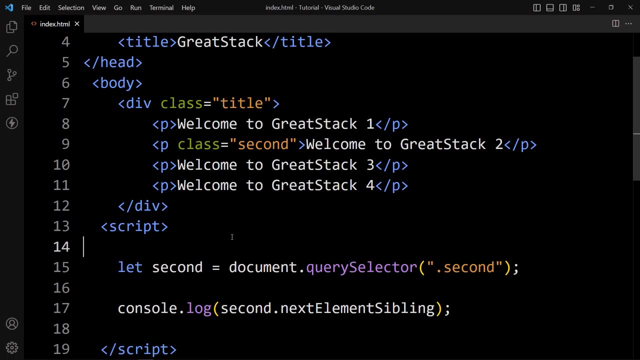 stack three, because we are selecting this second one and we are adding next siblings, So it will display third. Now let's see the output Here. it is displaying welcome to greater stack three. So this is how you can select the previous siblings and next siblings. 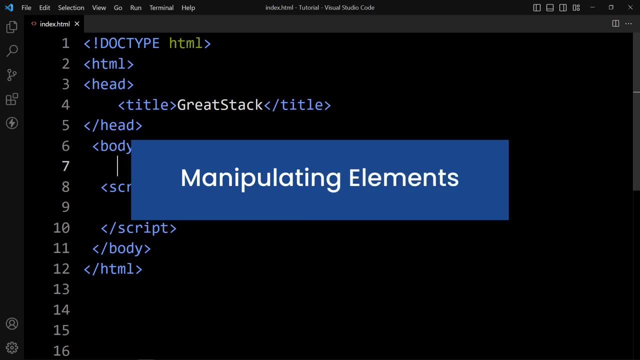 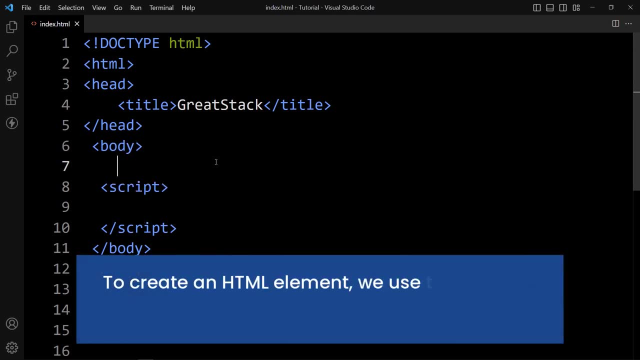 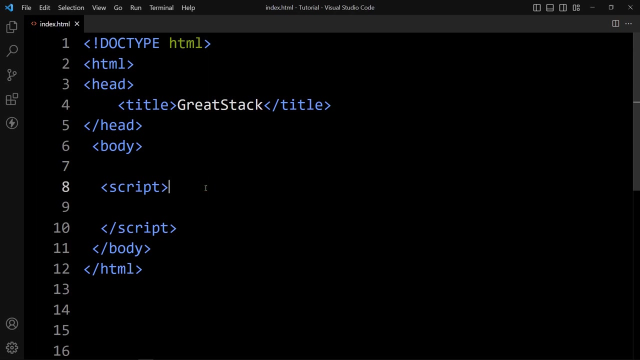 Now let's learn how to manipulate the HTML elements. So the first one we will learn is create element. To create an HTML element, we use the create element method, The documentcreate element accept an HTML tag name And return a new node with the element type. So let's understand it with one example Here. 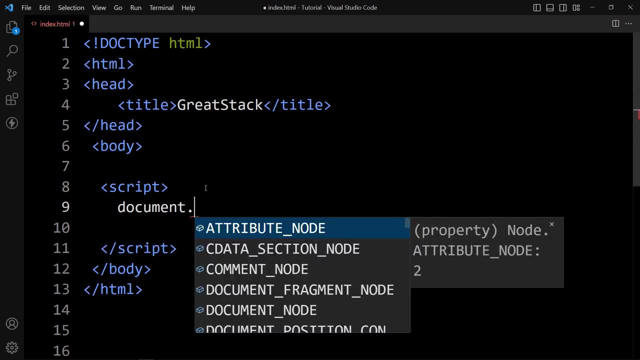 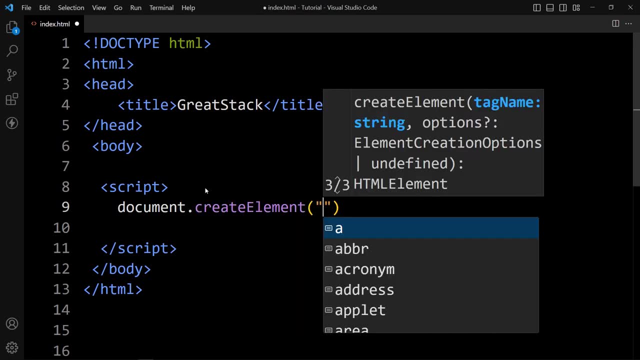 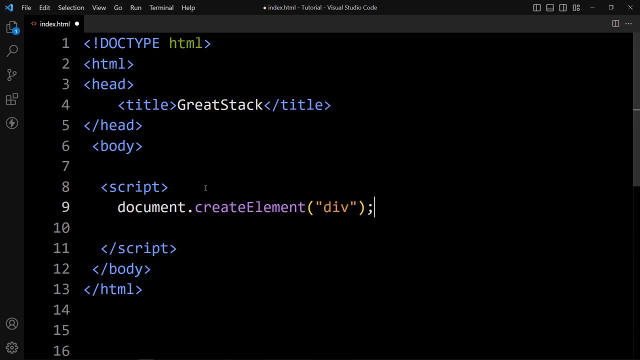 we can add document dot create element, And in this one we have to add one HTML tag. So let's add the div tag, So it will create one div element. We can store it in any variable, So we'll add div dot set. div is equal to document dot create element div, So it will create one div element. 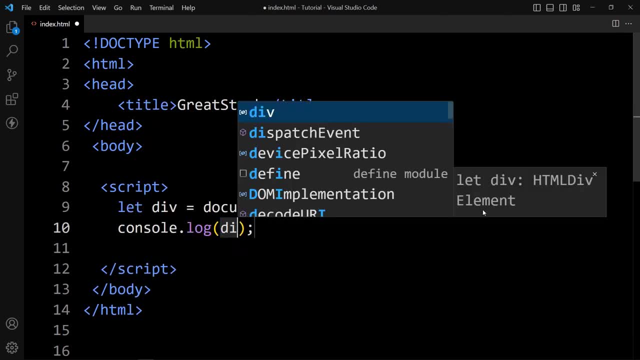 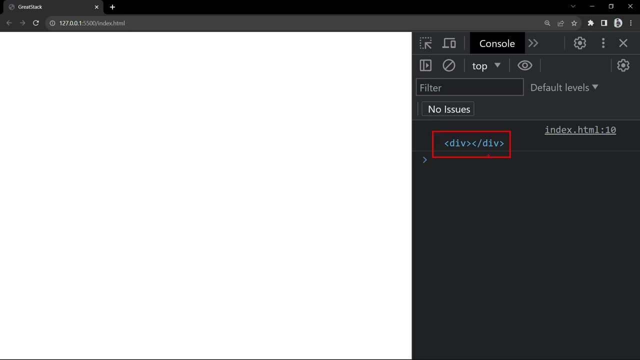 Now we can print it. Let's add console dot log div. You can see the output on the web page. It is displaying this div. This div is empty right now, So let's come back here. In the next line will add: 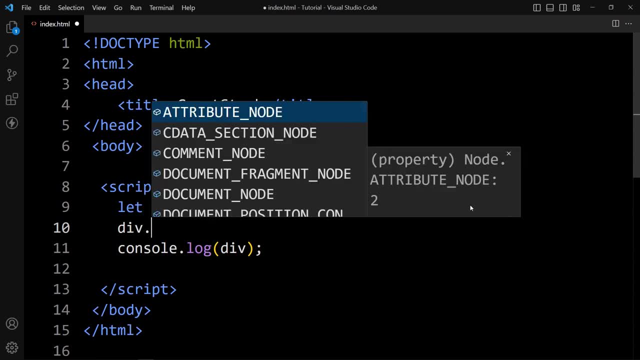 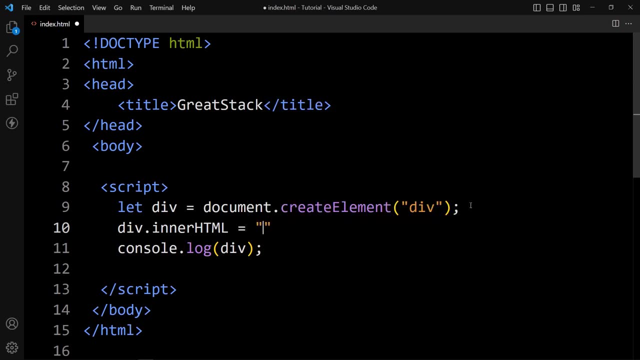 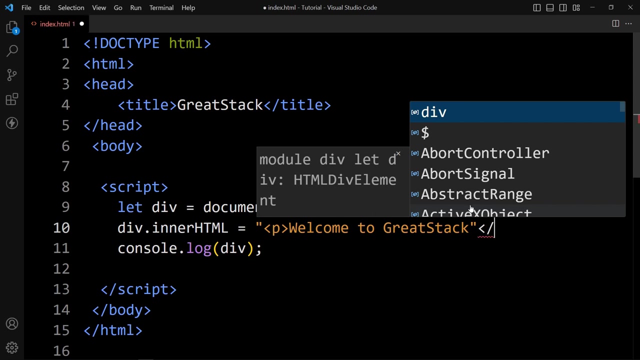 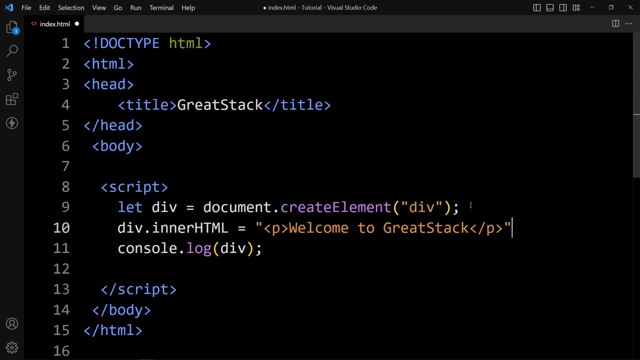 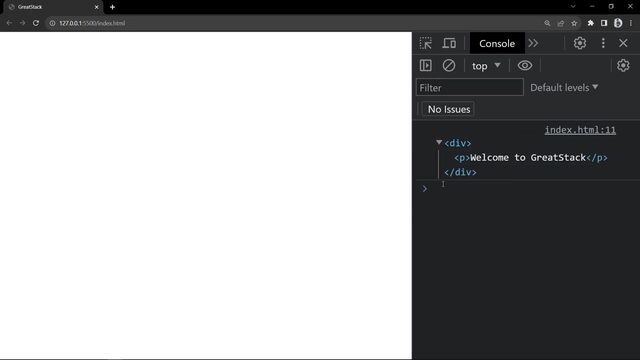 Div, div, dot, div, dot, innerHtml. we will learn innerHtml also. so here we can write any html code. we will add one p tag and in this p we will add welcome to great stack and close this p. Now we will see the output. here you can see one div and here we have one text in this. 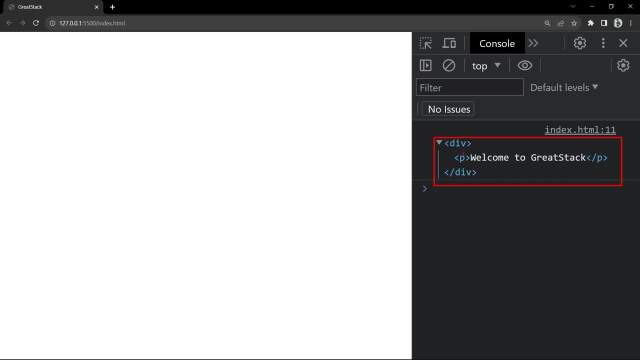 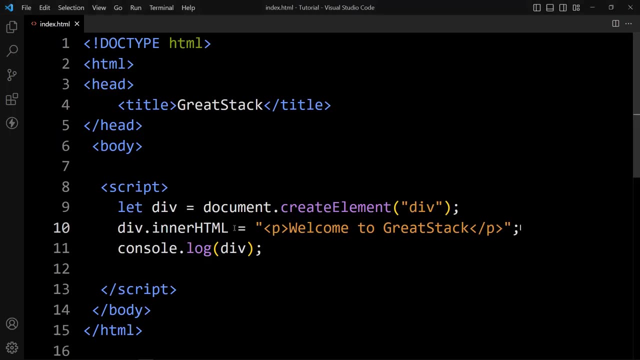 p, we have one div tag and within this div we have p tag and the text is welcome to great stack. So you can see, using this documentcreate element, we can create one div element or any html element and we can add any html code within this element and we can print it and 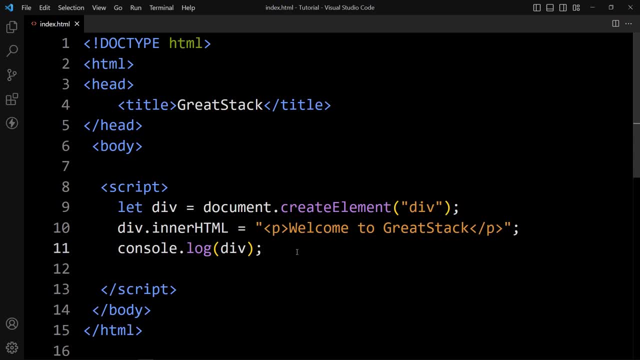 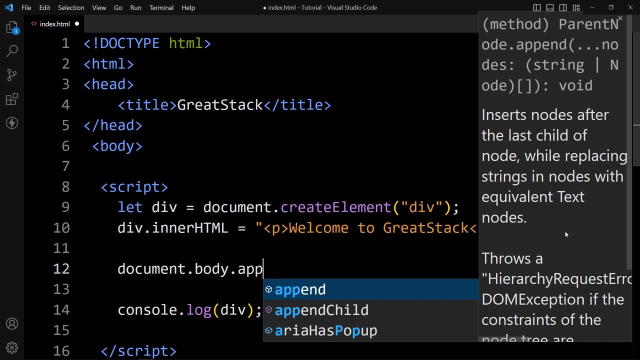 we can also add this element on our web page. So to add this element on our web page. here let's add documentbody. we will add this element on the body. so here we will add bodyappendchild. we will learn the appendchild later, so to insert: 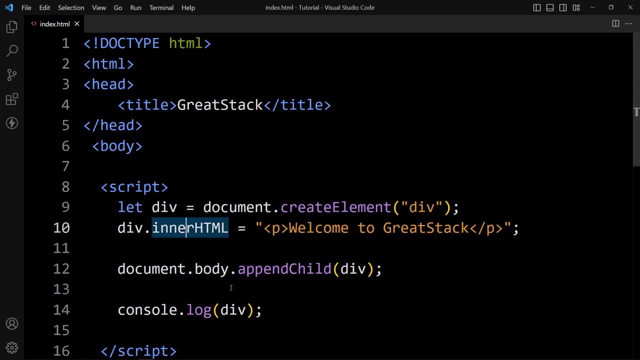 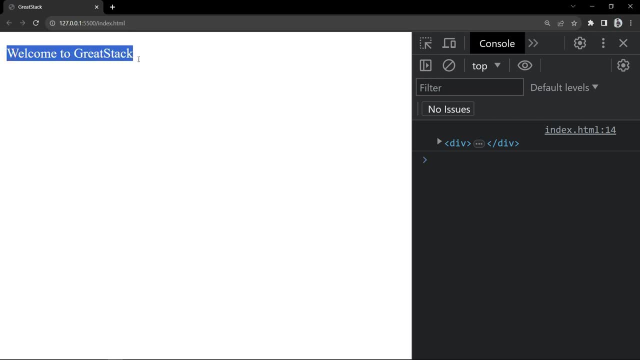 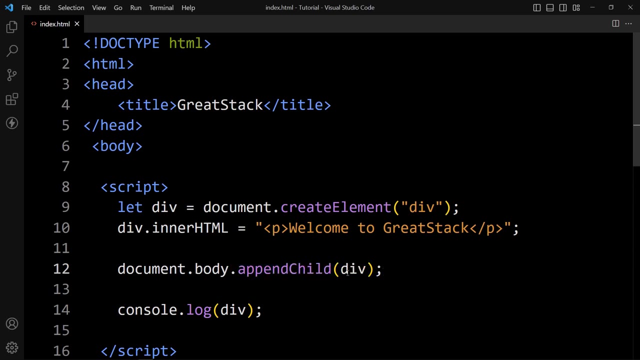 this newly created div. in this body we are adding appendchild div. so after adding this, come back to the web page. You can see we have text here: welcome to great stack, right? so this is added using this appendchild div that we have newly created. 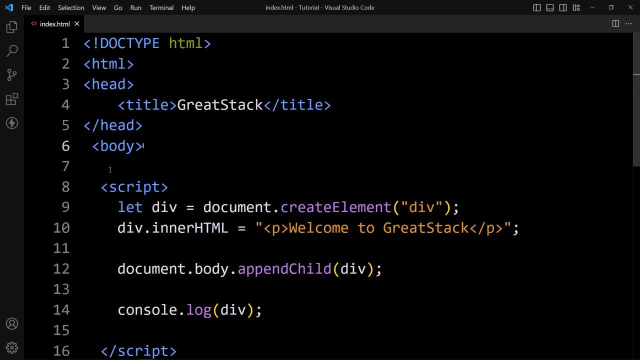 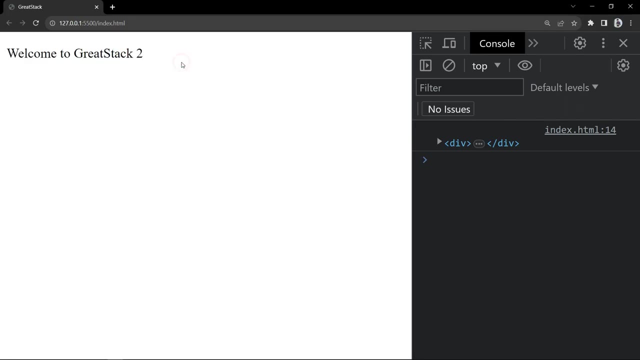 Within this body you can see we have not added any text in div or p tag. we are creating this element using this documentcreate element. if I change it, welcome to great stack 2,. you can see, it will be reflected here. welcome to great stack 2.. 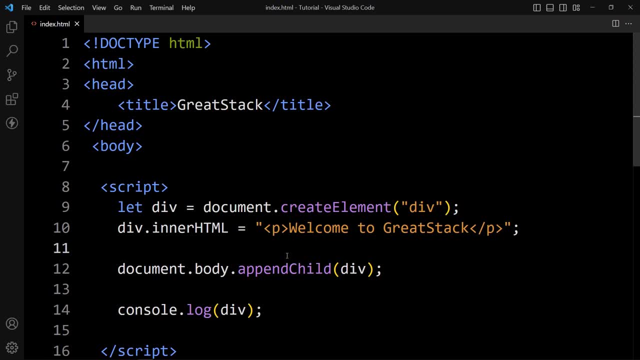 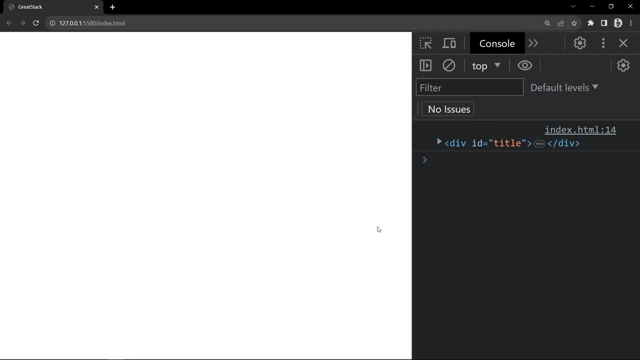 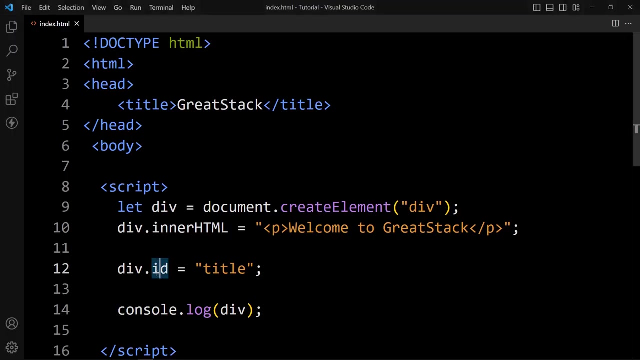 Now we can add the id or class name, anything in this newly created element. So here let's add: divid is equal to title. let's see: here we have this div with the id title. OK, now we can add the class name also just write div dot- class name. 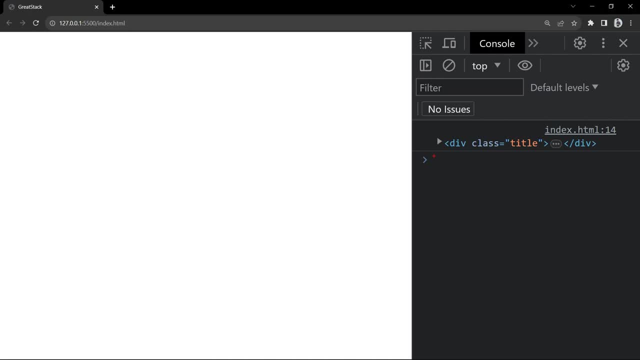 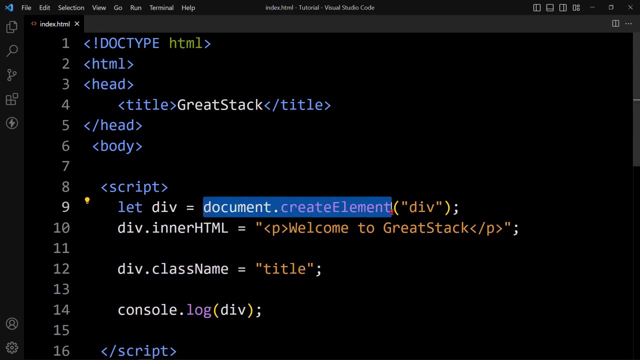 title and you can see the output here: div class title. so we can create a new element using document dot create element and we can add the content here. we can add the id, we can add the class name or any other attribute. next we will learn append child method. we use append child. 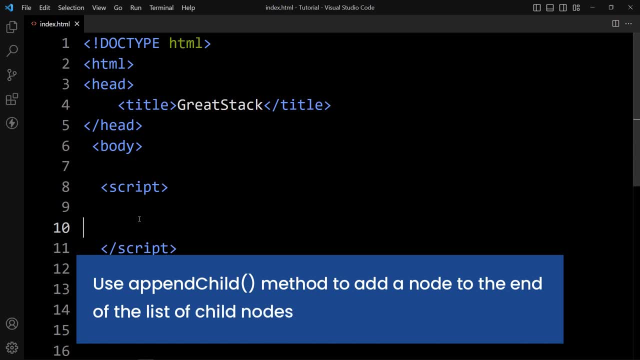 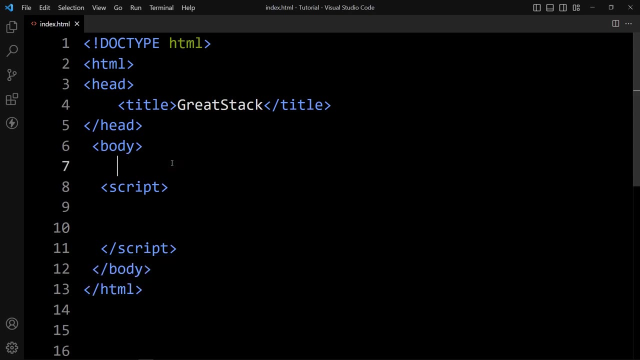 method to add a node to the end of the list of child nodes of a specific parent node. the append child can be used to move an existing child node to a new position within the document. so let's create some html elements here. here we will add one ul tag. 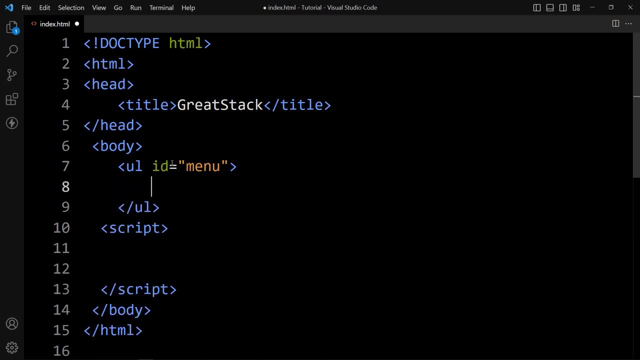 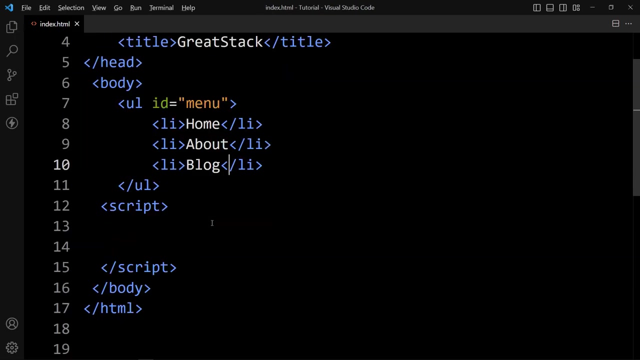 with the id menu so we can easily select it. here we will add some content in li home. second one is about. third one is blog. right, you can see these elements on the web page. home about blog. let's come back. let me add one more. here we will add project. 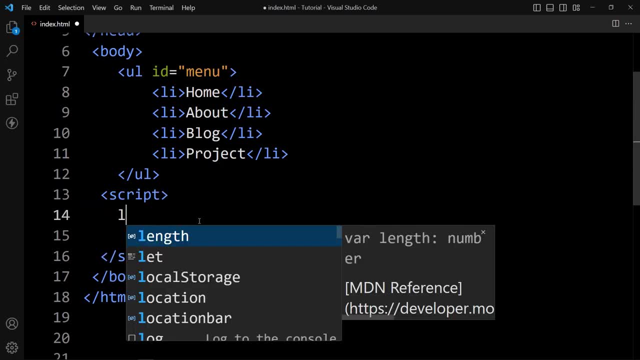 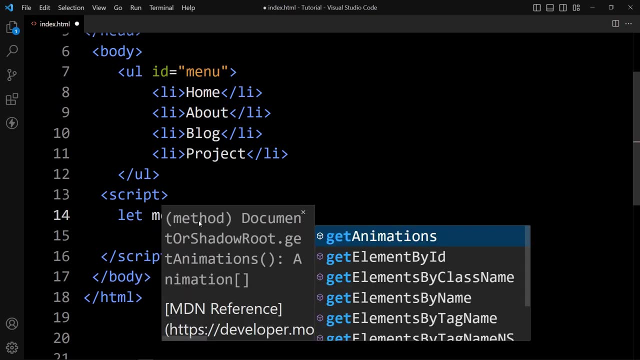 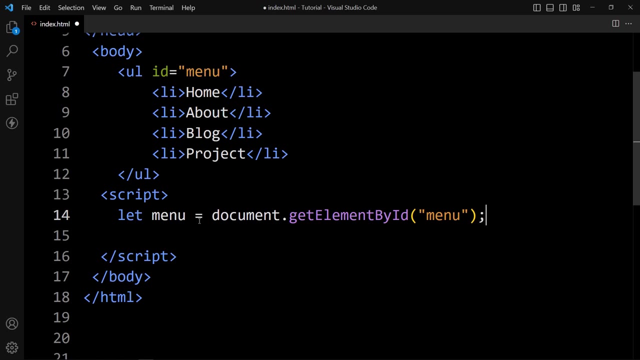 now within this script we will add let menu is equal to document. dot get element by id and the id is menu, so it will select the ul element. now we have to create one element and we will add that element in this ul. so here let's add let list is equal to document. 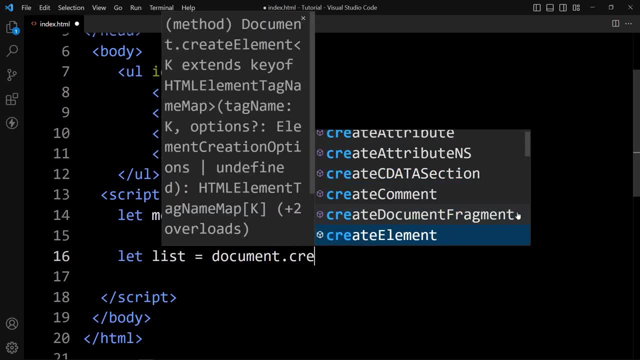 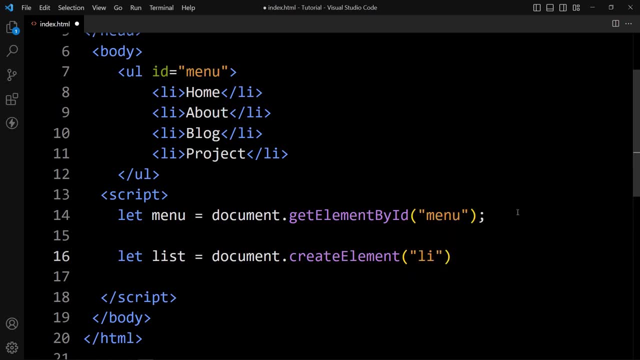 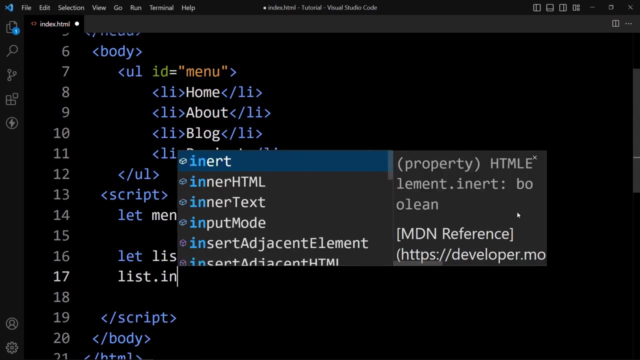 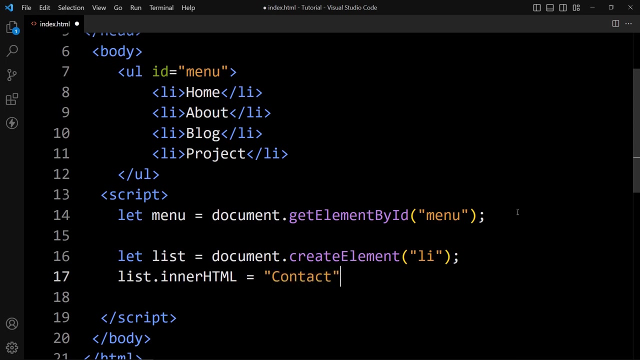 dot create element and the element tag name is li. so it will create one li element and its name is list. so in this list we will add inner html and through this inner html we will add one text contact like this: now we can use menu dot append child. 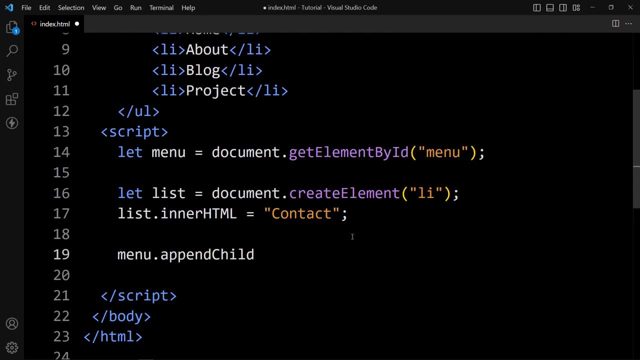 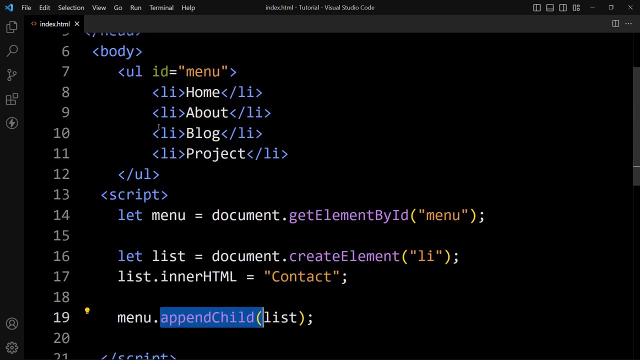 dot append child list. so this is the element which is here ul, and this append child will add this list at the end of this list. in this list we have home about blog project, so it will add the newly created list item after this project. so here we have created one list. 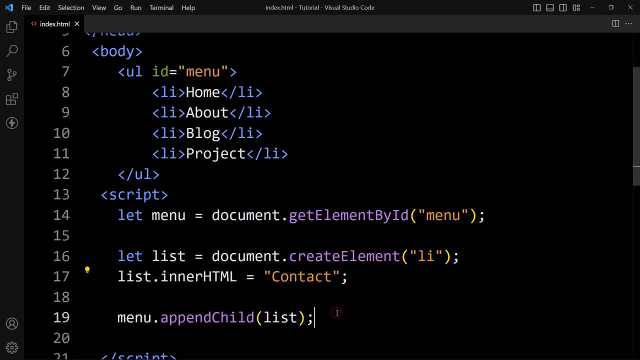 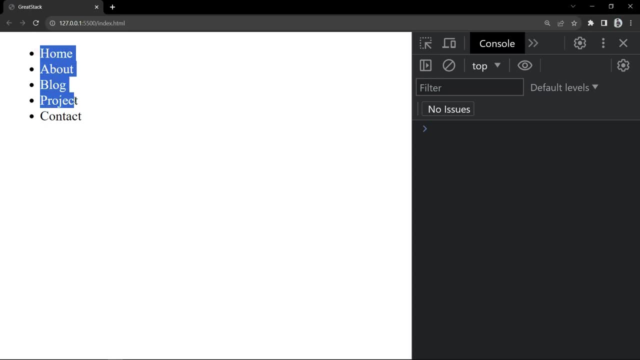 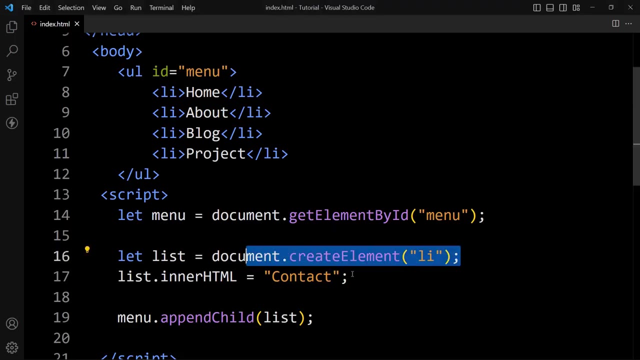 item and the text is contact. so this contact will be added after this project. you can see on the web page here we have home about blog project and after this project we have contact that we have created using this create element and added using append child in this project. 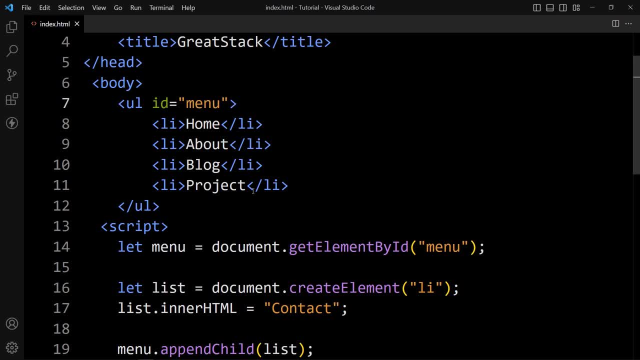 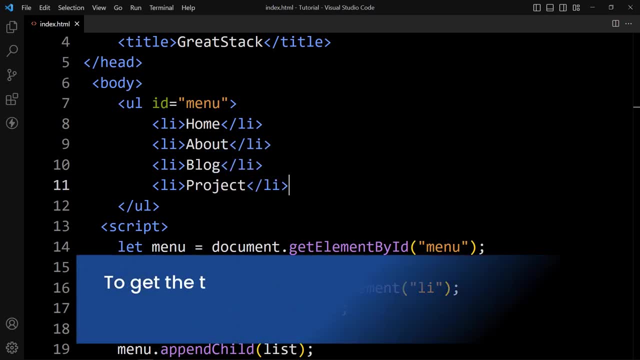 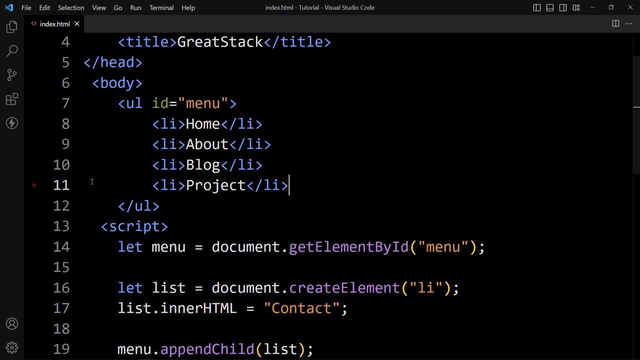 ul. so this newly created list will be added at the end of this list. next, we will learn about text content. to get the text content of a node and its descendants, you can use the text content property. so let's see one example. here we have the same html elements. 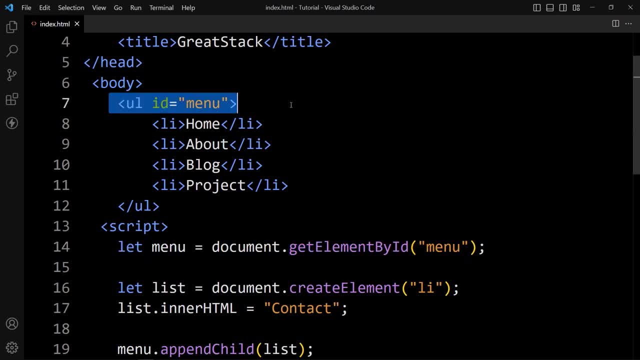 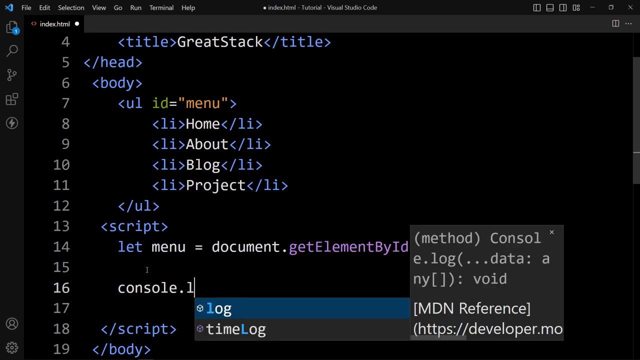 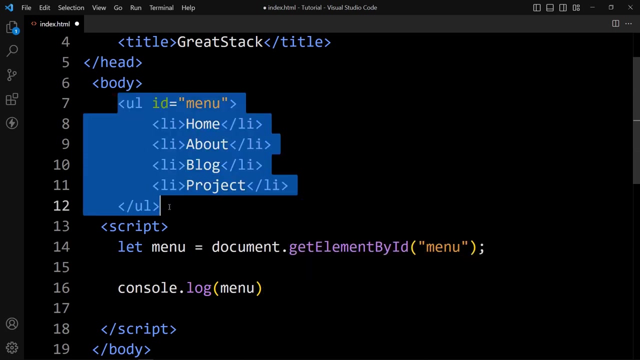 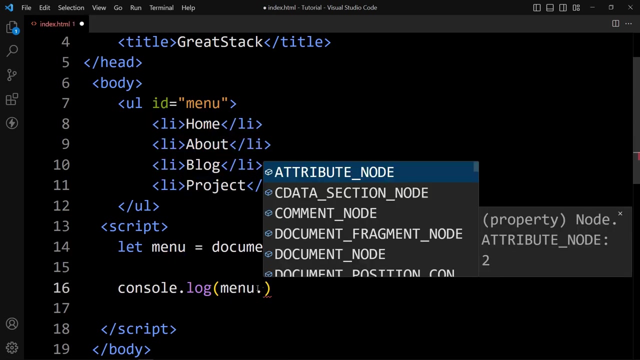 in this script we have added this line that will select this ul element and after that remove this, and here we will just add console dot- log menu. so it will display the complete menu in the console tab. now we just want these text, so here we will add menu dot text content. 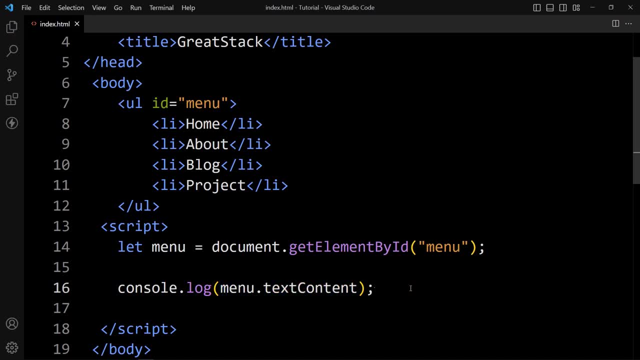 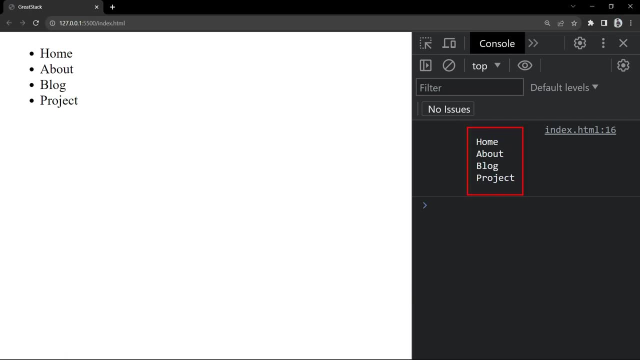 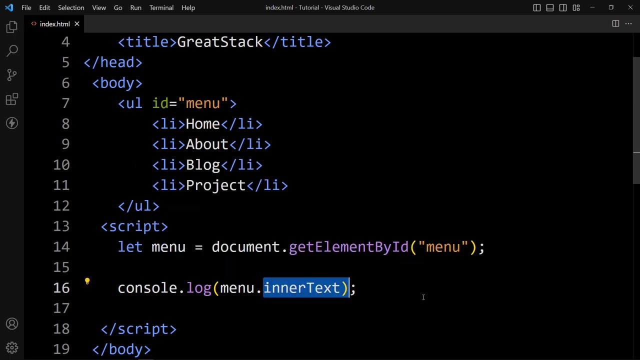 that's it. menu, dot text content and see the output in the console tab. here it is displaying home about blog and project, so it will ignore the html tag and display only text. now let's see one more thing here. if i write inner text, we are adding inner text and see the output. 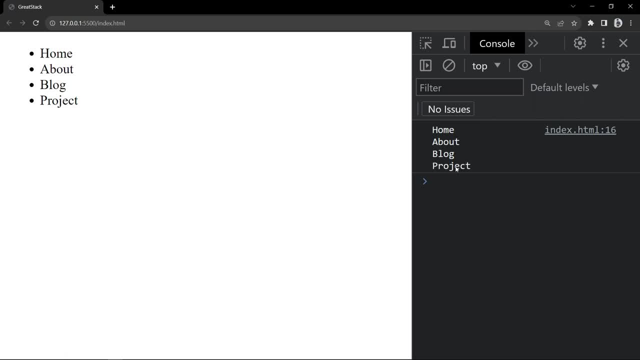 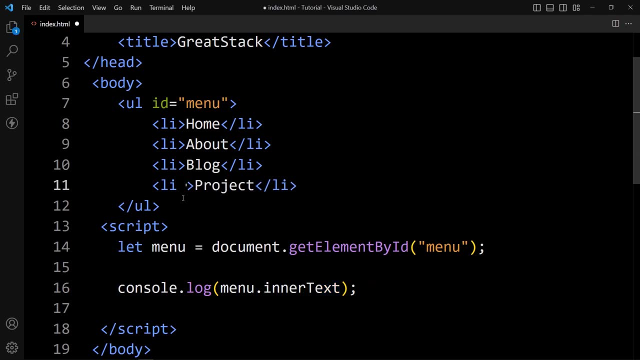 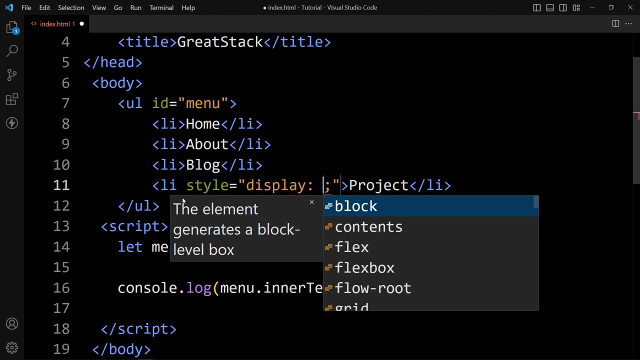 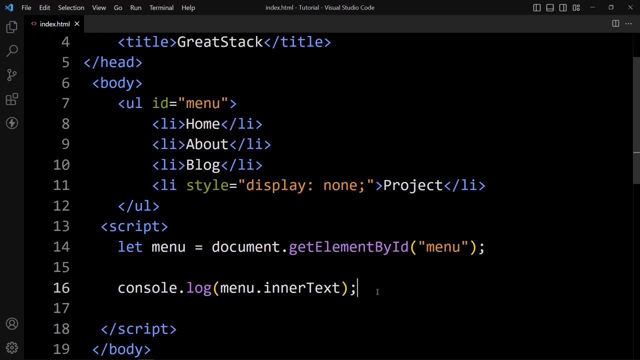 still, it is displaying home about blog and project. but there is another thing that we are adding here. i'm just setting the default default level here. but there is one difference in this: inner text is following the css also. but there is one difference: this inner text is following this css also. in this last one, if i add a style display none, so it will be hidden from the webpage you can see that is not visible. so it will be hidden from the webpage. that is not visible. so this in a text will return only visible text you can see. here we have home about blog and this home about log in. 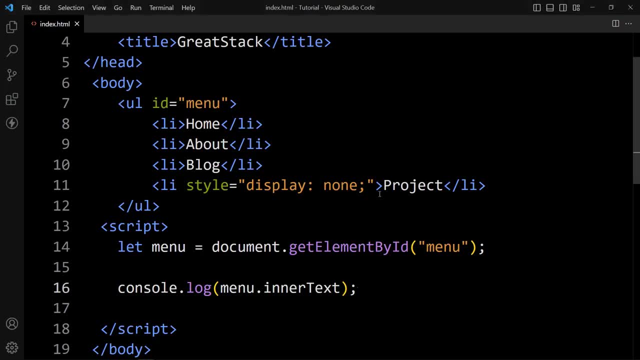 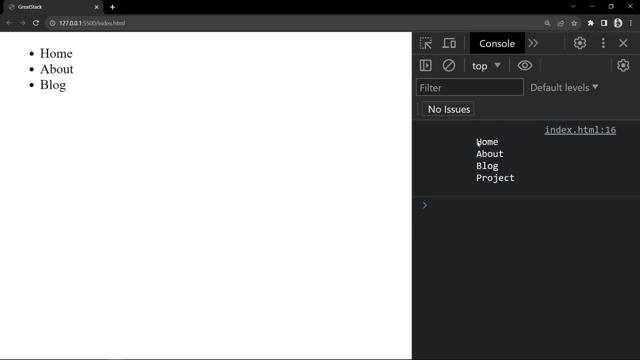 is here on the web page. but we have one more element here- project- which is invisible, but if i write text content it will display all the html text content you can see on the web page. we have home about blog only, but here it is displaying home about blog and project. so this text content. 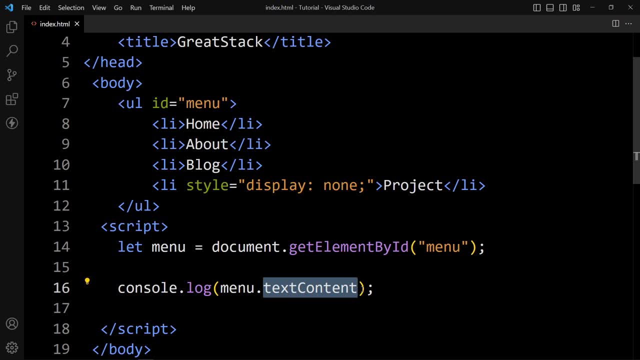 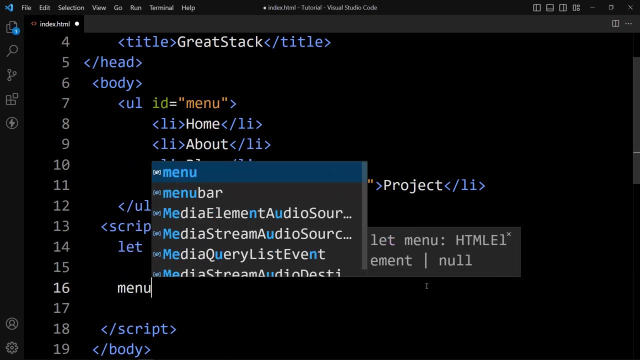 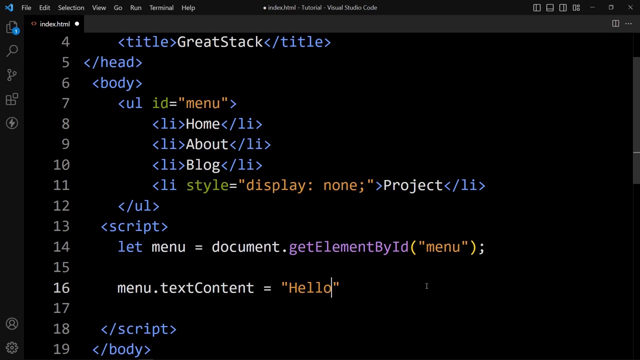 is displaying all the text inside that element and inner text is displaying visual text. only now we can use the text content to insert the text. also. let's add menu dot text content is equal to hello. so in this menu right now we have these list, so it will remove this. 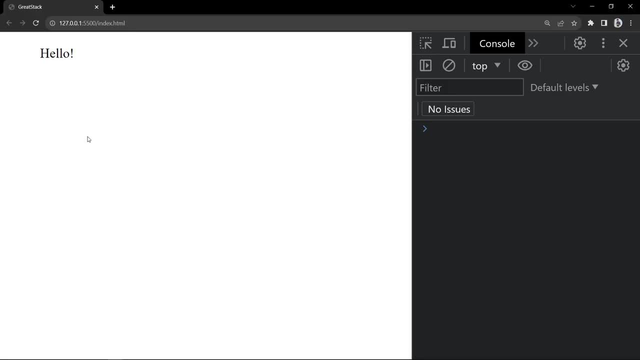 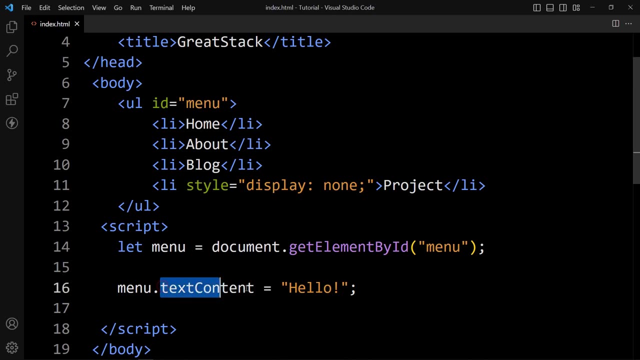 list and it will add hello. let's see the output here. you can see we have only hello in this web page, so we can read and add the text using this text content on the web page. next we will learn about inner html, so inner html is used to add the html code. 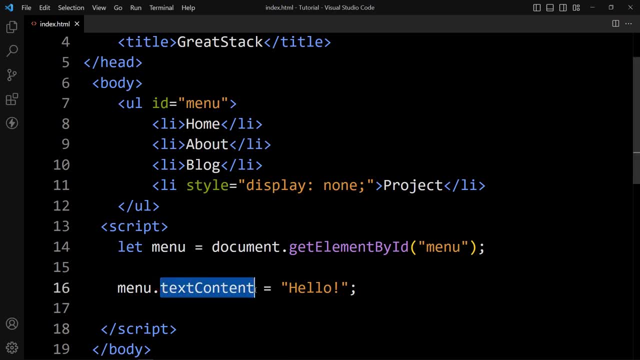 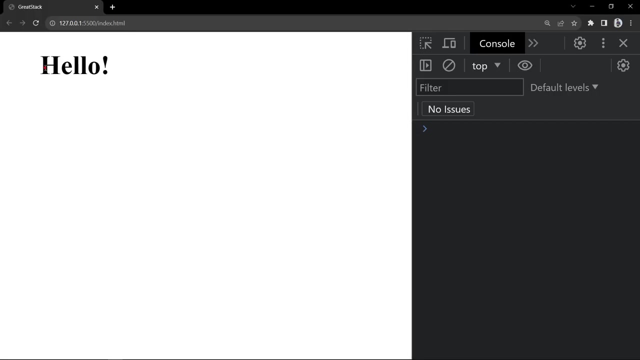 on the web page. so here we have added text content. so instead of this we will add inner html and see the output on the web page. you can see we have hello, so it is in the normal text. so here, if i write h1, it will add this hello text in heading. so it is in heading style: hello. so this inner html. 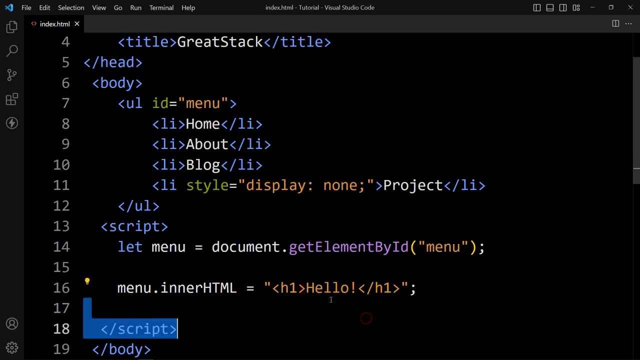 accept the html tags and add the text on the web page, but instead of this inner html, we will add text content. now you can see what will happen. it will add this as a plain text. h1 is also displaying here, and if i add inner html, it will add this text and this hello text will be in the 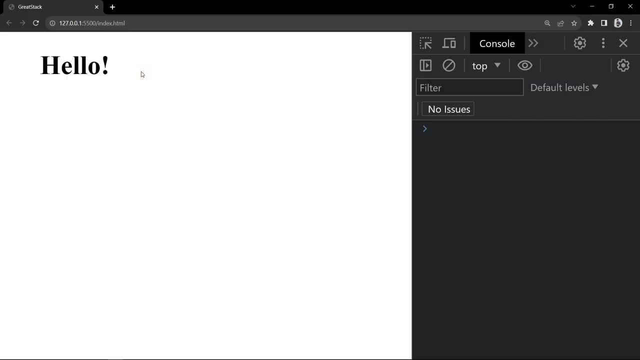 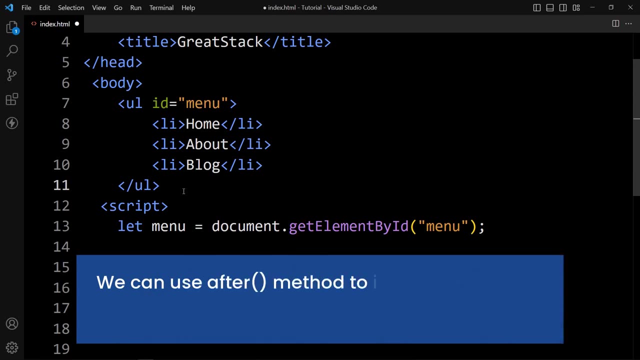 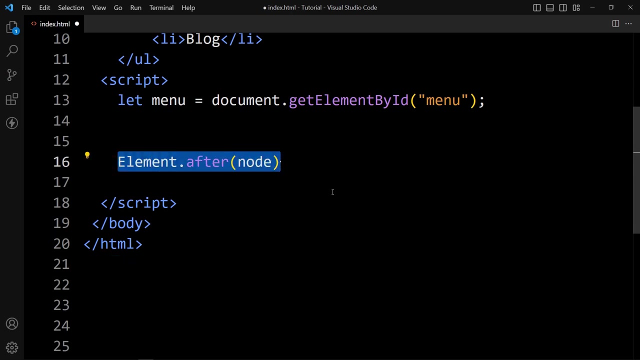 heading style. you can see this hello text on the web page. next one is after method. we can use after method to insert one or more nodes after the element. so this is the syntax for after method we have to add the element name, then after method and we have to pass a new node that we want to add after that particular element. 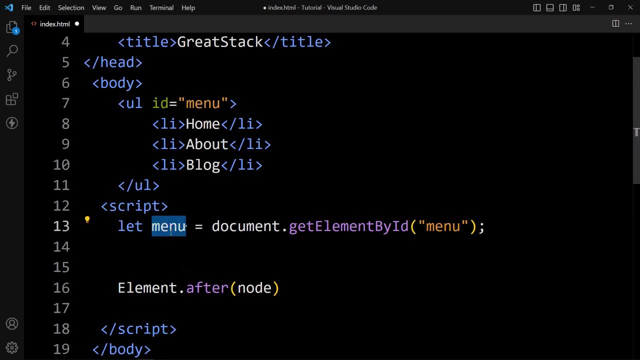 suppose we have this menu element so we can write this menu. then after method in this one we can pass a new element and we can create a new element using the create element method. this after method can accept multiple nodes, so we can add multiple element after this menu. it can also add a string. 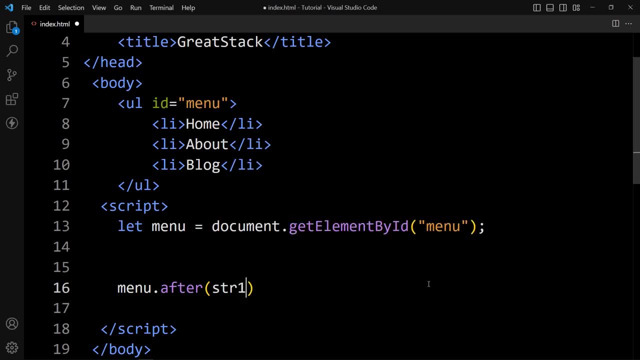 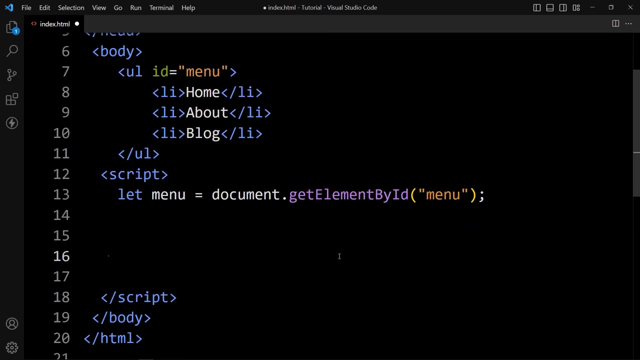 after the element. so we can add multiple string: str1, str2. like that we can add multiple string after this menu element. so so this is the use of this after method. now let's learn about append method. so this append method is also similar as append child, but in the append method 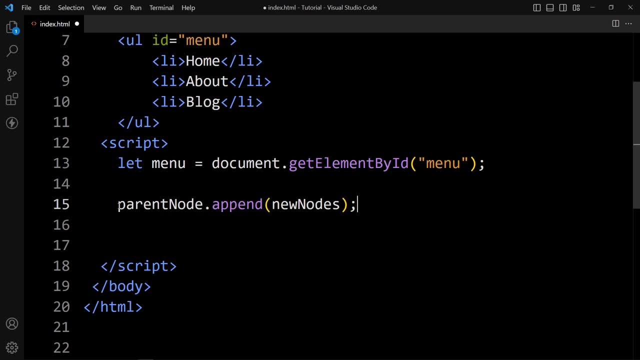 we can add multiple elements. this is the syntax for append methods. we have to add the parent element, then append. then we have to pass a new element that we want to add in that parent element. so this new node or new element will be added in the parent element at the end of the list of. 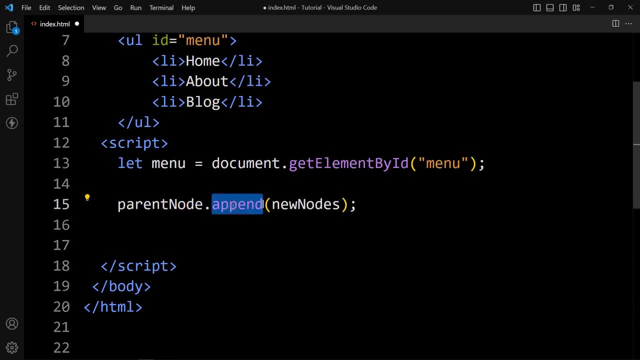 childs. so what's the difference between append and append child? so this append will accept multiple nodes and it can add string also. the next one is prepend method. so this is the syntax for prepend method: parent node dot prepend and new nodes. so it will add the new node as a first child in this parent node. so this is the prepend method. the next one is insert. 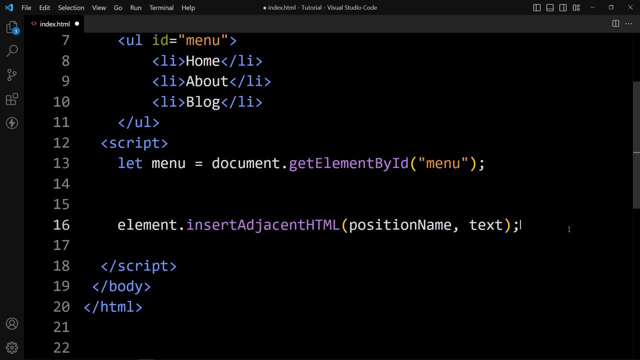 html. so this is the syntax for insert adjacent html. here we have to add one element, then insert adjacent html method, and here we have to give position and text. so suppose we will add this element menu and we want to add one text at the end of this list. so here we have to give. 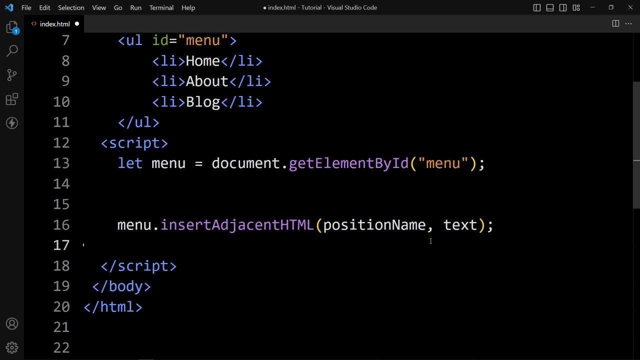 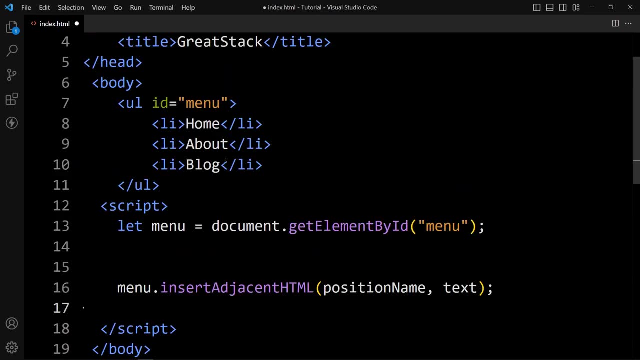 the position. so the position can be before begin, after begin, before end and after end. so suppose we add before begin. so this element is starting from here. so this before begin position means it will add the new node before this ul, and if we add after begin it will add it here. 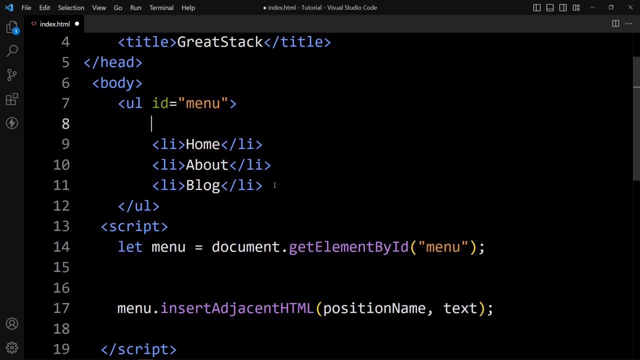 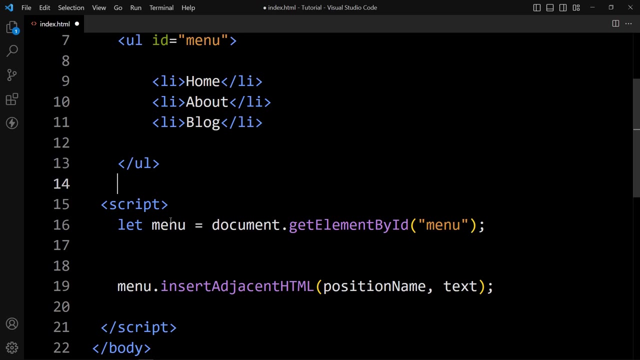 at this position. and if we add position before end, so this is the end, so it will add before end here. it will be added in this line. and if we add after end, so it will be added after closing of this ul. so let's test it here. we will add any one position, i will add. 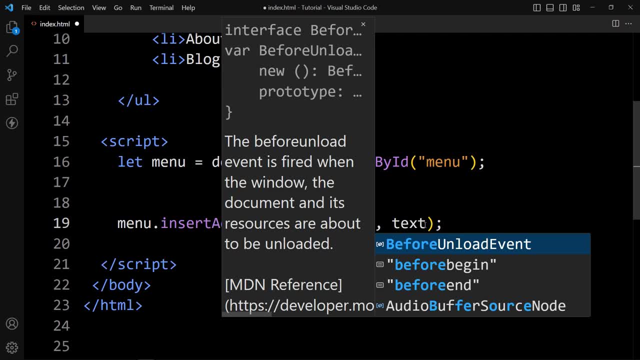 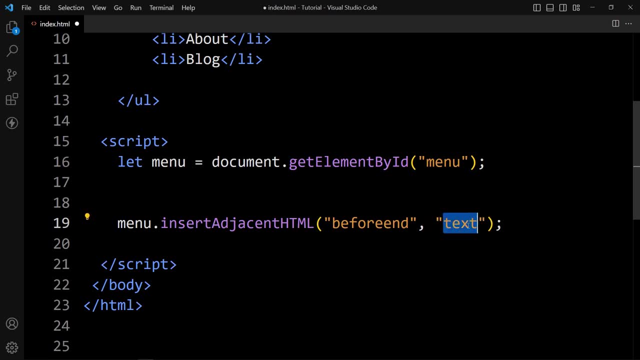 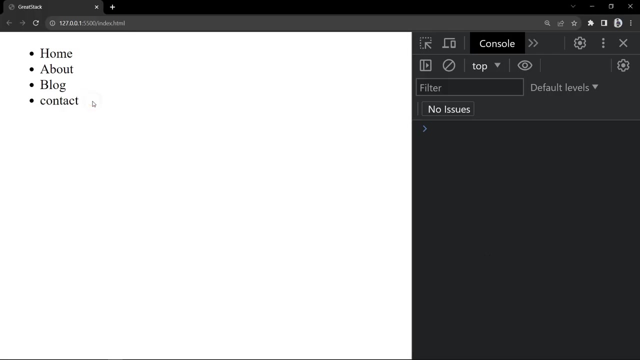 before end. let's add before end: and here let's add li contact, like this. so here i am adding one html text and this is the position and this is the element where we want to add this. so you can see the output on the web page. the contact is added here. now let's come back, and if i add, 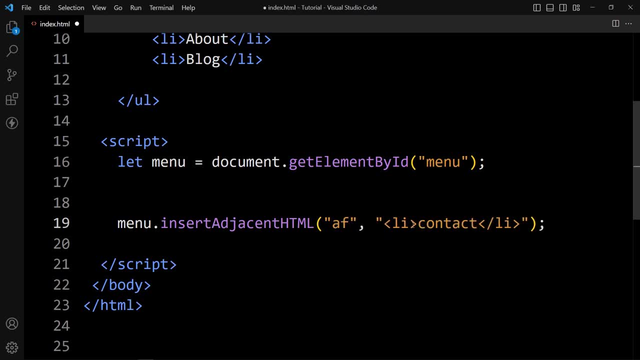 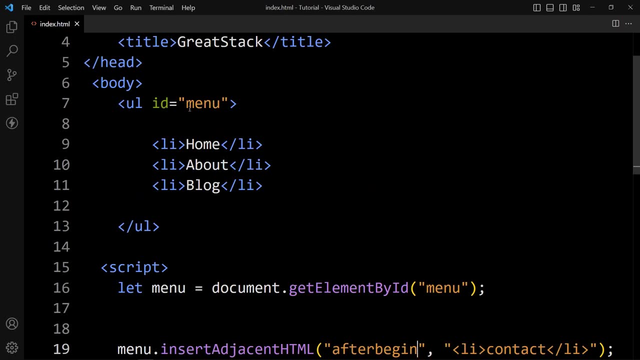 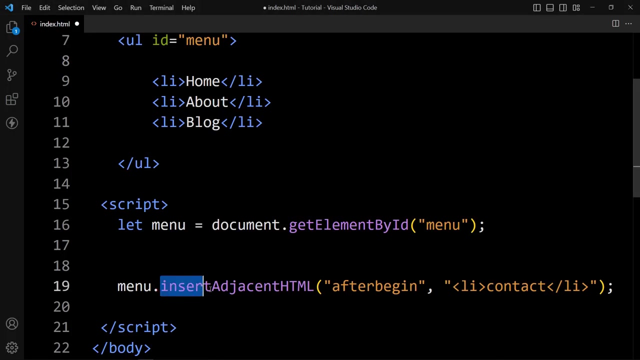 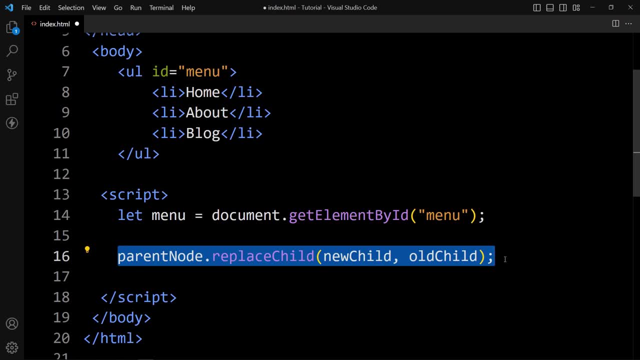 syntax for the replace child method. replace child method is used to replace the child element with the new one. so we can use this syntax. we will add the parent node, then replace child method. here we have to add the old child that we want to replace and here we have to add a new child. 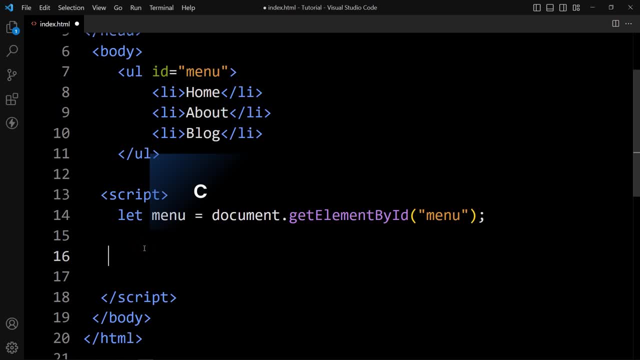 that will be replaced on the place of old child. next one is clone node method. we can use clone node method to clone an element. head is the syntax for clone node method. we will add the original node, then clone node, so this new node will have the another copy of this existing node. if i add menu, so this new node will have. 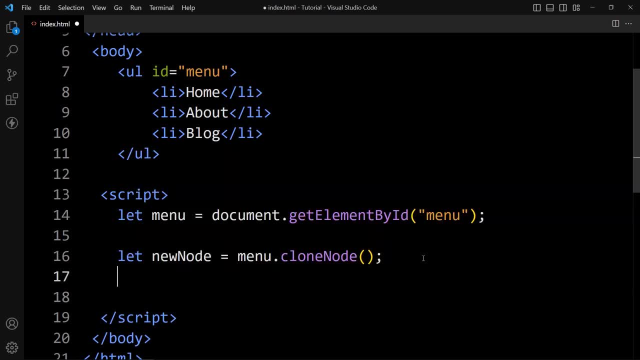 one copy of this menu element. let's print this one here. we will add consolelog, new node. you can see the output. it is displaying ul li menu. now let's come back and here we can pass the argument. so if i write true, it will clone this descendants, also this ul element and these li. 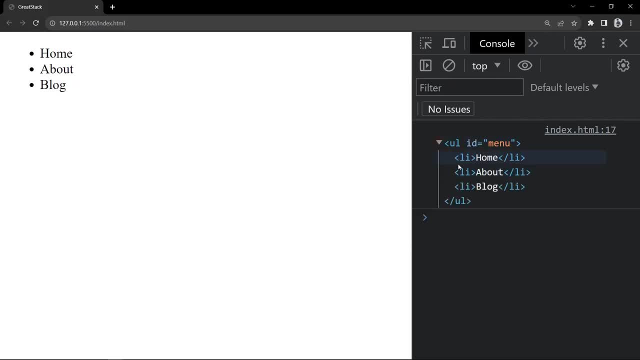 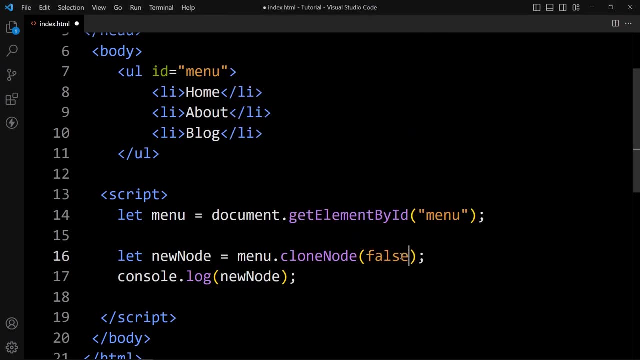 elements. also. let's come back. you can see we have ul and all these li and if i remove it or write false, by default it is false, you don't need to write. but if i write false, you can see here we only have ul element and if i 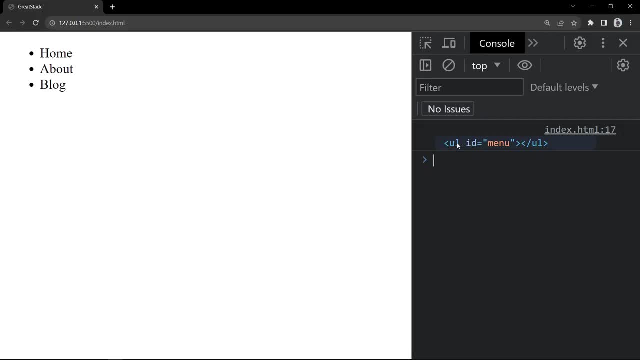 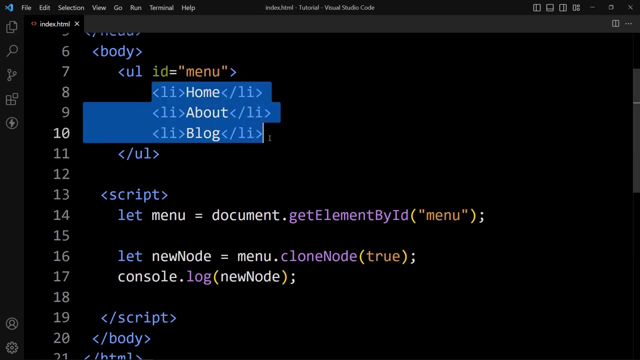 remove it. still it will be only ul and if i write true it will clone the element and all the child element also. you can see ul and all three li. so this is the clone node method. next one is remove child method. to remove the child element of a node we can use remove child method. here is the syntax for remove child method. here we have: 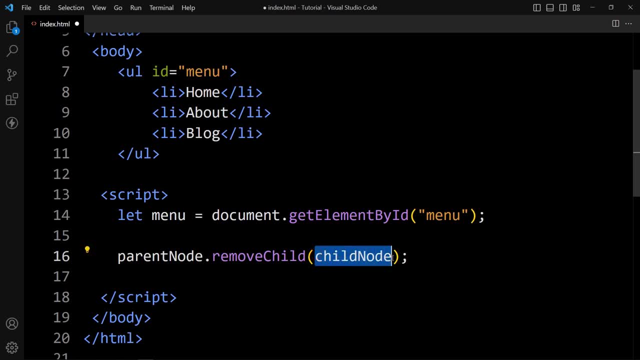 to add the parent element and then write the element that we want to remove from the parent element. so here let's add menu and from this menu, suppose i want to remove this last one. so here we will add menu dot last child element. so it will remove this blog. you can see on the web page here: 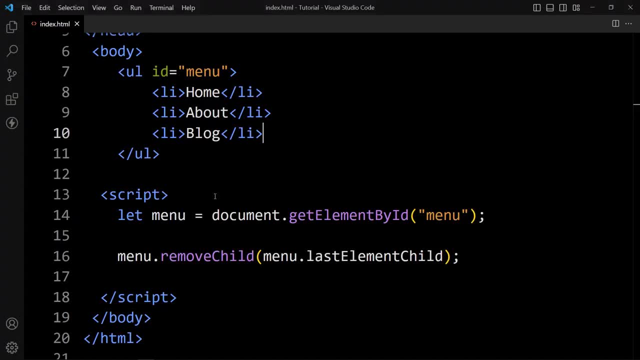 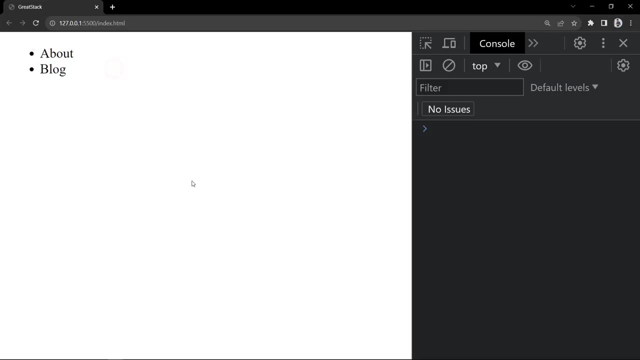 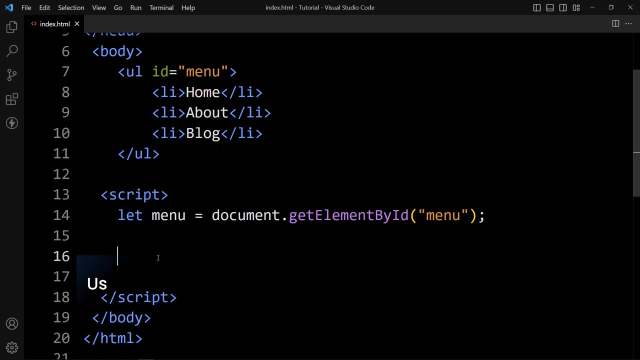 we have home about blog is missing if i write menu dot, first element child. so it will remove the first element which is home. you can see on the web page here we have about and blog. so this is the remove child method. next one is insert before method. we can use insert before method to insert a new node. 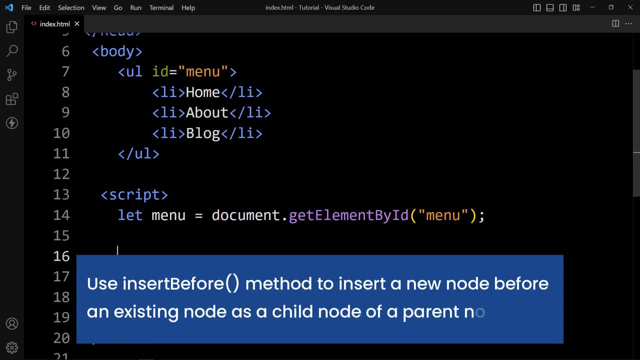 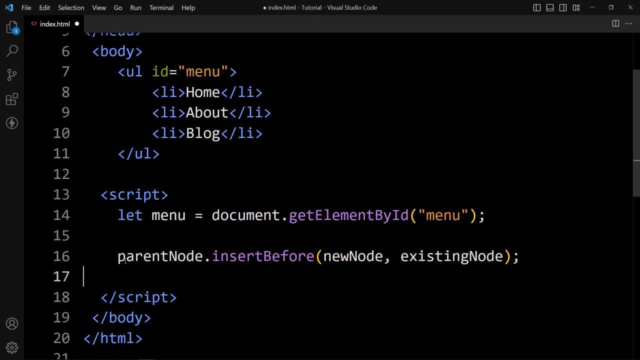 before an existing node as a child node of a parent node. here is the syntax for insert before method: we have to add one parent element, then this insert before method and it will accept two arguments in this one we have to add the new element that we want to add and we have to add the existing element. 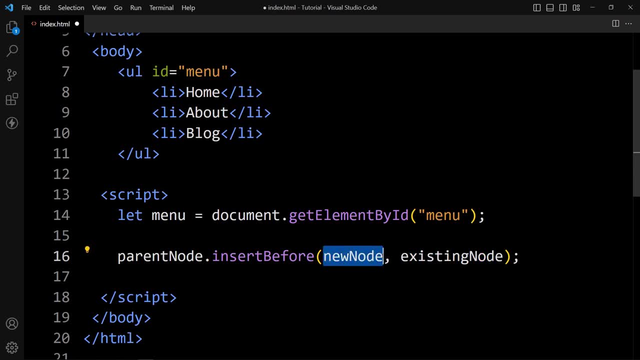 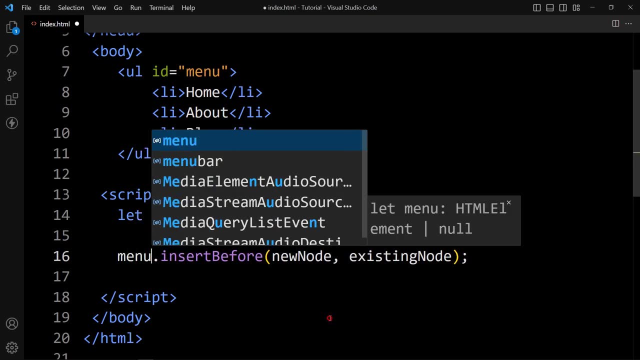 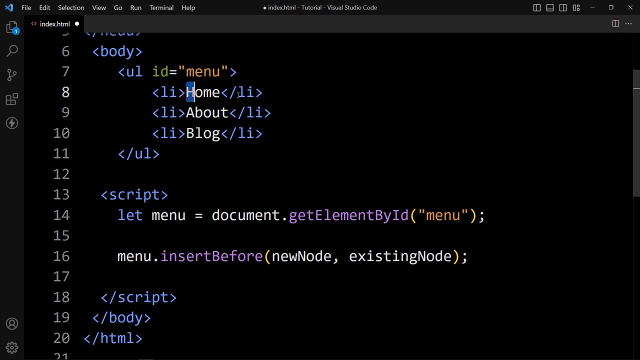 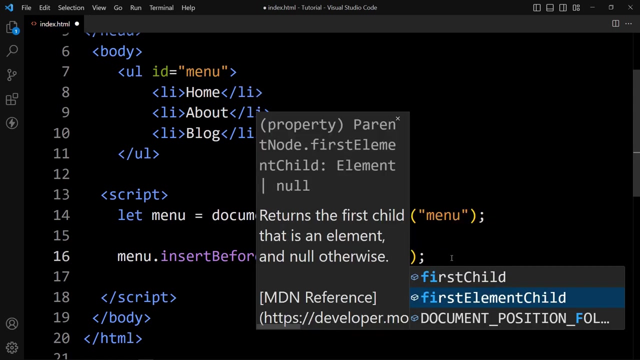 before that existing element. this new element will be added. we have the parent element menu, so we will add menu here and we want to add the new element before this li, that home link. so here we will add menu dot, first element: child. so this new node will be added. 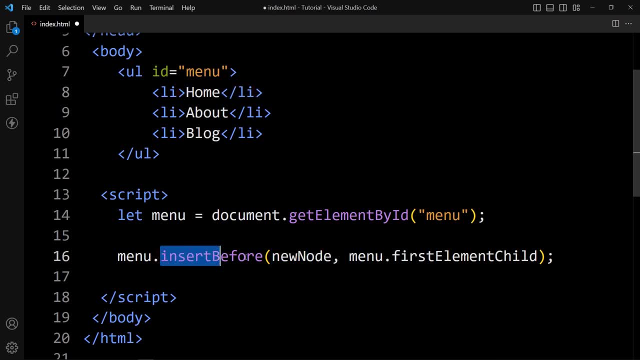 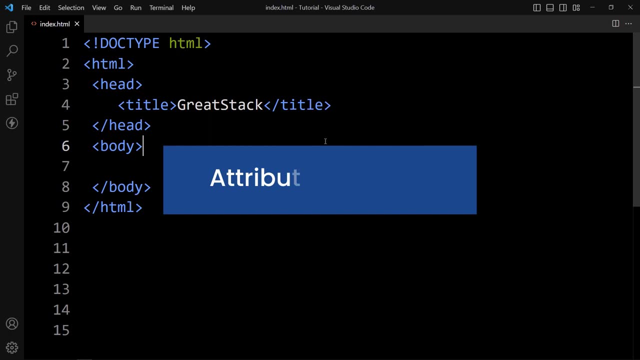 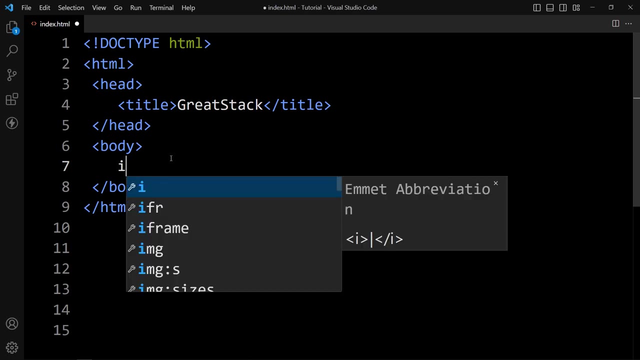 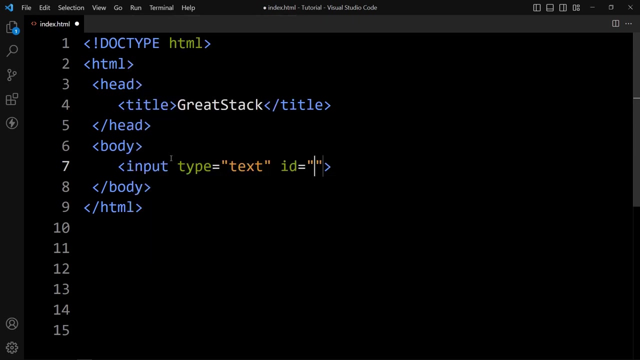 before this home. so this is the insert before method. so these are the methods to manage the play, the html elements. now we will learn about attribute methods, so let's understand what is attributes here. i will add one html element. input type is text. we will add one id, so let's add the. 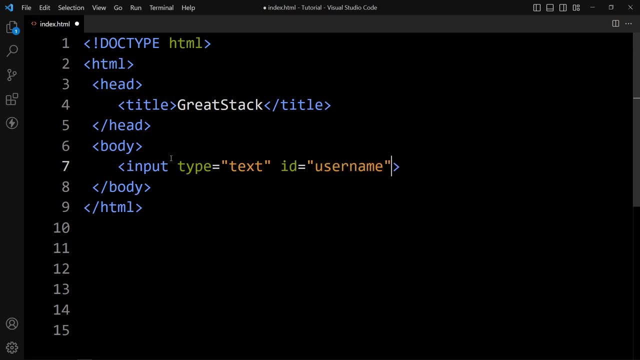 id, username, and we can add the placeholder also user name. so in this html tag we have added three attributes, which is this one, this one and this one. this is the attribute name and this is the attribute value. the id is the attribute name. username is the attribute value. this placeholder is the attribute. 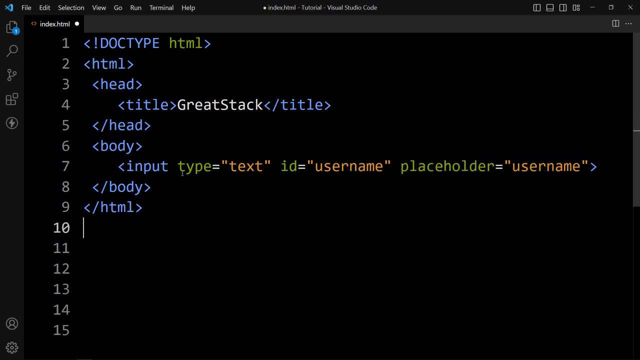 name and username is the attribute value. now how we can get the attributes of any html element using javascript. so let's add one script tag here where we will add our javascript code. first we have to select this element, so we can use any method to select the element. let. 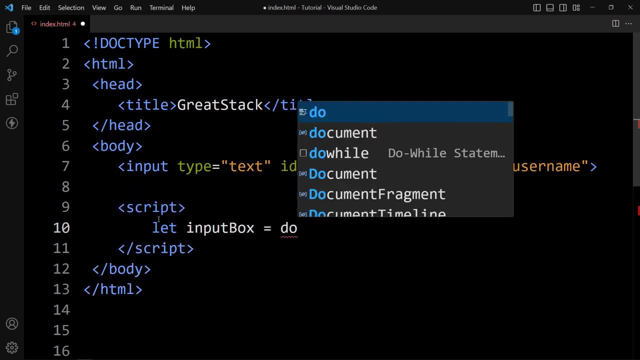 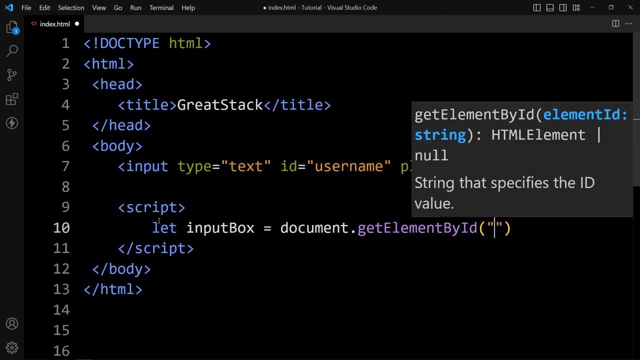 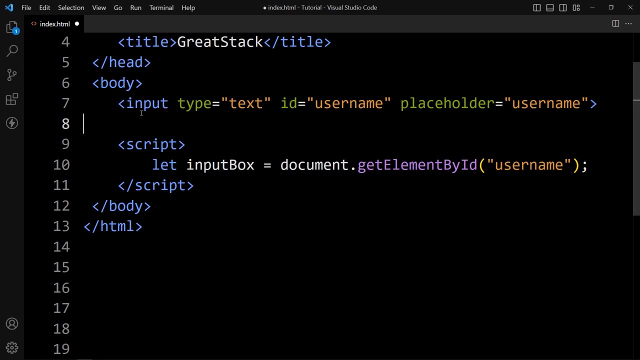 input box is equal to document: dot. get element by id. i'm using get element by id method and we will end this id using element dot. i'm using get element by id method and we will add this id username. After selecting the element, we can find the attributes available in this HTML element. 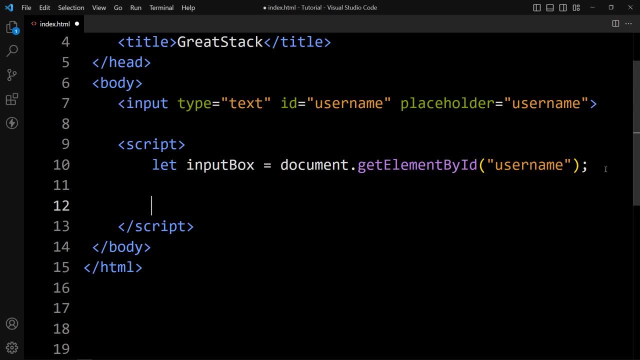 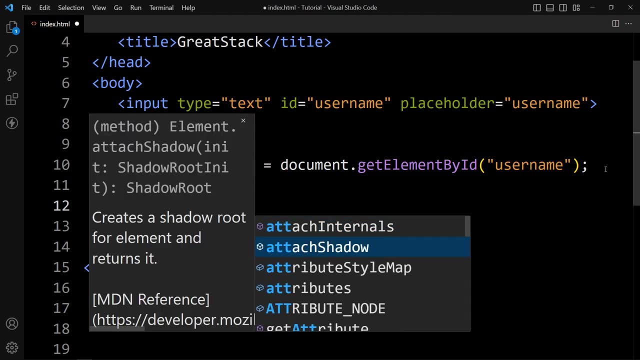 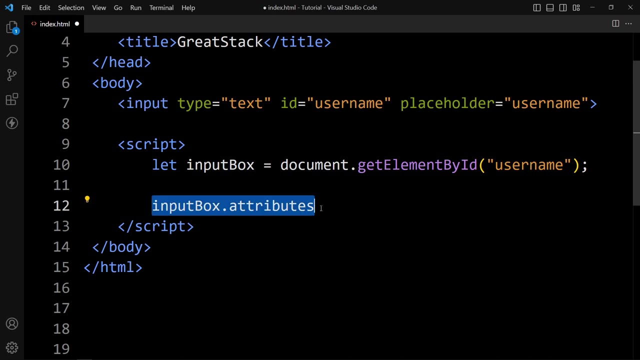 So to get the attribute, we will just add the element which is input box And after that just add attributes. That's it. It will give all the attributes available in this HTML element. So to print this in console, we will add console dot log and add this code: input box dot attributes. 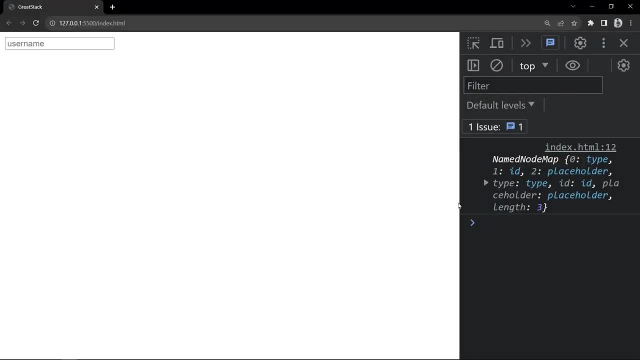 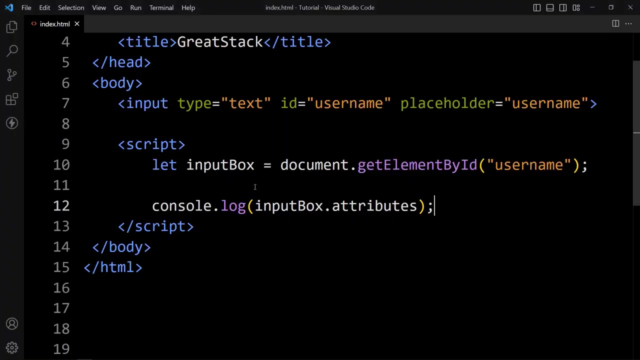 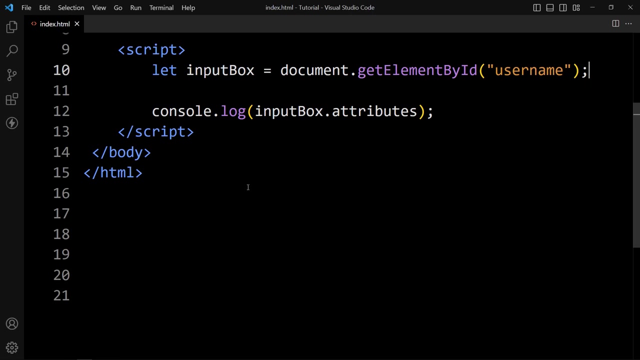 After adding this, let's come back to the web page and you can see the console tab. It is displaying type, then ID, then placeholder. So we have three attributes in this HTML element. Now we have some attribute methods to get the attribute value and to set the attribute of any. 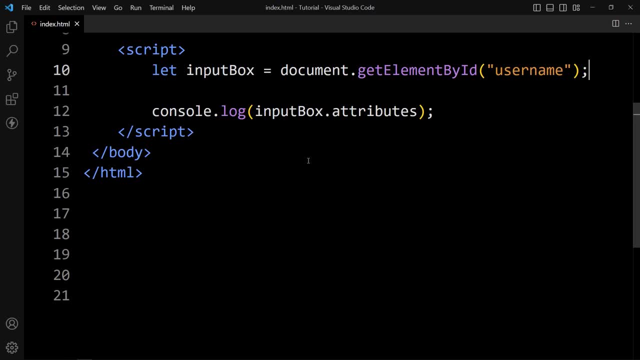 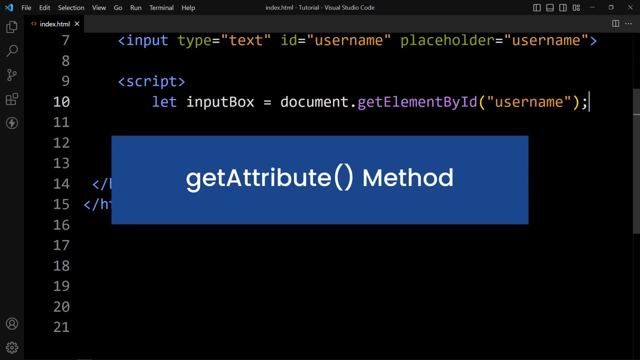 HTML, We can check for some attribute, whether it is available or not, and we can also remove the attribute using the attribute methods. So let's see the first method, which is get attribute. So instead of this we will add the element which is input box, And here we will add: 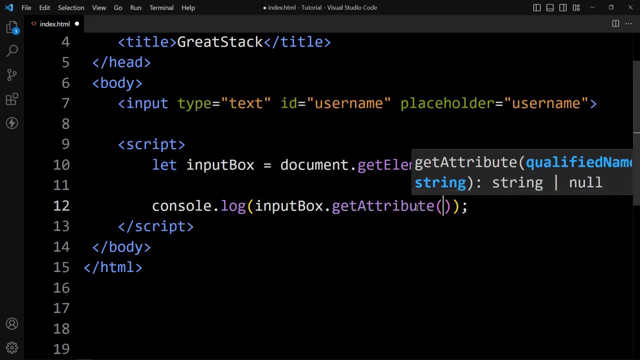 get attribute and in this get attribute, we have to add one argument, So we will add the attribute name. So here we have the attribute name, type. So just add type like this, And after that let's come back to the web page. 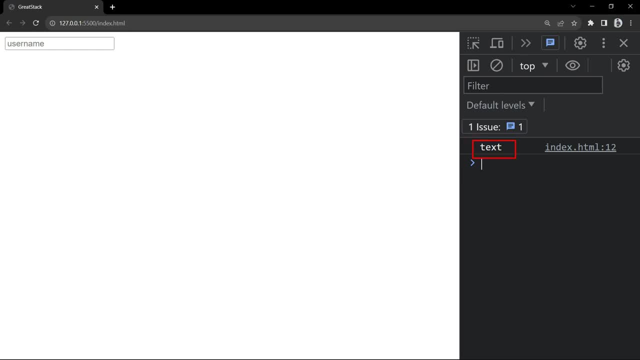 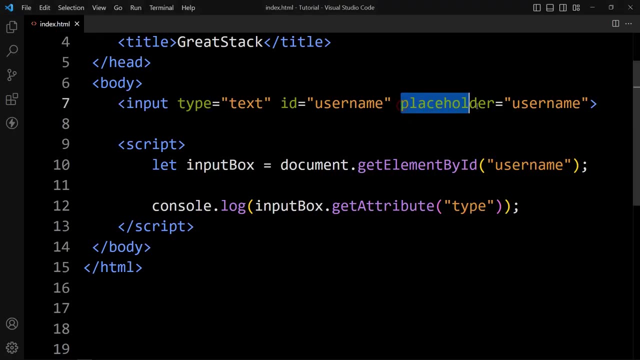 You can see here it is displaying text. So we can read the value of the attribute using the get attribute method. Let's take another example. Here I will add this placeholder: Write this placeholder here. Now it will display the value written in this placeholder attribute. So come back to the web page Here. 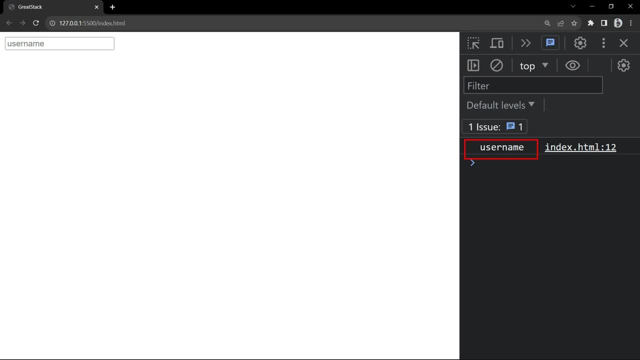 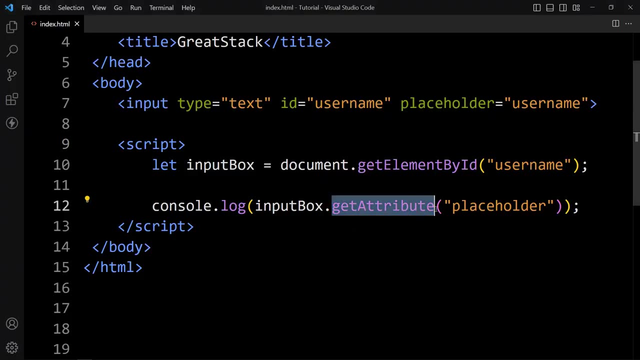 you can see, it is displaying username. This username text is available in the placeholder attribute. So this was the first method: get attribute to read the attribute value. Now we will learn about second method, which is set attribute. So let's remove this one. 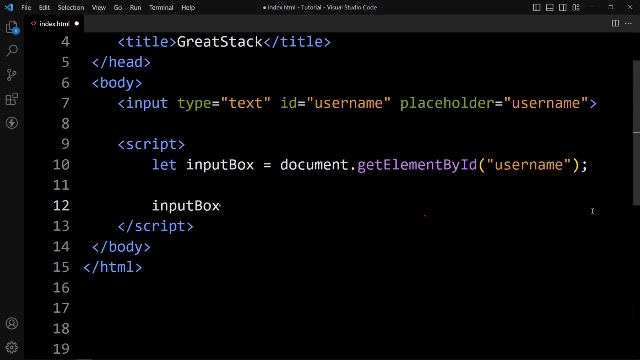 Here we will add the element which is input box. On this input box we will apply set attribute, and this set attribute will accept two argument. So the first argument will be attribute name and the second argument will be attribute value, like this: Here we will add the. 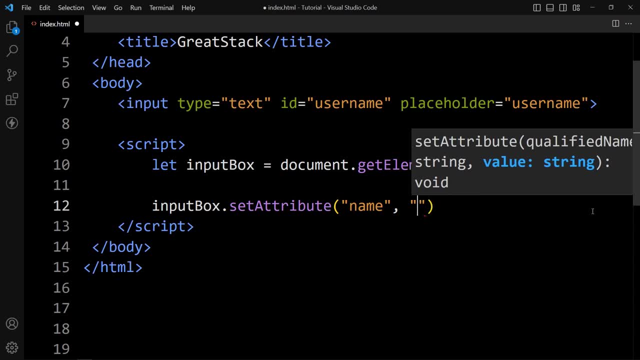 name, comma value like this: So let's remove this here and here we will add any attribute name. So let me add the class, So the attribute name is class, and here we will add one value. Let's add the class name user Like this: So it will add one attribute which is class and the value is user. 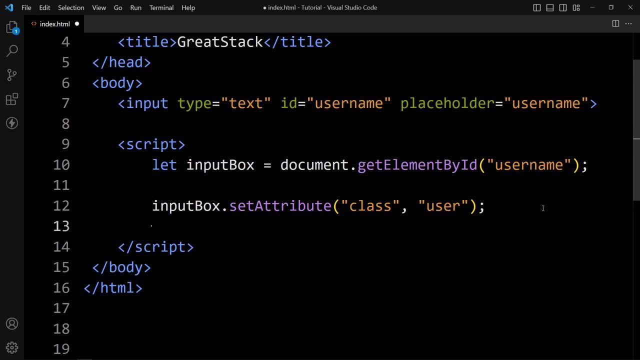 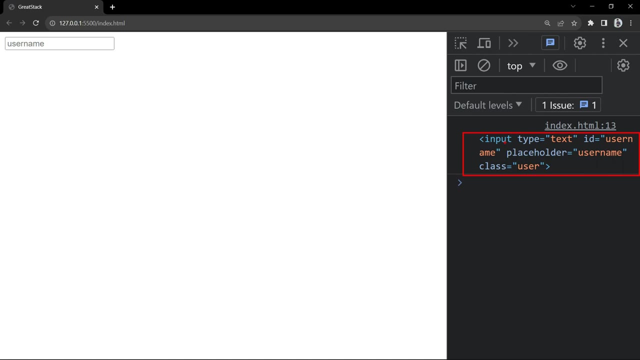 Now to see the updated input, let's add consolelog and here we will add input box, So it will display this complete element on the console. So let's come back to the web page. Here in this console you can see we have the input element with the type text: id, username, placeholder. 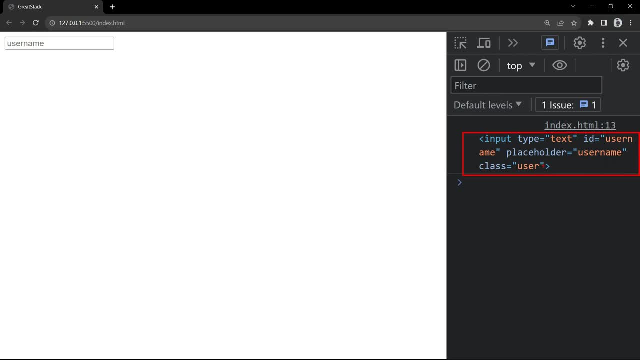 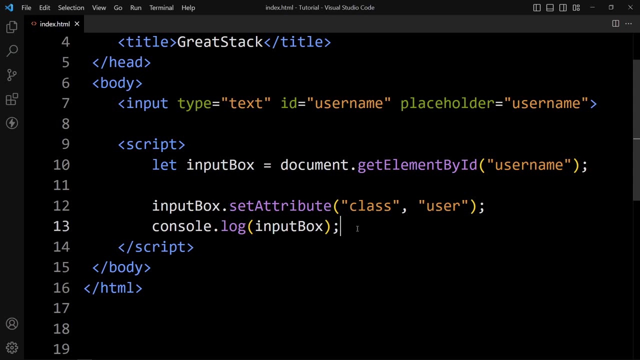 username. And there is one more attribute, which is class user, that we have added using this input dot set attribute, class user. So this was this set attribute method. Now we will learn about next one, which is has attribute. So it will tell us whether this attribute is available on the element or not. It will result in true or 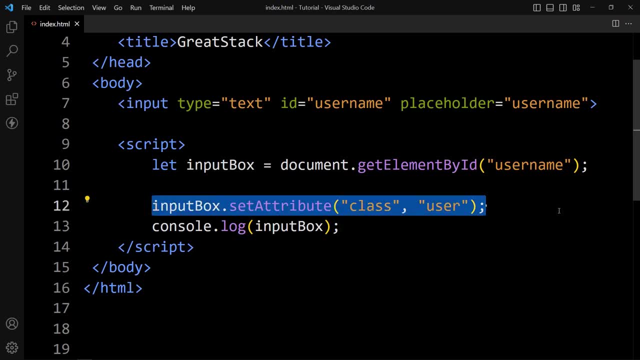 false. so here we will add another example. we will add the element input box then has attribute, and this will accept only one argument. so in this one let's add class, and it will return one true or false value. so we can directly print this one. so just add consolelog: input box has attribute, class. so you can see in this: 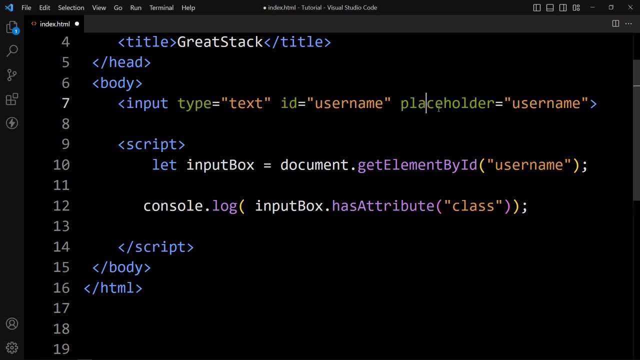 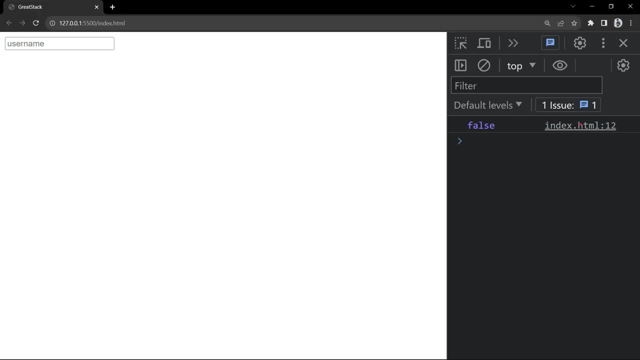 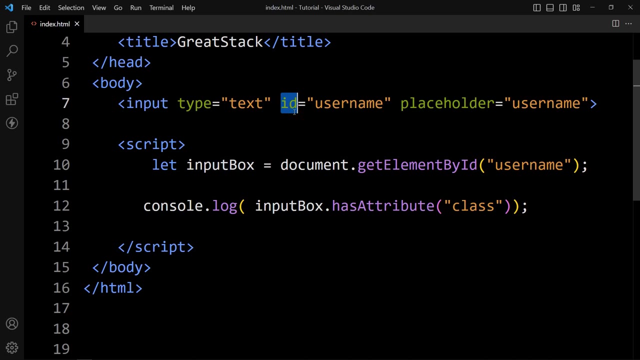 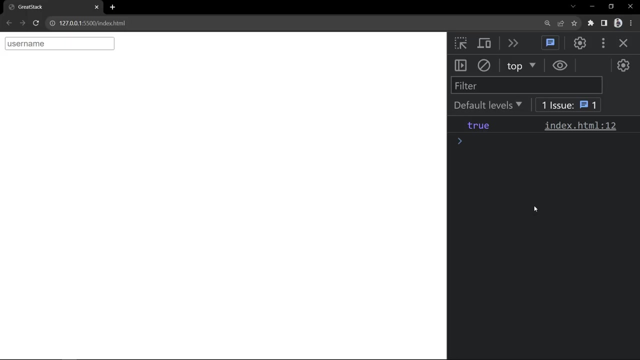 input field we have the type id and placeholder. we don't have class here, so it should return false. let's see the output. you can see it is displaying false. now let's come back and instead of this class we will add id, so it will return true. let's come back to the webpage. you can see it is displaying true in this console. 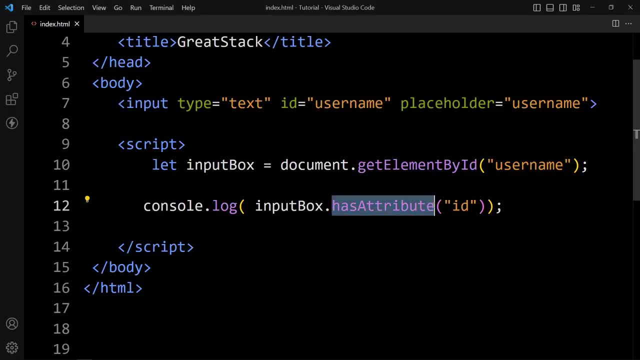 so this has attribute will return true or false value. if the attribute name is available in the input field, it will return true. if this attribute name is not available in the input field, then it will return false. so, using this has attribute, we can check the availability of that particular. 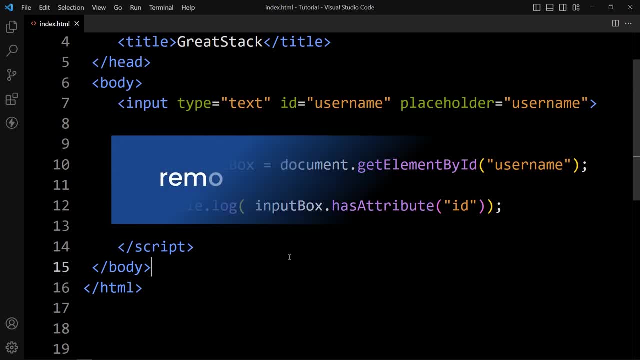 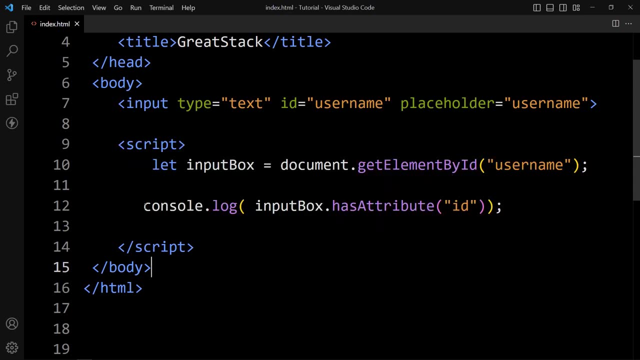 attribute on the element. next we will learn about another method, which is remove attribute. that will remove the attribute from the element. so in this one we will add element, then remove attribute, and in this remove attribute we will add one attribute name that we want to remove. so here, 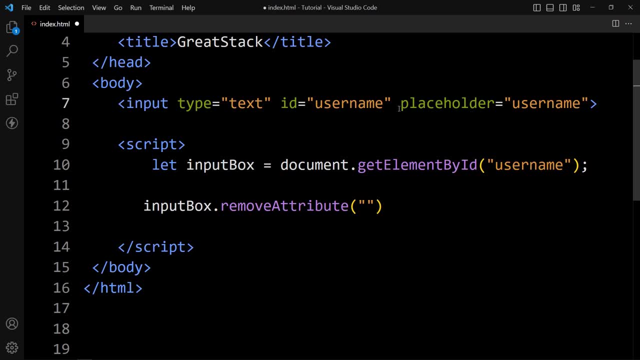 we have type id and placeholder, so let's try to remove this placeholder. just copy this one, paste it here, so this remove attribute will remove this placeholder from this input element. now we will just print this input element in the console, we will add consolelog input box and now we will see the output in console. here we have the input element and in 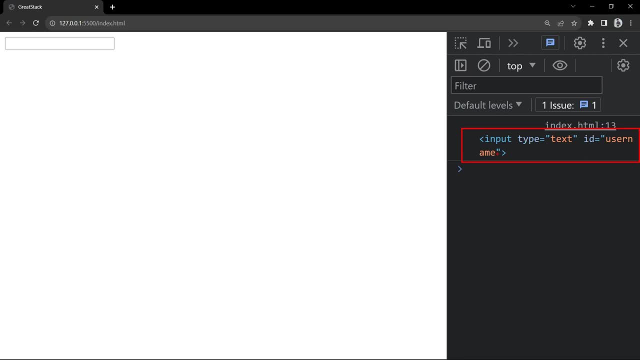 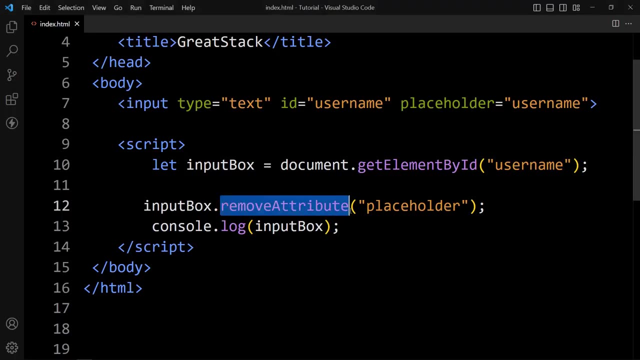 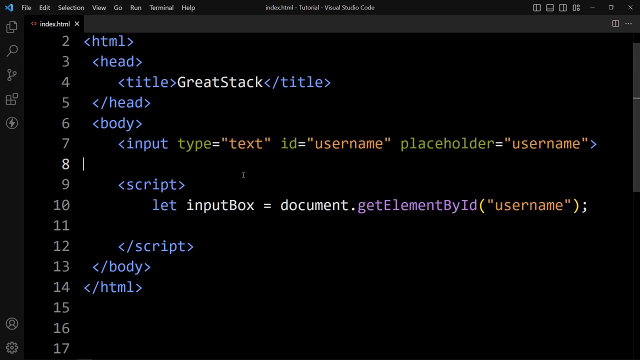 this input element we have type text, id, username, but here we don't have the placeholder, because in this code we have added remove attribute placeholder, so it will remove this placeholder attribute from this element. so these are all four attribute methods. now we will learn about manipulating elements style. to manipulate the style of the element, we have the property called 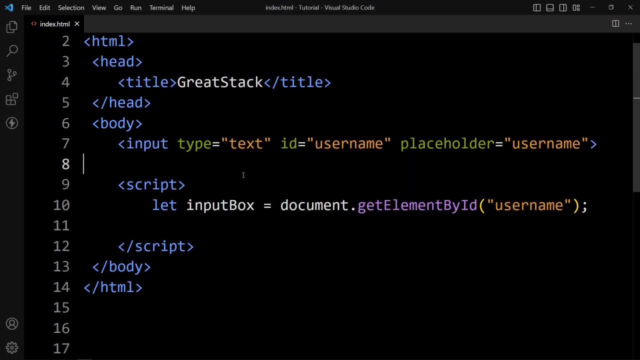 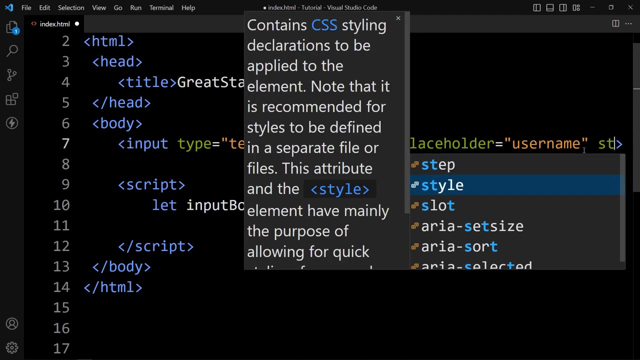 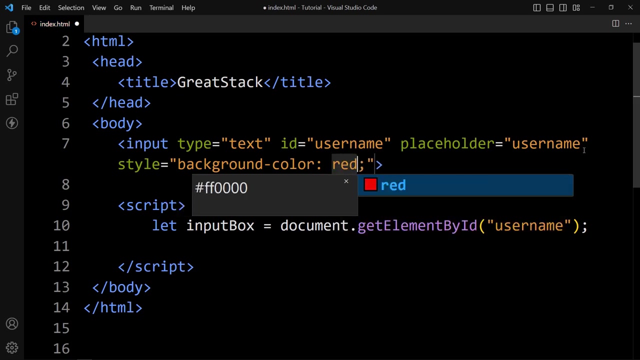 style and we can use this style property to get or set the inline style of an element. so here we have the HTML element, which is input, and in this one we don't have any inline style. so let's add one style here, and here we will add the background color value is red and let's add one more CSS. 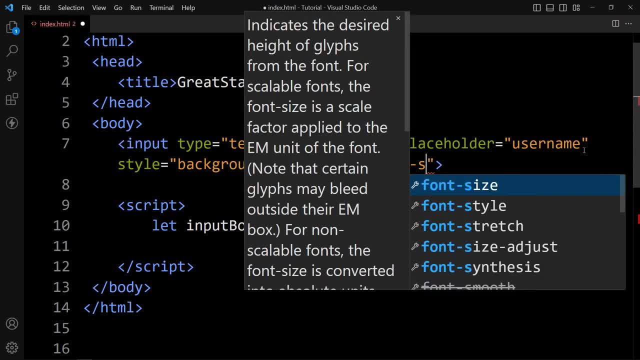 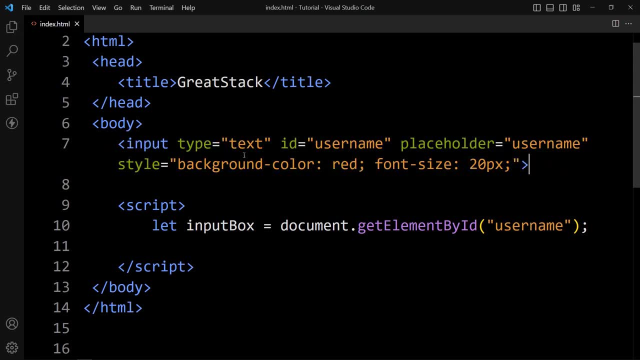 property here that will be font size: 20 pixel. so in this HTML element we have the HTML element which is input, and in this one we don't have any inline style element. we have added the inline CSS. in this one we have added the background color and font size. 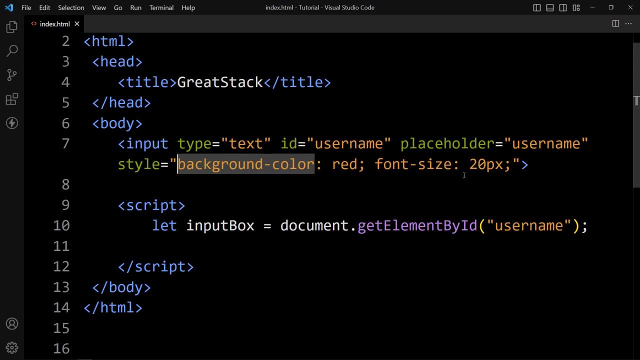 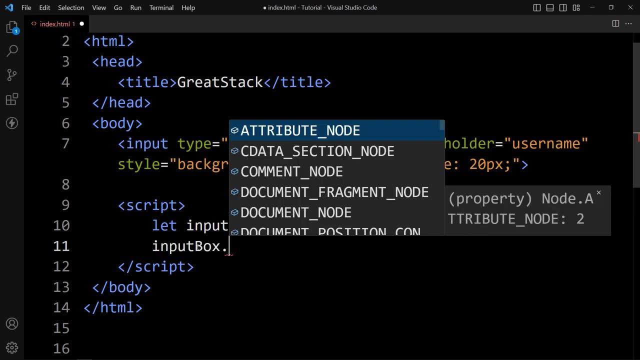 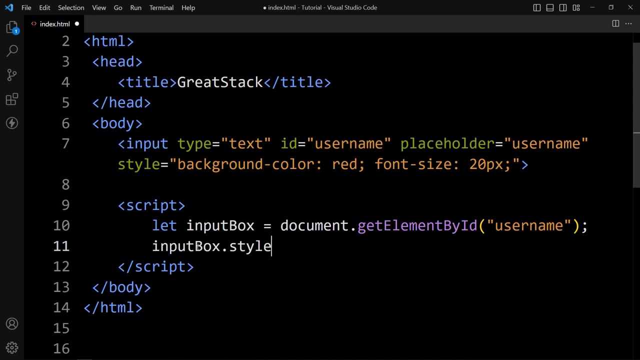 now to get these inline CSS, we can use the style property on this element. so here let's add the element which is input box, dot style, so it will return the CSS properties available in this input field. in the inline CSS it is returning some value, so we can add console, dot log and the 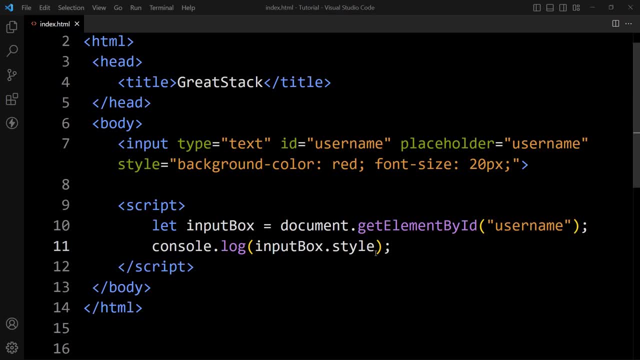 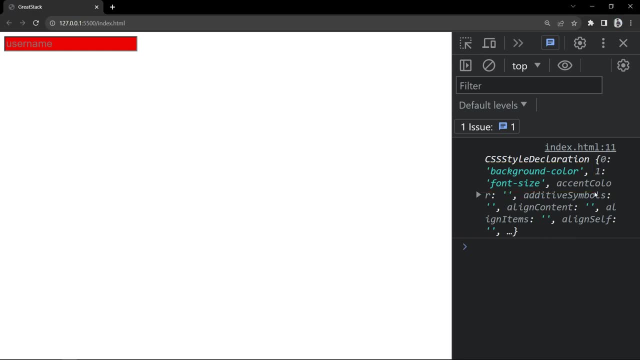 style will return the CSS properties in the inline CSS and we can use this code. now you can see the output in the console tab. in this console you can see it is displaying background color and font size, because here we have only two inline CSS properties, which is background color and font. 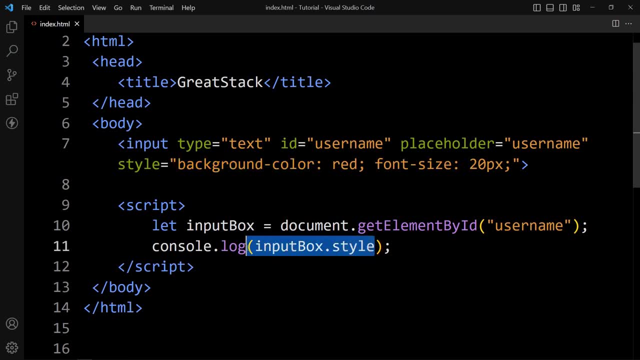 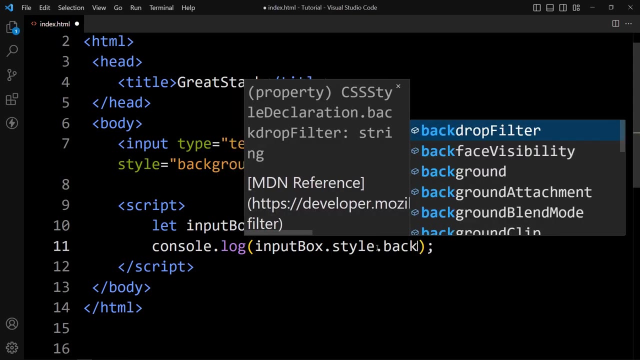 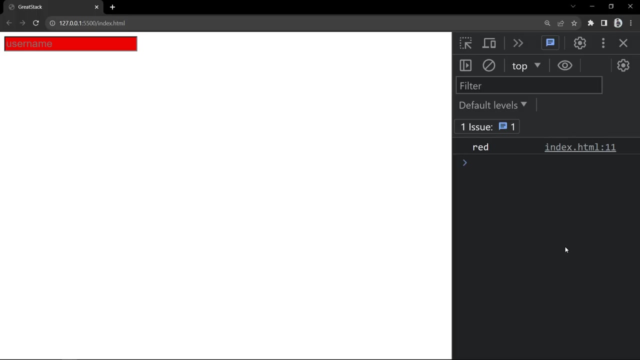 size. so this element dot style will return the inline CSS available in the element. now if you want to return the background color value or the font size value, then we can write input box style- dot background color like this: after adding this, come back to the web page here. you can see it is. 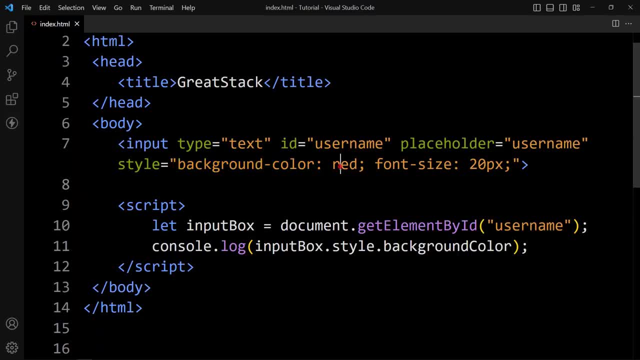 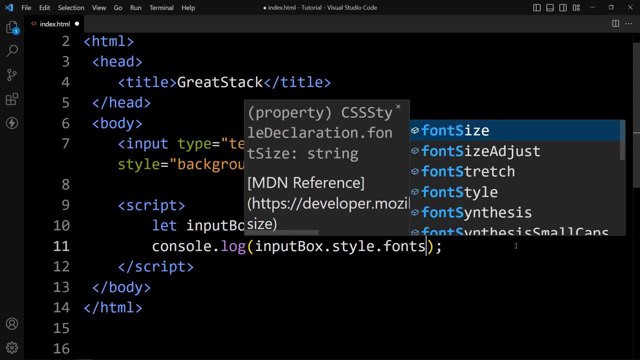 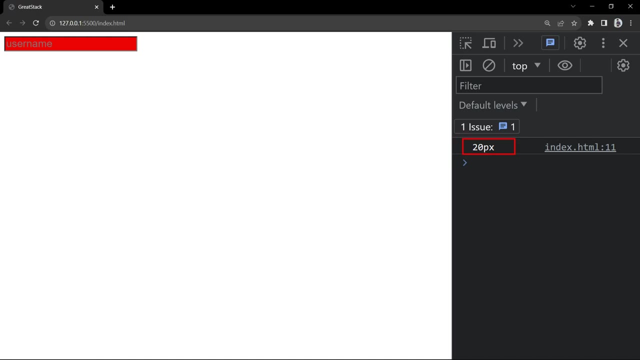 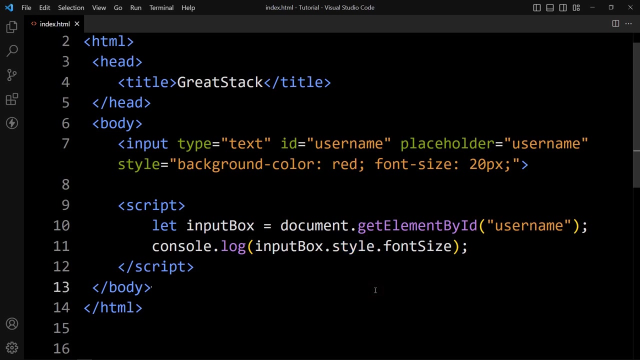 displaying red background. color value is red. now, if you want to see the value of this font size, here we will add font size and you can see the output here in the console tab. it is displaying 20 pixel, so we can get the property name also and value also. now we can use this style property to set the style of the element. so let's add input. 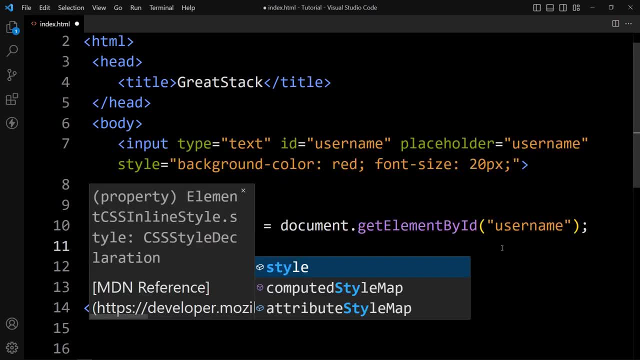 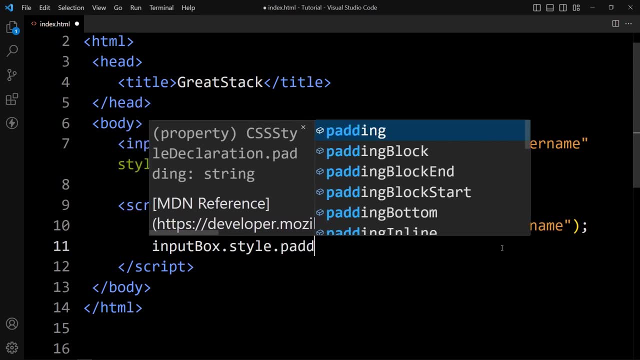 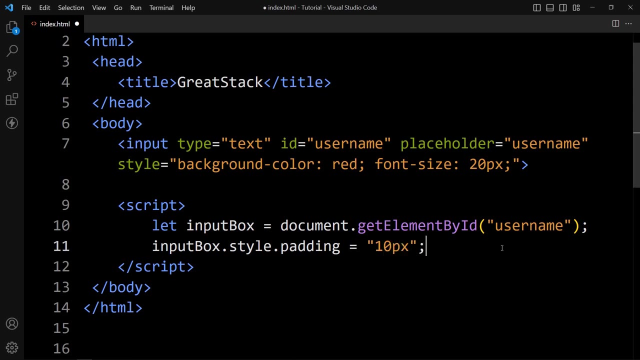 box, and on this input box we will add a style, and in this style, let's add one new CSS property. let's add padding. padding is equal to 10 pixel. after adding this, we will display this input in the console. so we will display this input in the console. so we will display this input in the console. so we 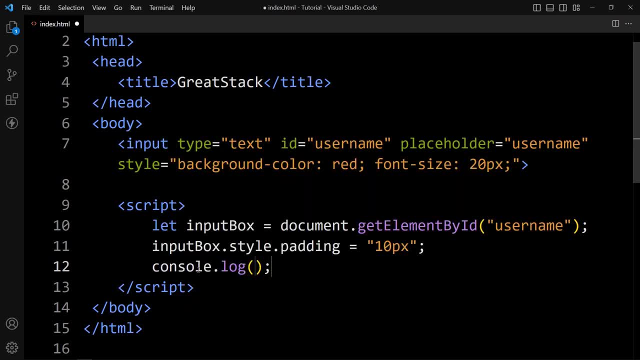 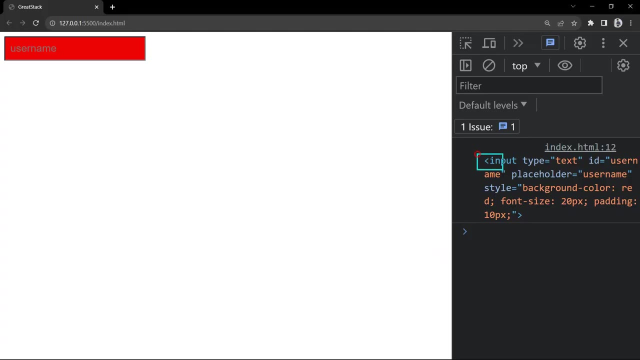 will add consolelog input box, so it will display this input field in the console tab, where it will add the padding also. so let's come back here. you can see we have this input element. in this one we have the style background color, then font size, and after that you can see this padding. let's select. 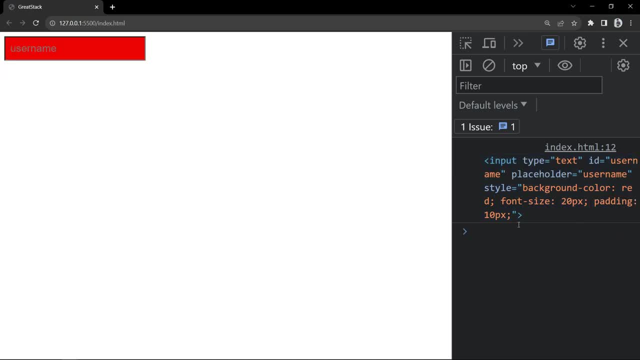 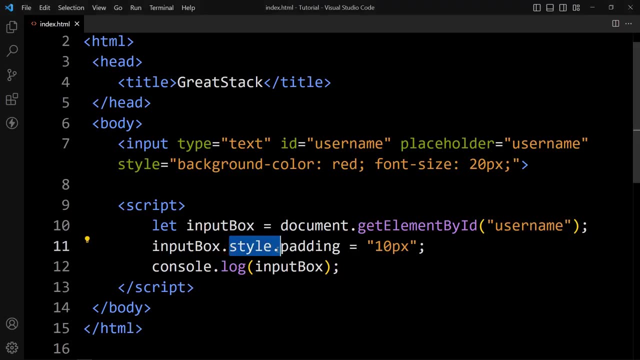 here you can see padding, and the padding value is 10 pixel. so using this style property we can get the inline CSS and we can also set the inline CSS. now we have one more option to add the inline style in the HTML element that is using CSS text. so here we will add the element, then style, then CSS text. 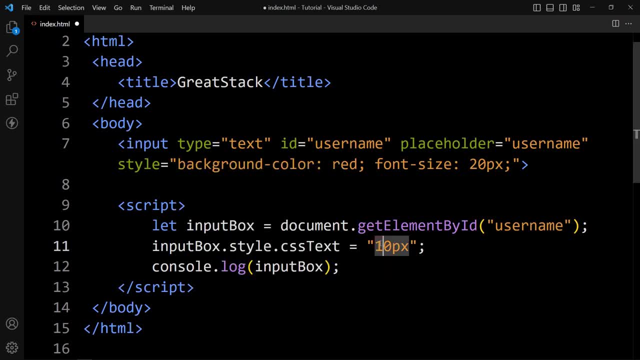 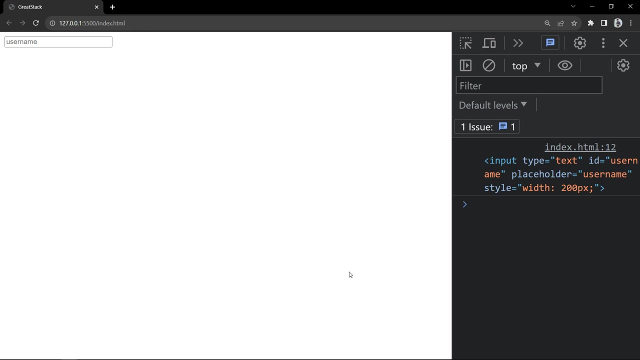 and in this CSS text we can add the CSS. so let's add width: 200 pixel. after adding this, let's print this element in the console. you can see the output here on the webpage. it is displaying this element with the style vector style. so we can add this element in the output here on the web page. it is displaying this. 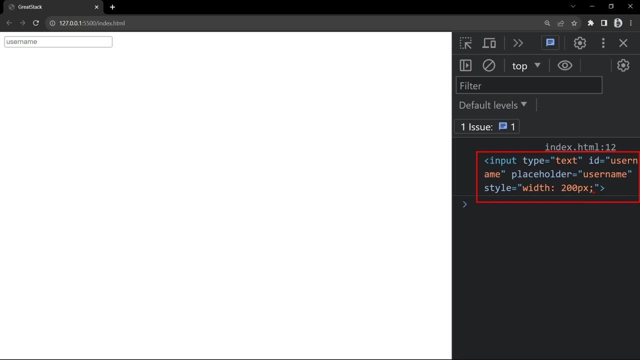 with the style vector element, then style element in the console. you can see this element here on the web page. it is displaying this element to simultaneously permit first name: aku should. are you click 2021.. style width: 200px. here we have only one CSS property, which is width 200px. let's come. 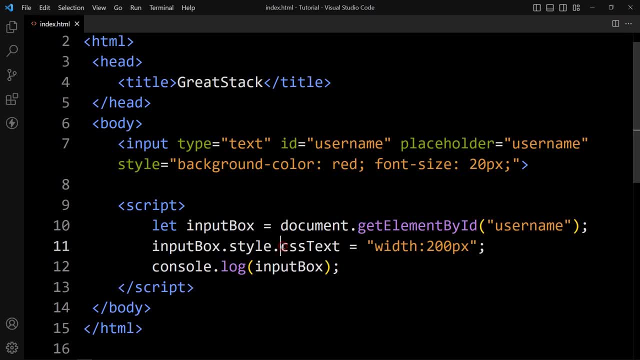 back to the web page. we have added CSS text width 200px, so it will overwrite the existing inline CSS. you can see we already have background color, font size, but it is not available on the web page. why? because we are adding width 200px using this CSS text, so it will. 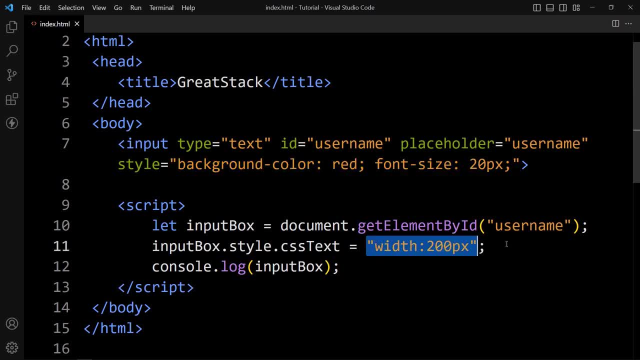 overwrite completely, it will remove this and add this one. but if you want to keep the existing CSS also and add this one also, then you can use the concatenate to perform the concatenate. we will just add plus before this assignment operator like this after: 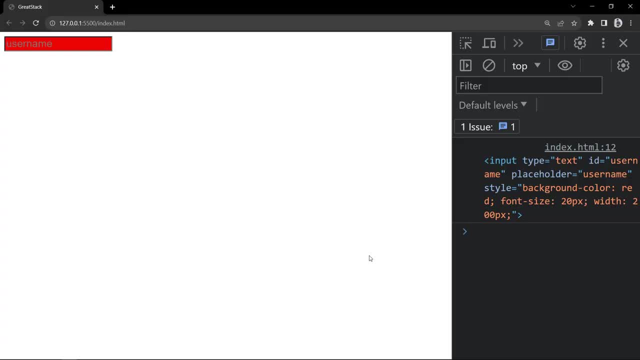 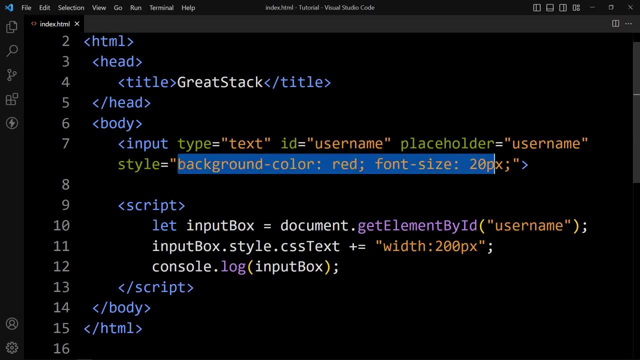 concatenate. we can use the existing inline CSS also and we can add a new inline CSS using this CSS text. we can add multiple CSS properties at the same time. you can see we have added width, so we will add more CSS properties. just add semicolon and add another. 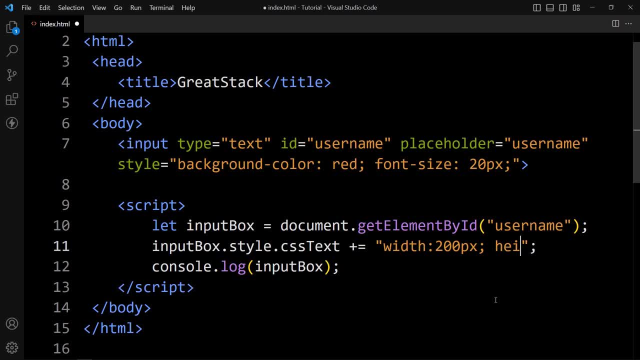 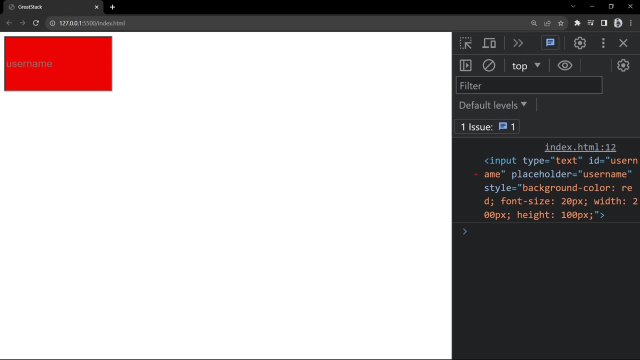 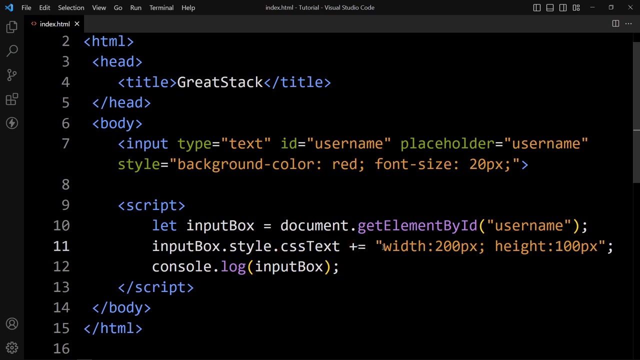 CSS property. Let's add height. height will be 100px. now we will come back to the web page. you can see height is also applied in this input field. you can see it in the console also. here we have height 100px. so using this CSS text, we can add multiple CSS properties in the 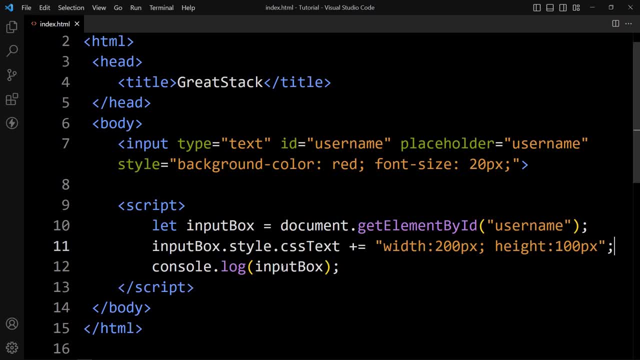 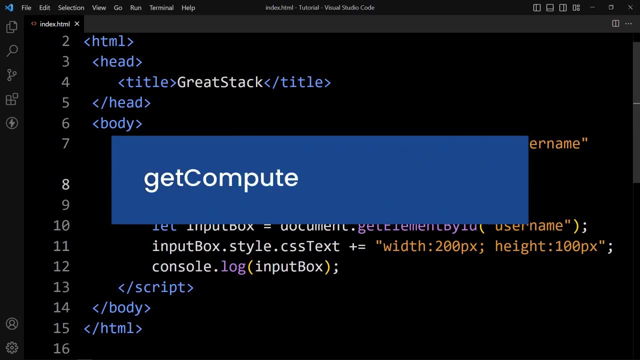 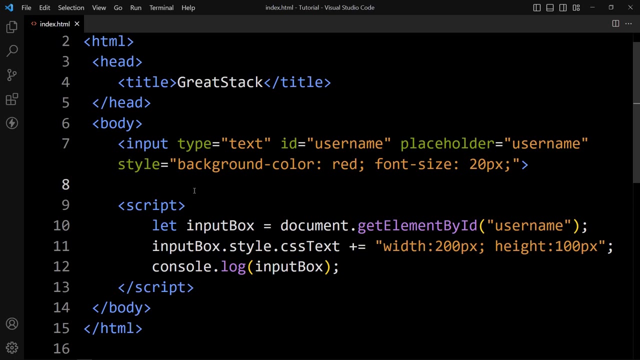 HTML element as an inline CSS. So this was the use of CSS Text for modifying the inline CSS of the HTML element. Now we will learn about getComputedStyle method. currently, we have learned how to modify and get the inline CSS properties of the HTML element using JavaScript. 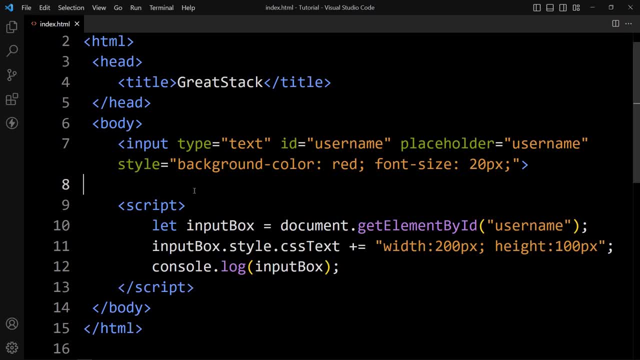 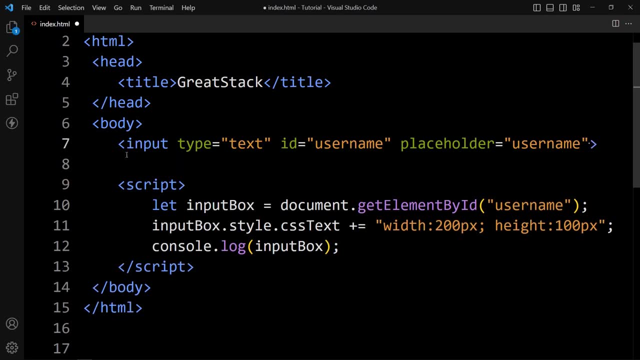 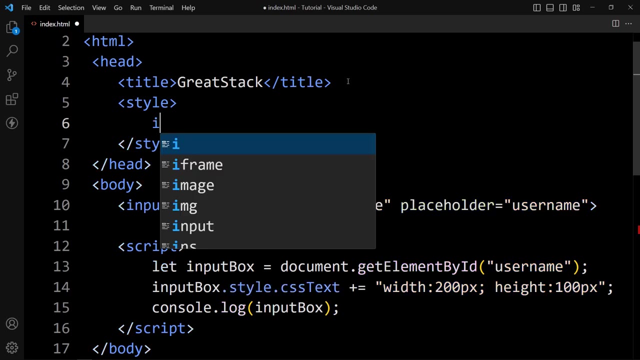 Now how to get the CSS properties written in the external CSS. So let's remove the CSS from here, remove this inline CSS and we will add the CSS properties in this head. Here we will add style tag. within this style we will add the CSS selector input and for. 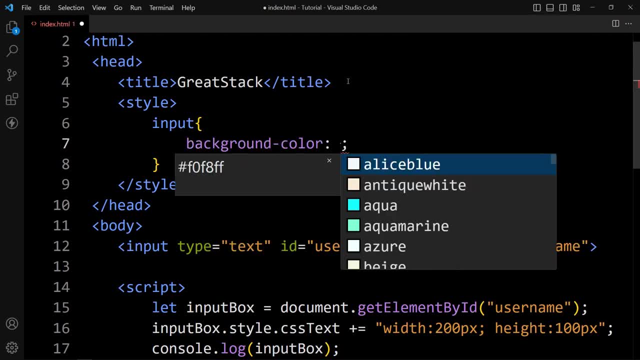 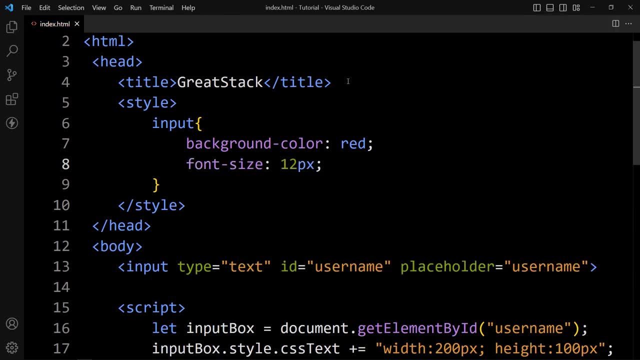 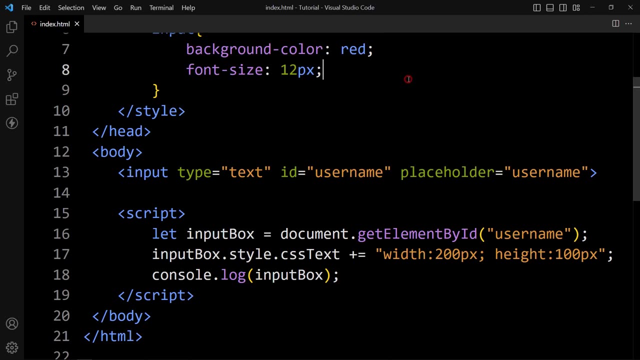 this input, we will add the background. Let's add the background. color: red and font size: 12px. So we have added two CSS properties for this input element. Now how to get these CSS properties? to get the CSS properties of this input element. 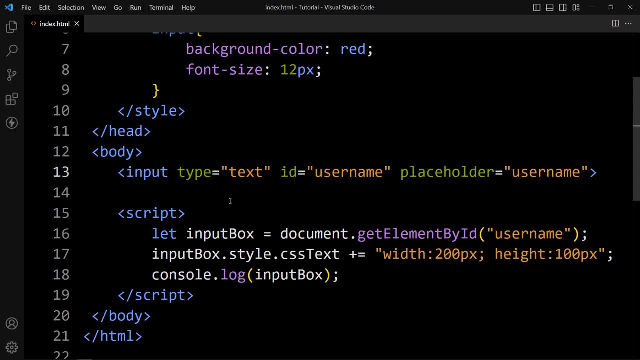 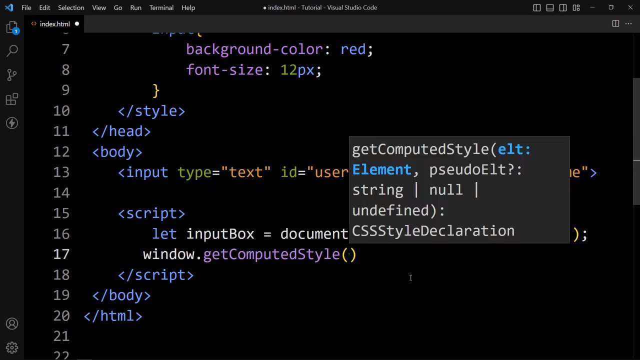 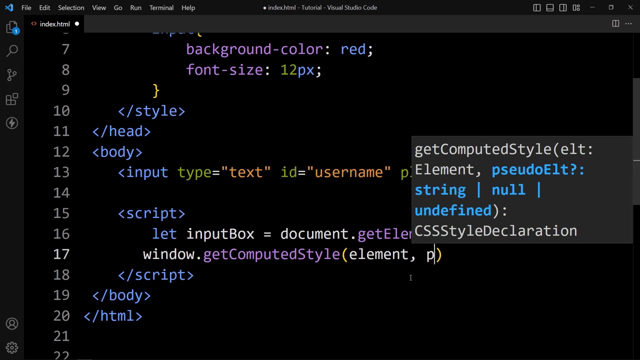 we will use getComputedStyle method. So let's see the syntax first. This getComputedStyle method is a window object, So we will add windowgetComputedStyle and in this one we will add the element. We can add one more argument, that will be sudo element. 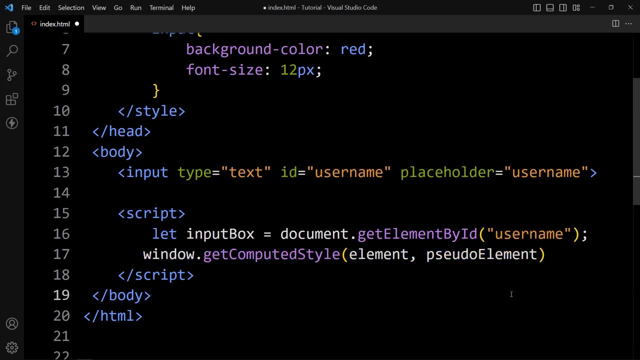 So this is the syntax for getComputedStyle. Ok, In this one we will add the element. if you want to get the CSS property of the element And if you want to get the CSS properties of the sudo element, then you have to add. 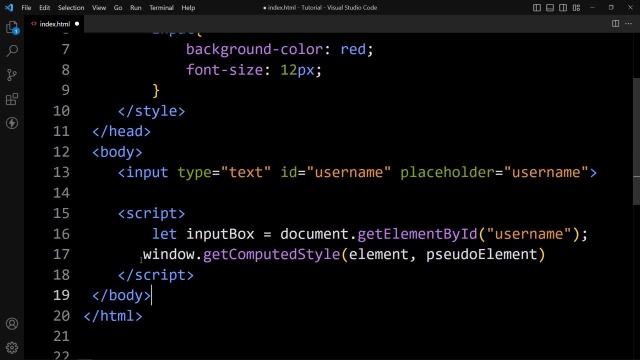 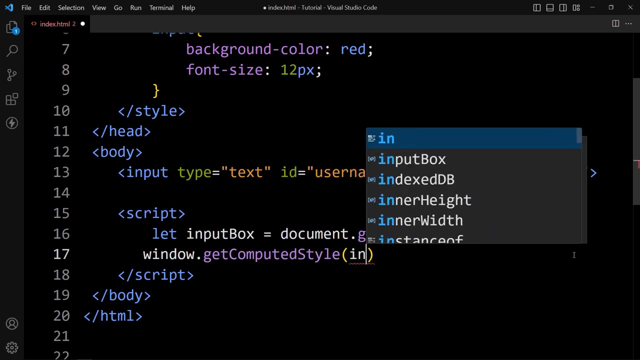 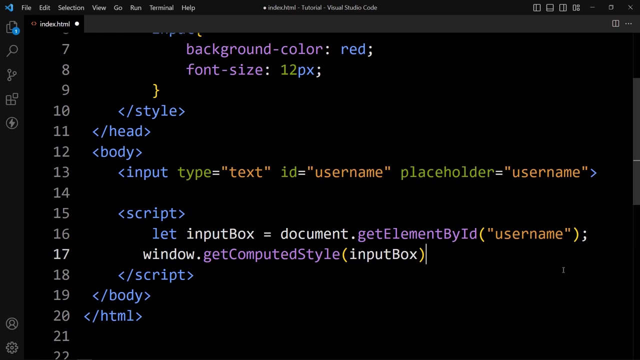 the element and its sudo element. And now let's see the example for this input field. So here we will add windowgetComputedStyle, and in this one we will just pass the element which is inputVox. Now it will return the CSS properties available on this input field, so we can print it using. 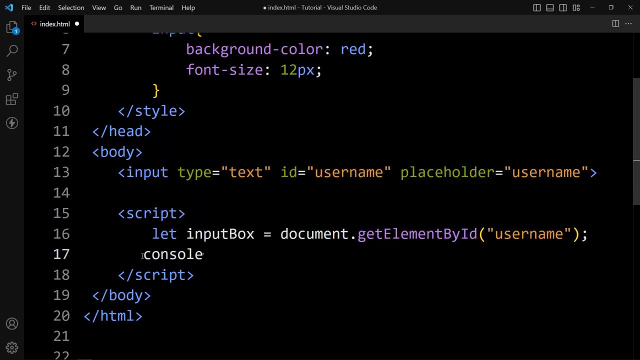 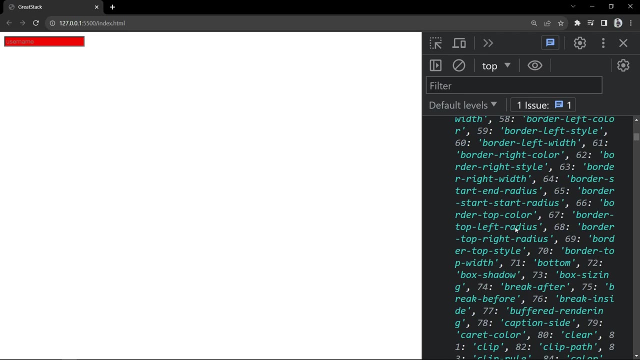 console consolelog and add this one. Now let's come back to the webpage to see the console tab. Here it is displaying all the CSS properties that are applied by default on the element. In this one we will find the background color also. 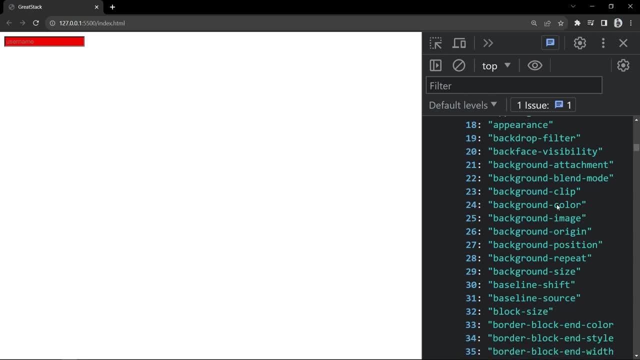 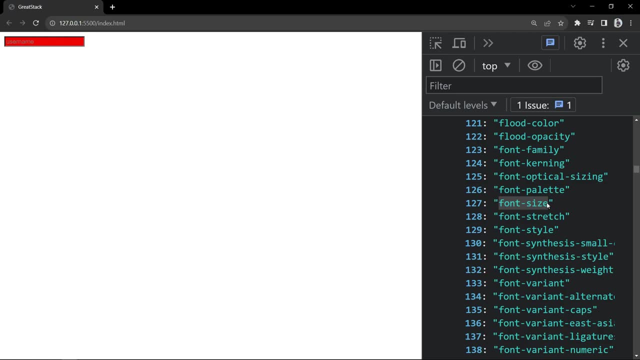 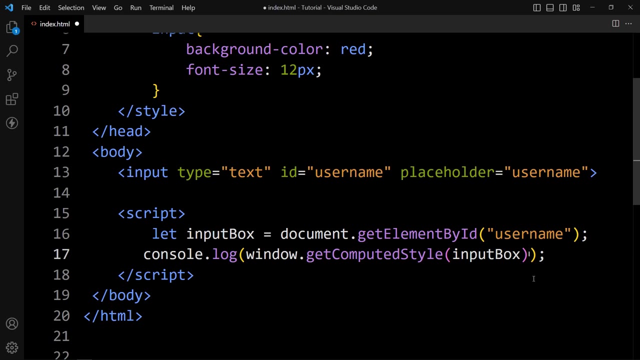 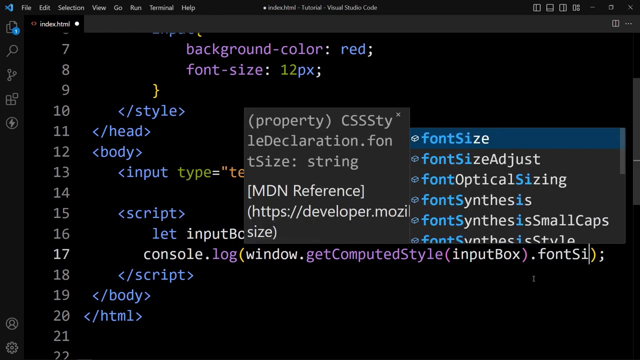 You can see the background color here And there will be font-size also. It is here font-size, So now we can get the value of the particular CSS property. So from this inputVox we will add font-size. Now it will display the value of this font-size. 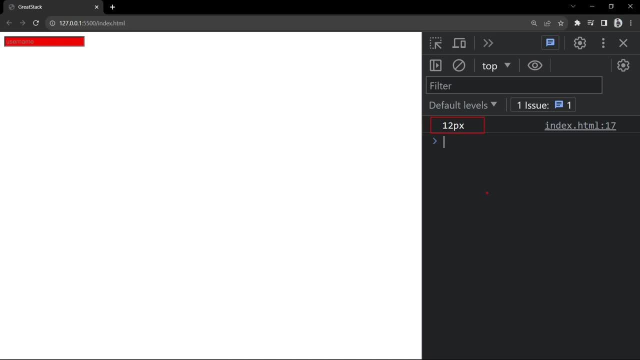 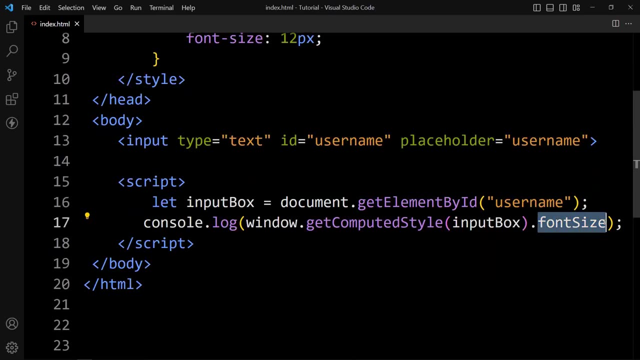 Ok, You can see it is displaying 12px that we have added here in external CSS. Now let's add the background color. We are adding this windowgetComputedStyle, then passing this element, And from this element we will get the value of this background color. 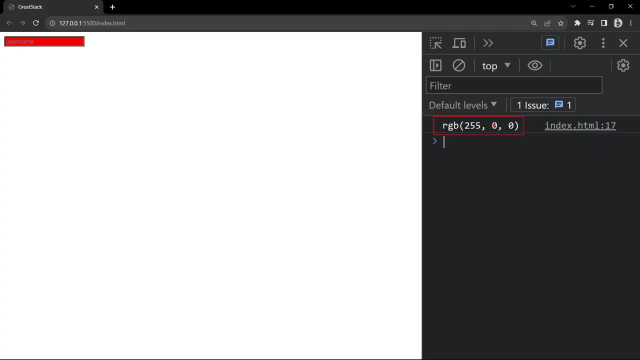 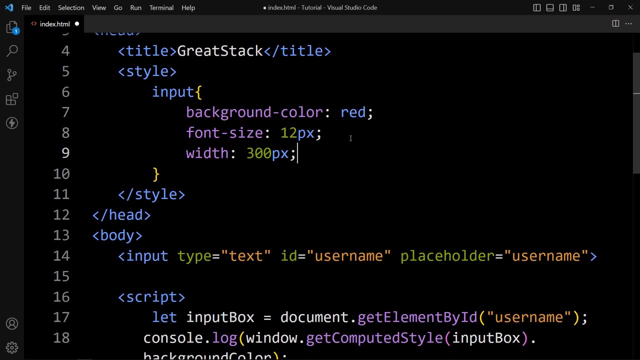 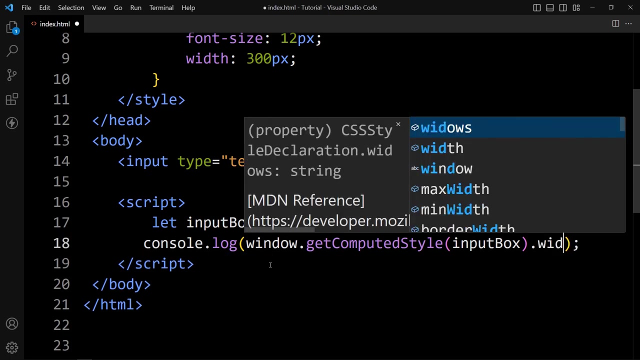 Let's come back to the webpage. Here it is displaying 12px, It is displaying the color. Now let's come back. In this one we will add one more property. Let's add the width of 300px, And here we will add width. 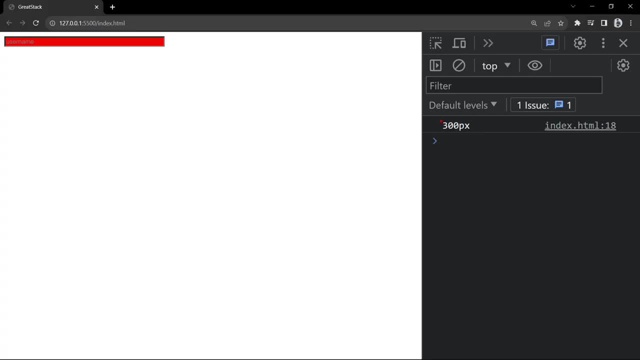 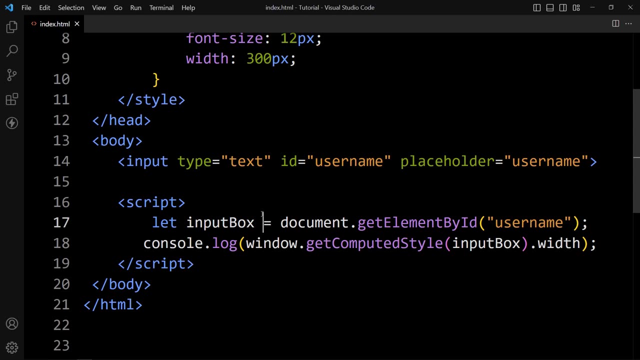 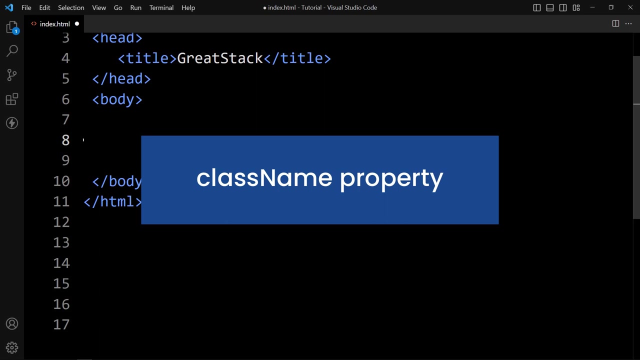 Then we will see the output. It is displaying 300px. So, using the getComputedStyle method, we can read all the CSS properties applied on any HTML element. Now we will learn about className property. ClassName property returns a list of classes separated by a space. 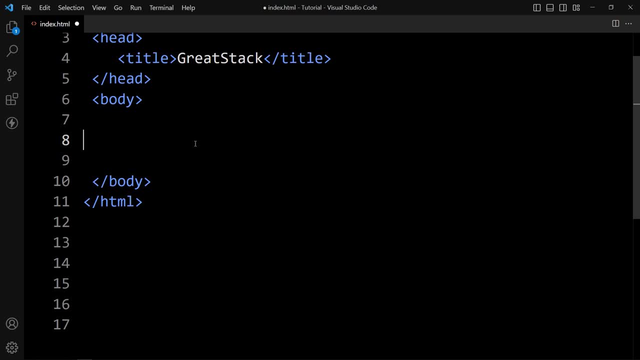 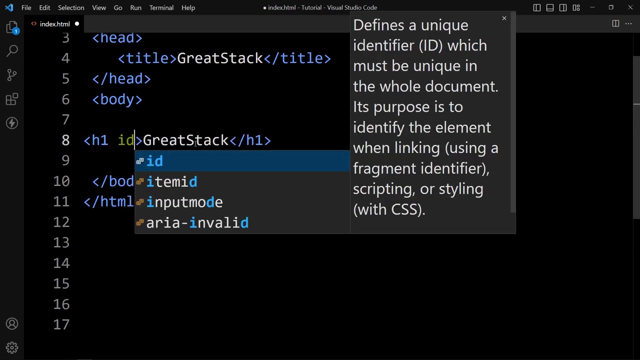 So let's take one example Here: we will add one title in h1 tag. So let's add the text Greatest tag And with this h1, we will add one id To select this. we will add a title: Greatest tag. 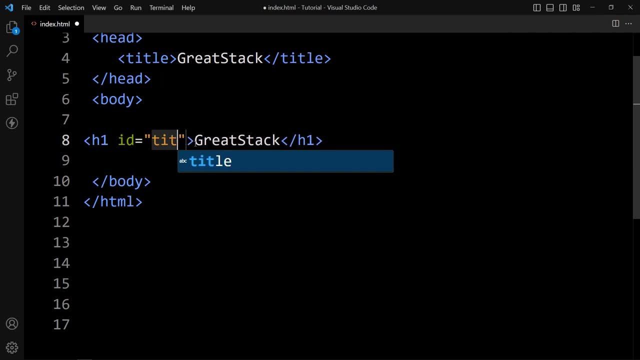 And with this h1, we will add one id To select this. we will add one id To select this. we will add one id, We will add the idtitle And let's add some className also. So let's add the class main, the first className. 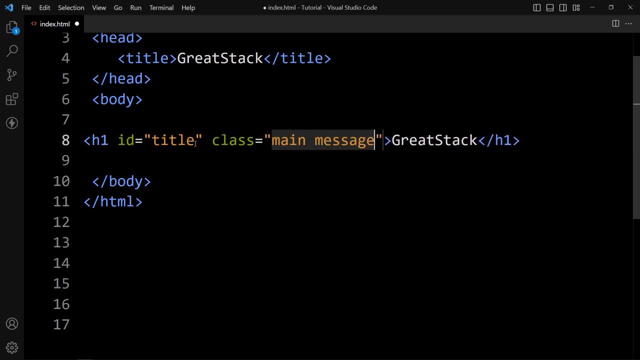 Let's add one more className, which is message. So in this one we have added two classes, which is main and message. Now, to get the className of this element, we will use the className property of JavaScript. So let's add the JavaScript here. 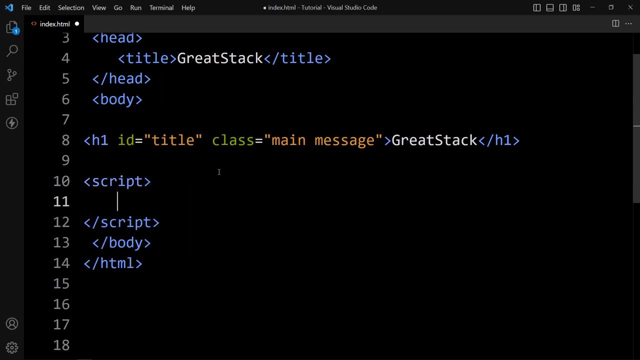 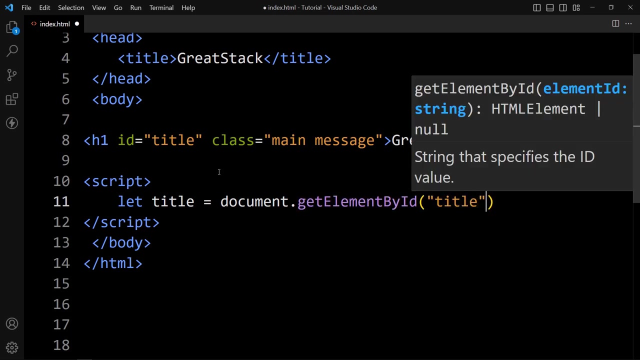 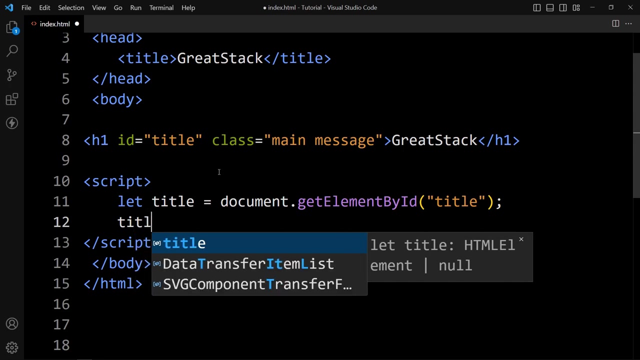 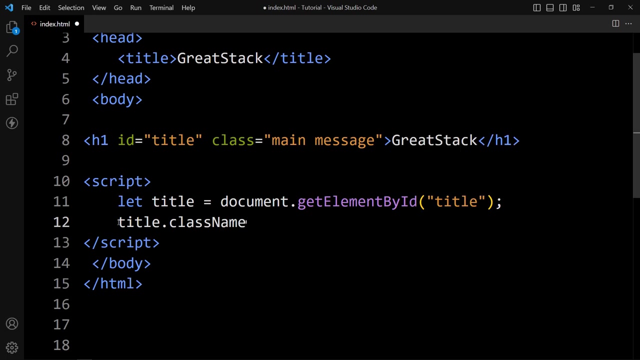 In this script tag type. First we have to select the element. So let's add the variable with the name title and select the element using document dot, get element by ID and write the ID title. After that we will add title, dot, class, name. That's it. It will return the list of classes. 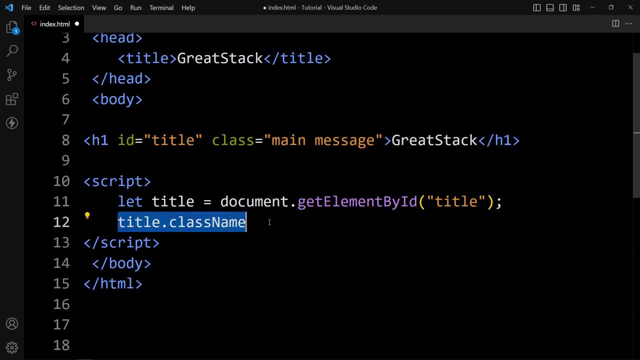 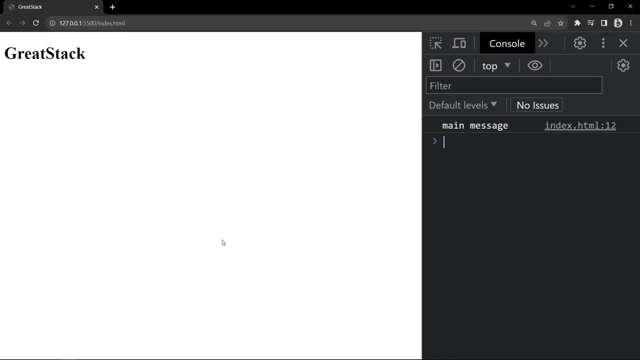 available on this element, So it is returning some value. Then we can print this one in console. Let's add console dot. log title, dot. class name. That's it Now. we will come back to the web page. Now it is displaying the classes available on this element, which is main, and message. 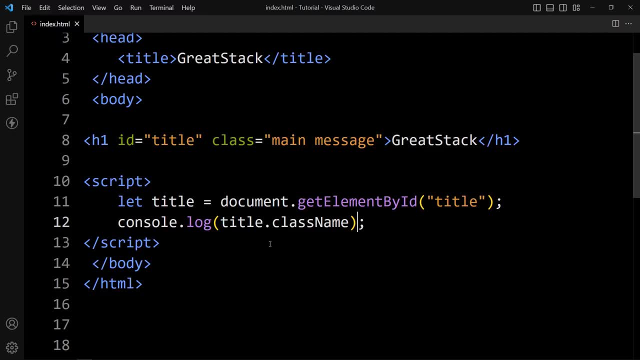 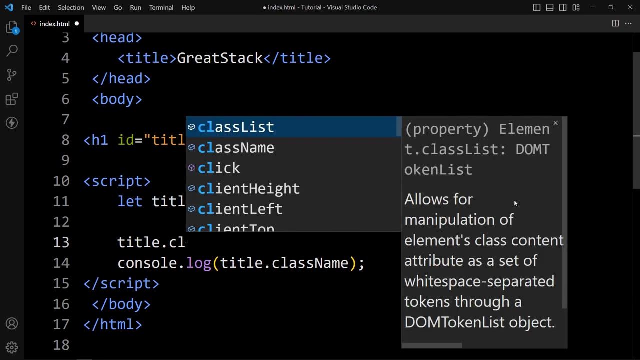 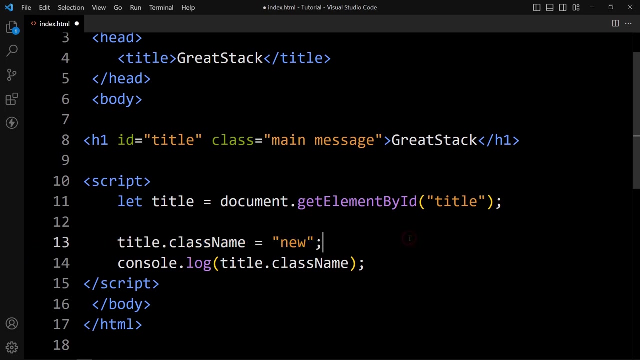 So we have two classes. We can use this class name property to add a new class also. So let's come back here, and here we will add title: dot. class name is equal to new, So this will add one class name which is new in this element. Let's remove this class. 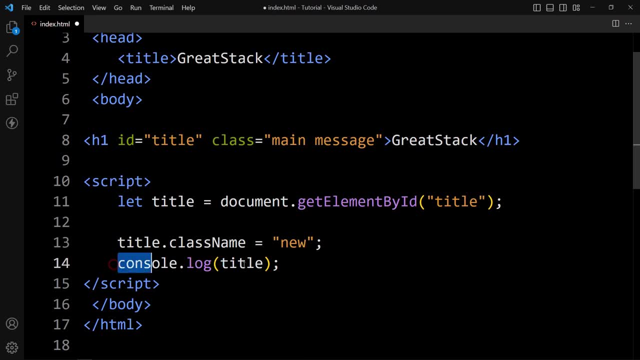 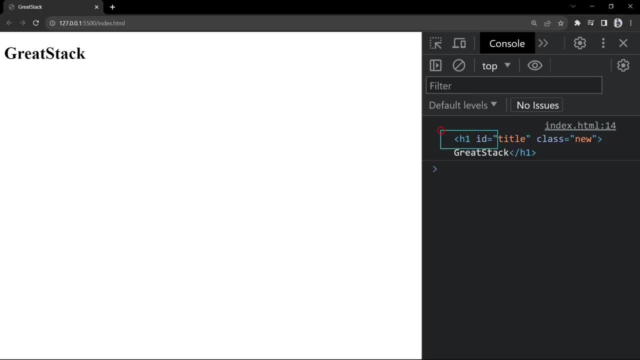 name. here We will display the complete element in the console using this console dot log title. Let's see the element here. You can see it is displaying this HTML element with ID title and class new. We have only one class, which is new, But in this HTML you can see. 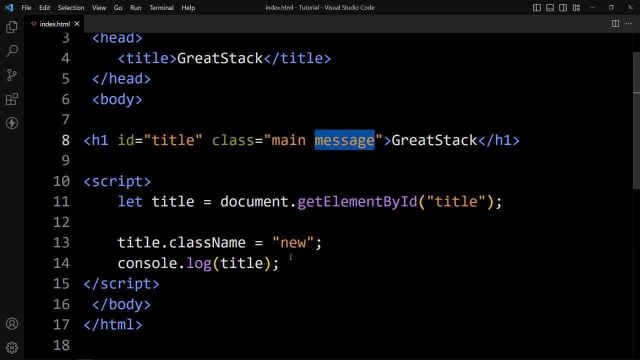 we have already added main and message, So this will override these classes. Here we have two classes that will be removed and this new will be added in this class. But if you want to keep the existing class also and new one also, then you can use the concatenate using this plus and this assignment operator. 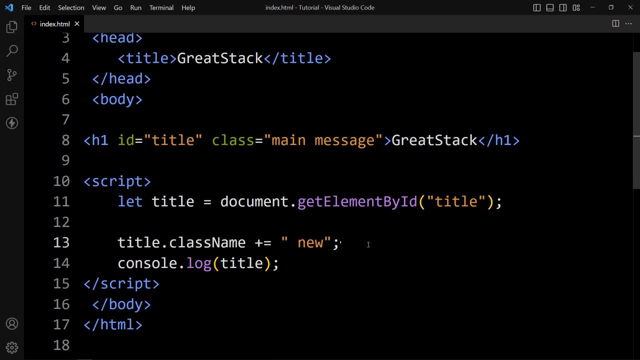 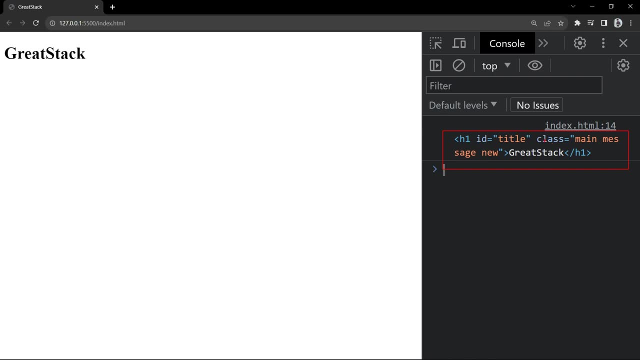 After adding this here, we will add a space. and let's come back to the web page. Now you can see the same element H1 here And in this element we have class main message and new. So we have total three classes here. 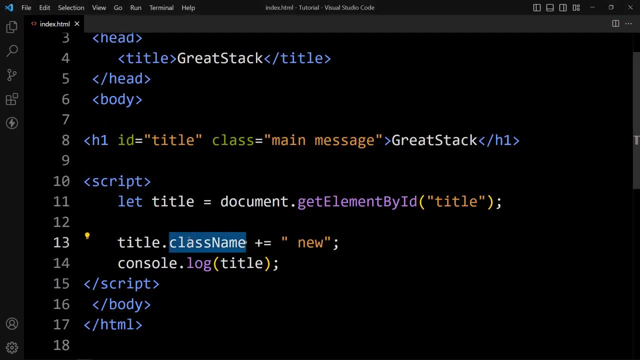 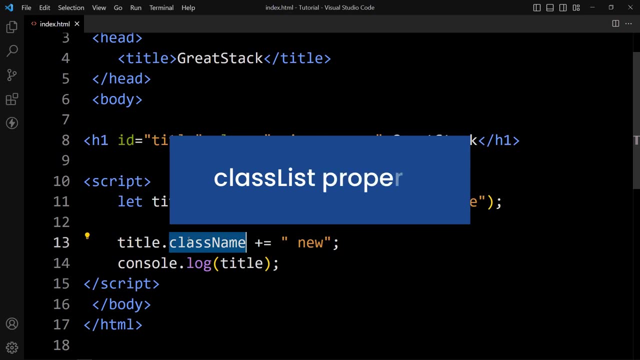 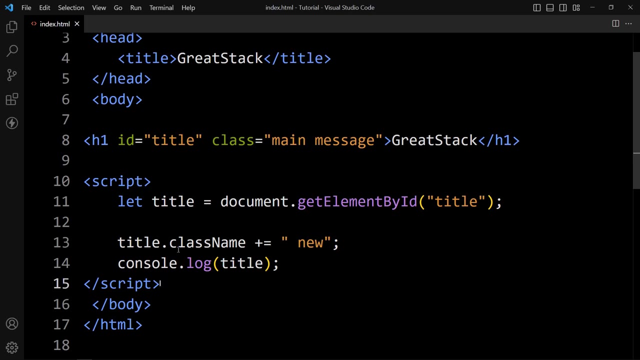 So, using this class name, we can read the class name of the HTML element and we can add a new class also. Now we will learn about class list property. Class list returns the collection of CSS classes. So let's see if we add class list property. 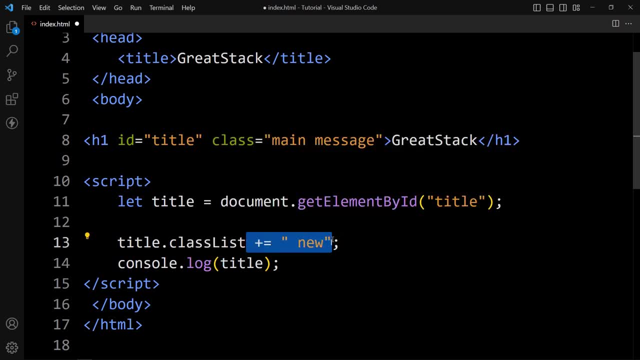 Let's see. So we have a class list and it is returning some value, So we will print this one titleclasslist like this: We are just adding titleclasslist and you can see we already have main and message class in this element. Now we will come back to the web page. In this one, you can see: 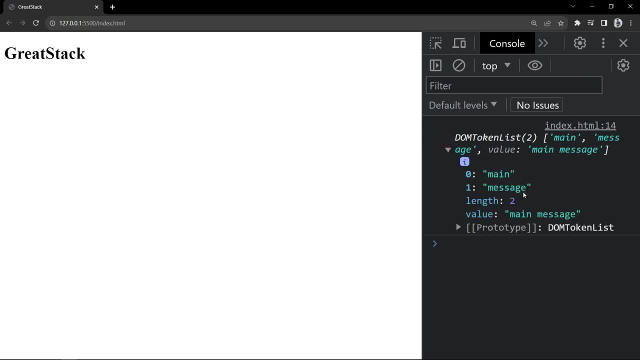 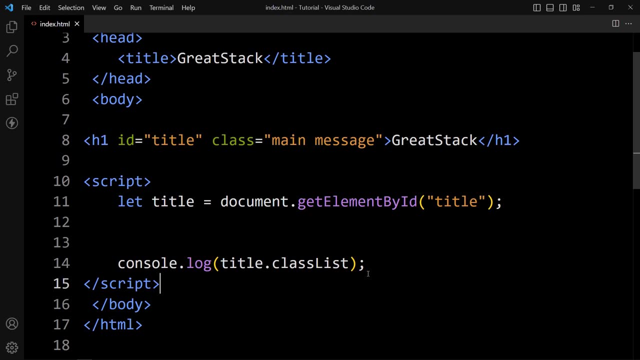 we have a list where we have main and message class, So we have two classes. So this class list is returning the collection of classes available in this element. Wait, let's click on the change now. In this article we have added just one class on it. the class name of this element, Let's. 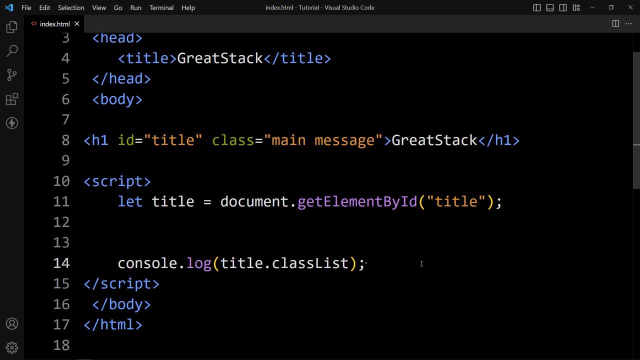 see if we can add this one too. So based on this we are going to define only to a class needs. It says important class list. Let's consider a class in the table. We can reject our pack strategy of a class, but when we add another class on the first, 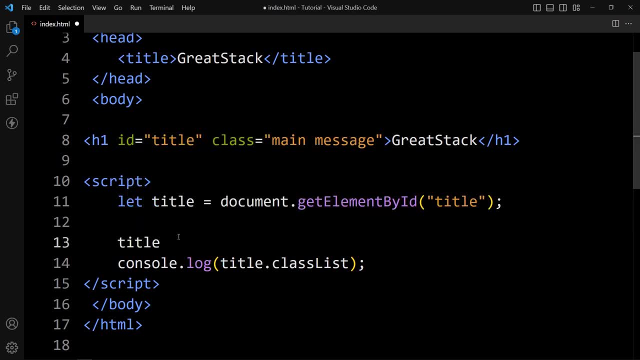 class. we cannot add another class Just like a line. We can also add umpolize text to. let's try to add a tickile hate tournament. What will happen? This is going to change class list, dot add, and in this one we can add a new class. just add new, like this. that's it. 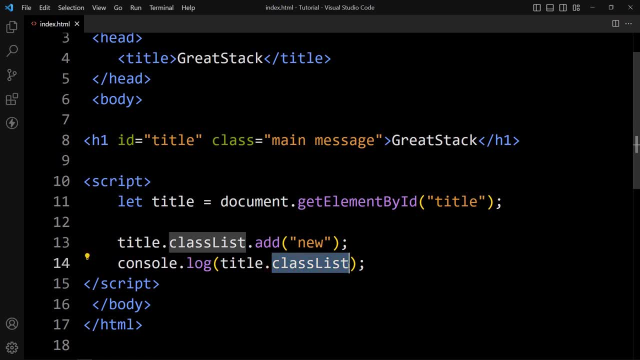 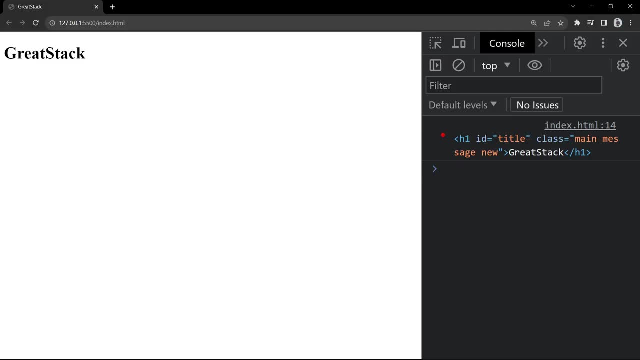 after adding this, we will display this complete element in console tab. we are displaying this title. let's come back to the web page. here you can see we have this element with three classes: main, then message, then new. let's change the size so you can see we have total three classes. 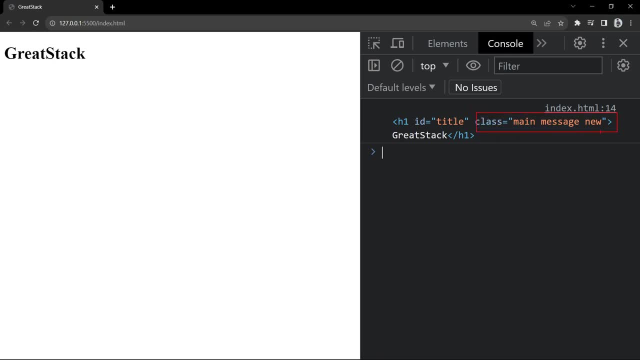 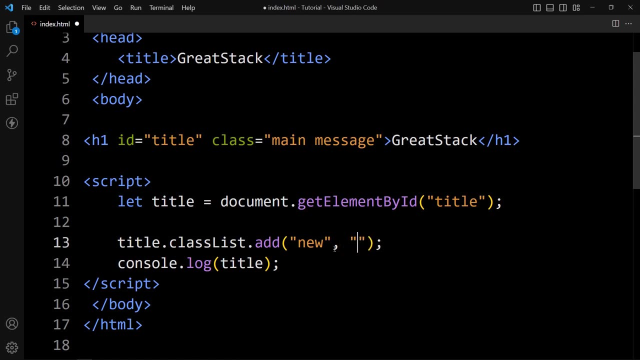 main message and new. now let's come back. if i add multiple classes, we will just add a comma and add a new class name like new to. so we are adding another class name. like this, we can add multiple classes using this class name. like this, we can add multiple classes using this: 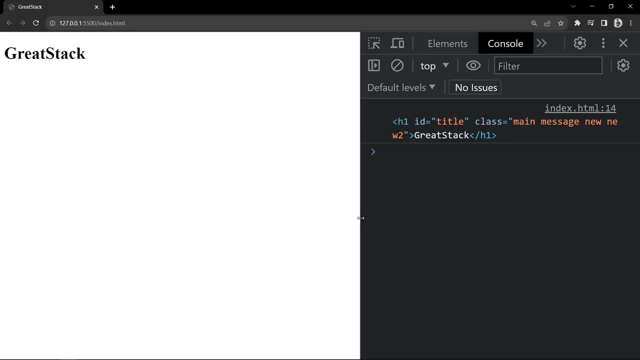 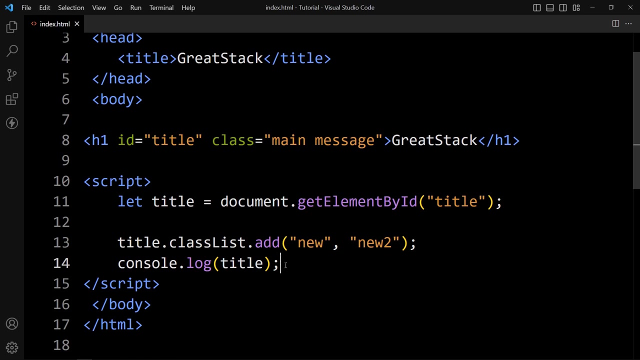 class list. you can see we have more class name here. main message: new and new to. so using this class list dot add, we can add a new class name in the html element. now we can use this class list to remove any class. so instead of this add, just type. 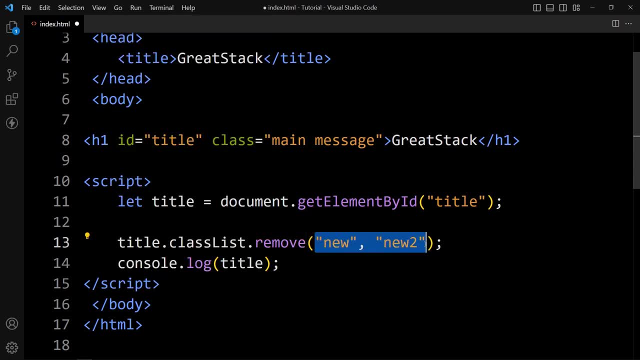 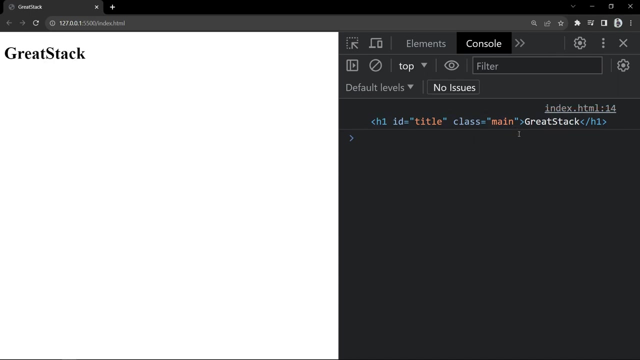 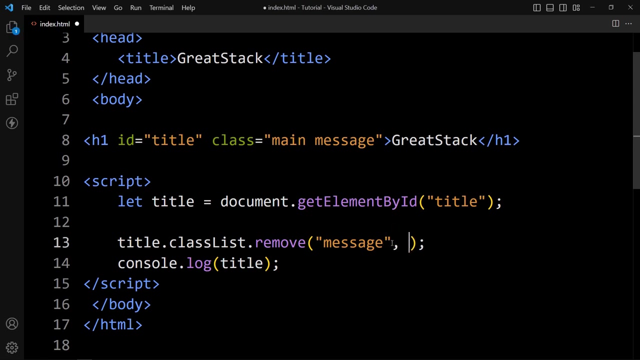 remove class list, dot. remove and and what we will remove. we already have main and message, so let's remove this message, write it here in a quote and come back to the web page. here you can see in this element we only have one class, which is main. now just come back and we can remove both classes, so let's add comma and write. 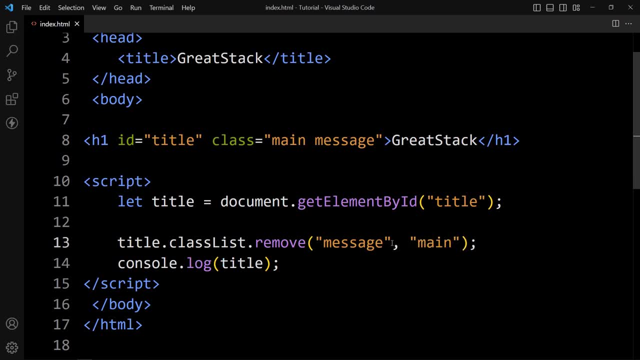 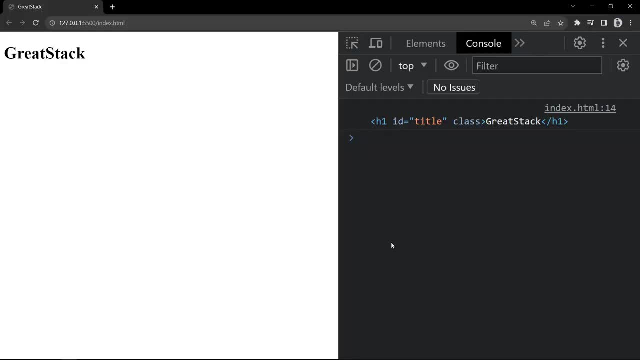 main, so it will remove the another class. also, we can type multiple class name here and it will remove all that classes from that element. you can see this element. in this element we don't have any class. we have the class attribute name here, but we don't have any value in this class. 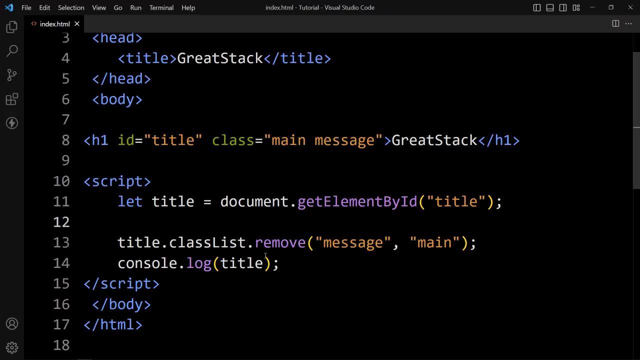 next, we can use this class list to replace any class. so instead of this remove, we will add replace. and to replace this one we have to add the existing class name and new class name. so in this html element we have message, so write message here and we are adding a new class name. 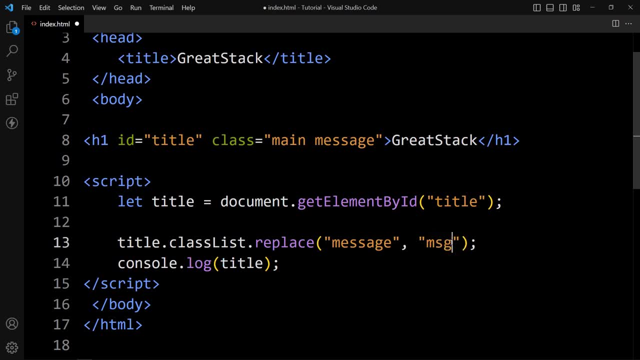 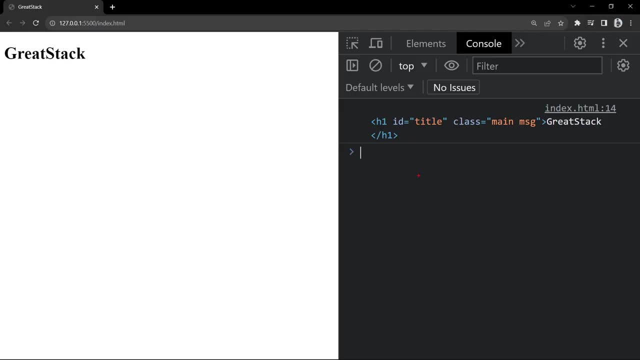 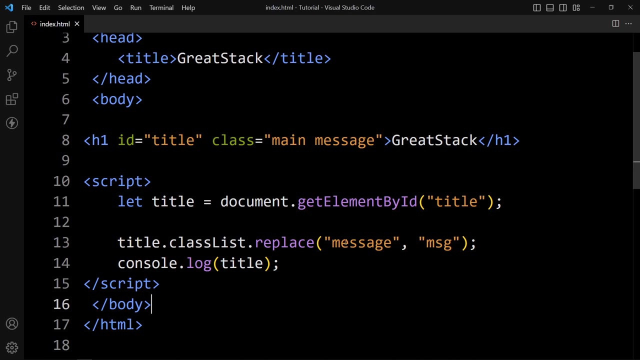 instead of this message. so we'll add msg. so instead of this message, we will replace it with msg. now just come back to the web page. you can see the output in console. here we have class name, main and msg, so we are replacing this message class with msg class. 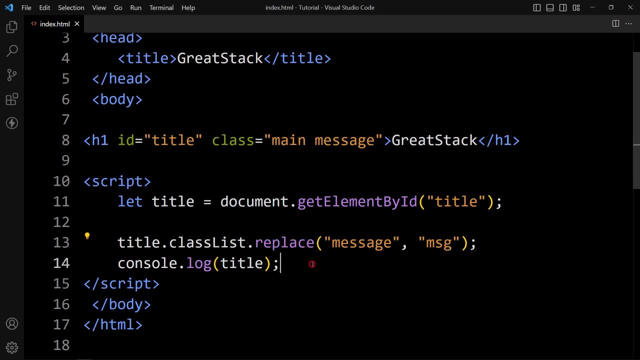 using this class list dot replace. now we have one more option to check whether the class is available or not. for that here we will add class list dot contains, and in this one we'll add any class name. so this message is here. we are adding message, so this will return the value either true or false. if this message is available in this element, then 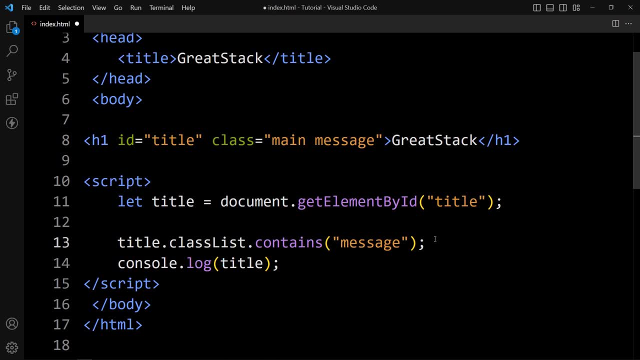 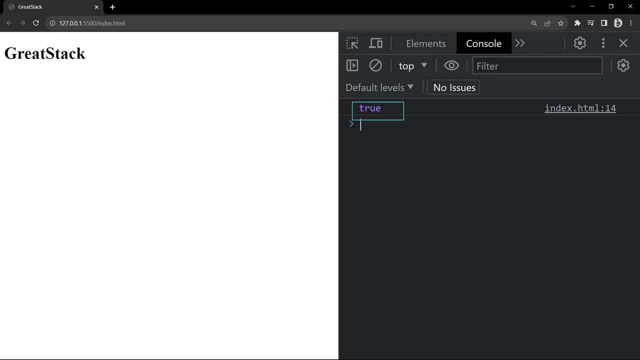 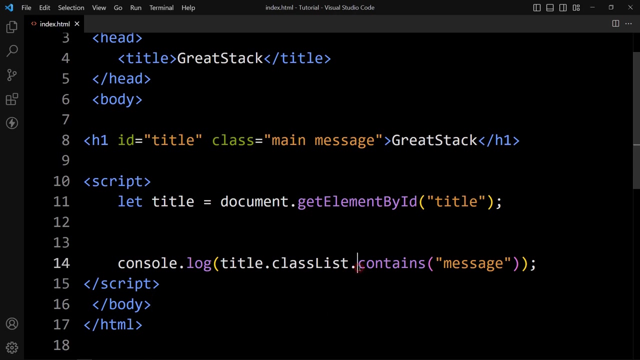 it will return true. if it is not available, it will return false. so we will just print this one, remove it from here, add it in console and come back to the web page. you can see it is printing true because this message class is available in this element, so we are adding classlist dot contains. 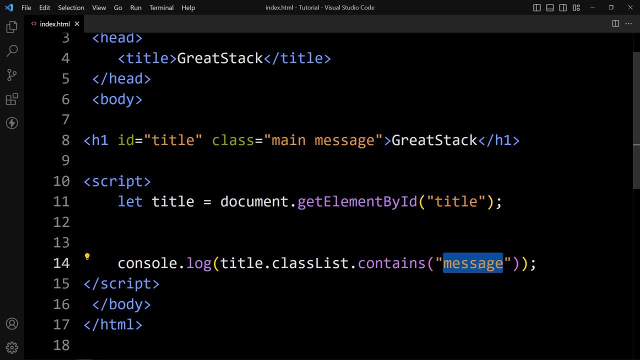 and class name. this class name is available in the element. that's why it is returning true. suppose we add msg and this msg is not available in this element, then it should return false. you can see the output: it is false. now we have one more thing, which is toggle. let's see this example here. we will remove this one. 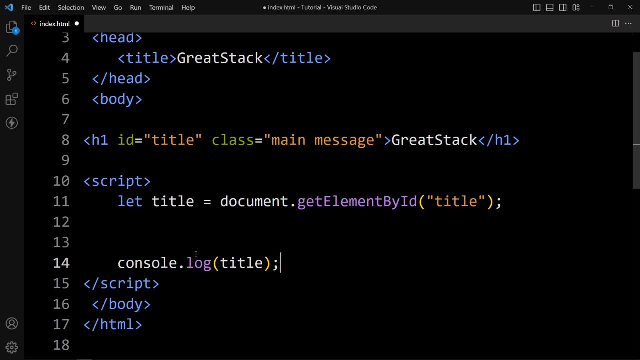 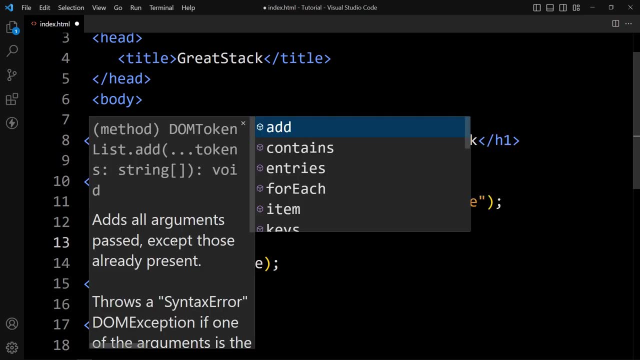 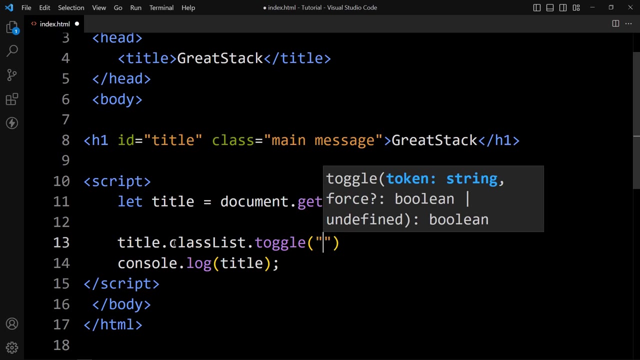 we will just print this complete element in console and here let's add title dot. class list dot toggle, and in this toggle we can add any class name. suppose we add message. what will happen if this message class is available in the element, it will remove it. this toggle means if the class name is available it will remove it, and if it 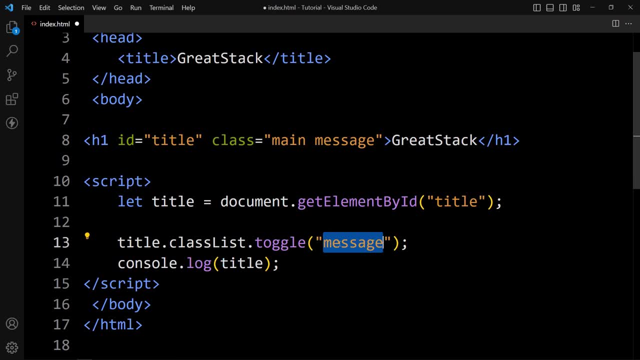 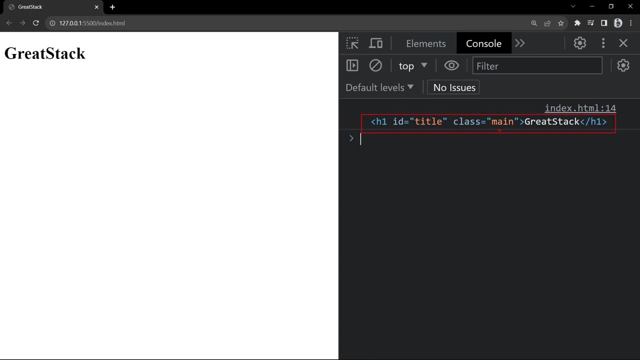 is not available, then it will add that class name in the element. so what will be the output? this message is already there and we are adding toggle message, so it will remove this message. let's see the output in console. here you can see class main. here we have only one class, which is main, so this toggle remove this. 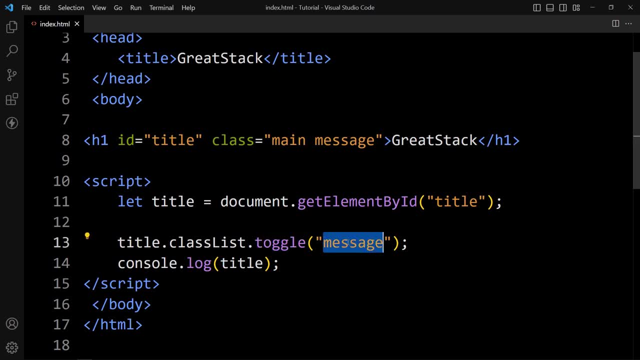 message: class now. instead of this message, we will add new. so what will happen? this new is not available here, so it will add this new in this element. let's come back to the web page again and now you can see we have total three class in this element. 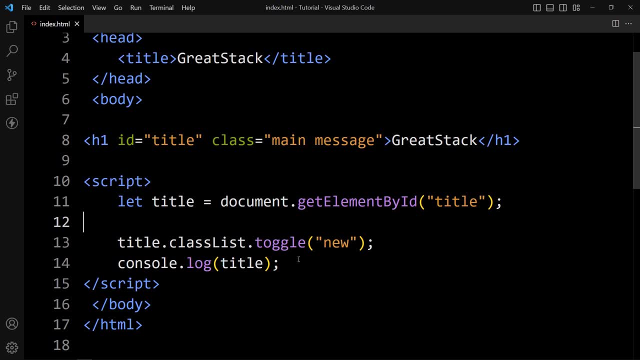 which is main message and new. so using this class list dot toggle, we can add and remove the class from the element. if the class name is already there, it will remove it, and if it is not there, it will add the class. so this was all about class list property in javascript. now we will learn. 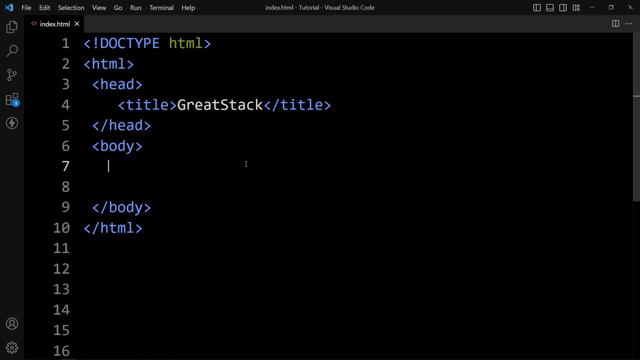 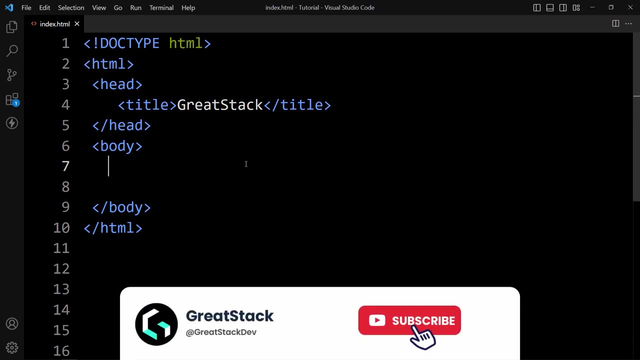 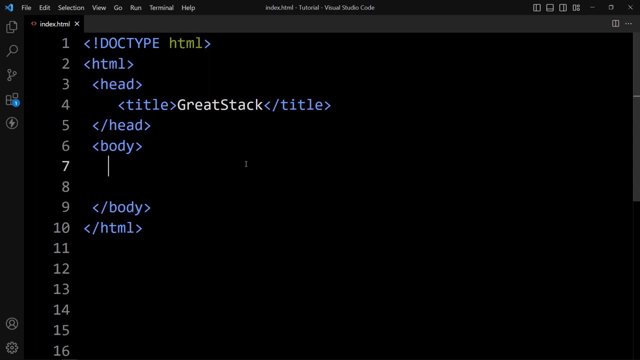 about javascript events. an event is an action that occurs in the web browser. when we click on the web page, that is a click event. when we move cursor over the web page, that is mouse move event. and when the web page loads, that is a load event. like that. we have multiple type of events in javascript. let's say we have a. 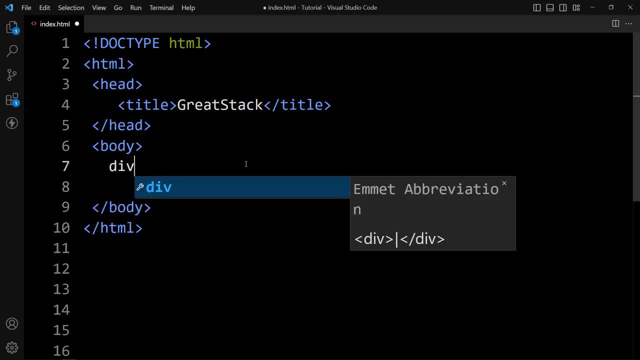 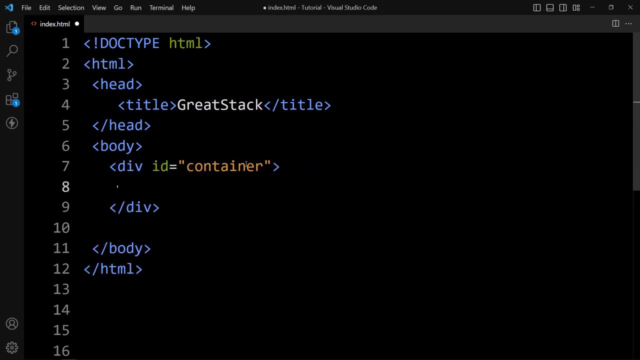 box event. it can be a task. if not a task, it can passes in a normal application. if not, we can collect it in a wondered way- and here we will find a topic called palavra house- and then we can include it in the points list function. let's start our project and see what. 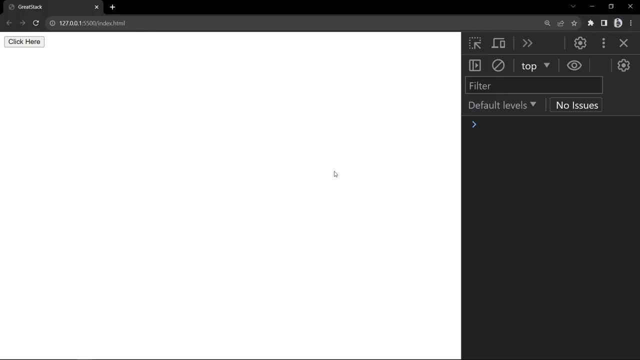 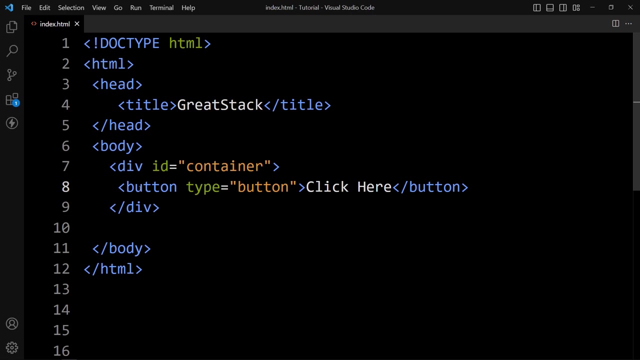 events do we see here? you can see this button: click here. if i click here, nothing is happening because we have not added anything. so let's come back. you can see we have added the button and clicked on this button. but when we click on this button, we are actually clicking on the button. this. 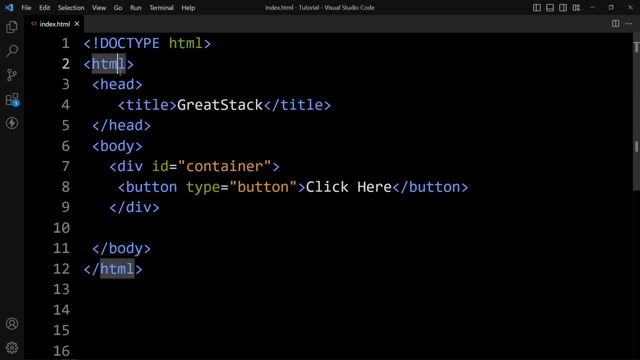 div, this body and this html and this document also. so when we click on any element, actually we are clicking on the all the patent elements also. that means this div with the id container, then body, then html and this document, and in modern browser this click goes up to window object. 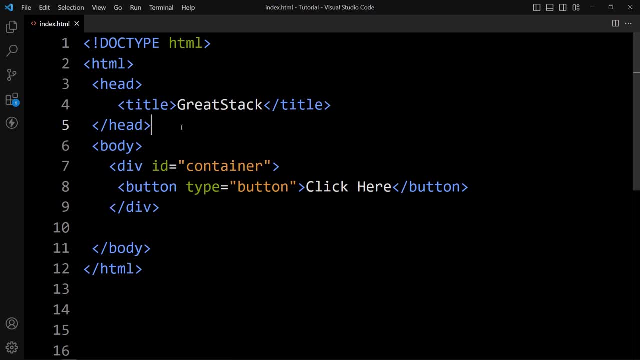 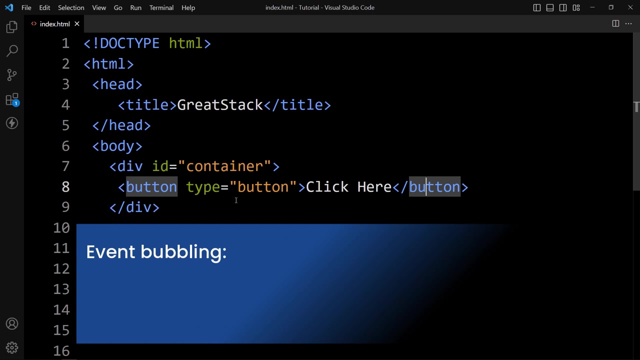 there are two event models, that is, event bubbling and event capturing. so when we click on the button, click a start from the button, then goes to div, then goes to body, then goes to html and then goes to document. so the event flows from the most specific element to the least specific element. that 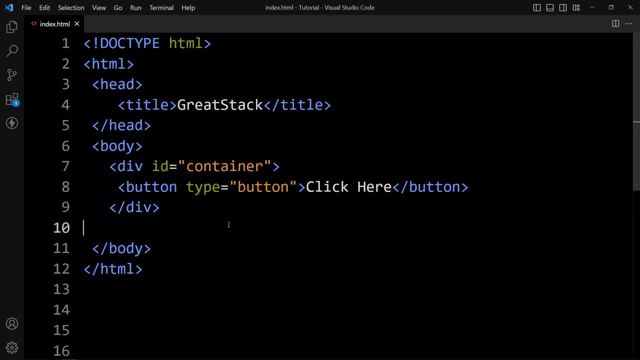 is event bubbling. but when the event start from the least specific element, it means it starts from the document, then event flow to html, then it flows to body, then it flows to div with the id container, then it comes to the target element, which is button. so this: 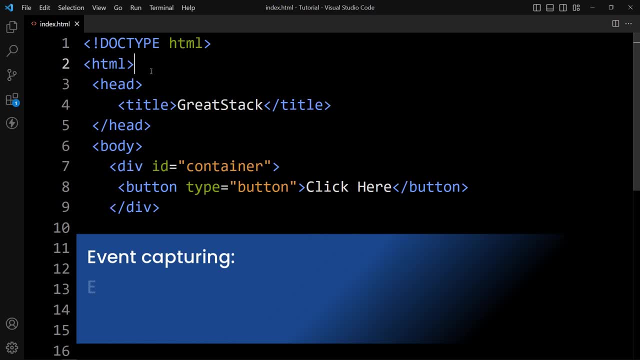 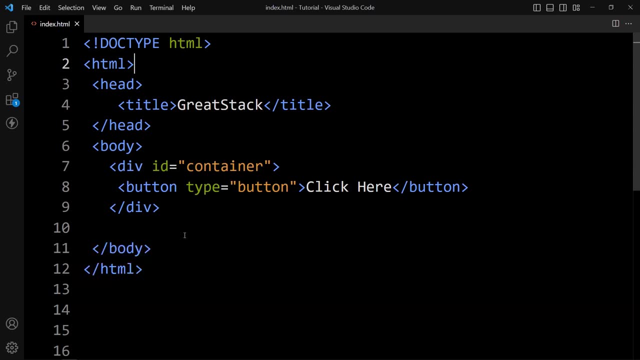 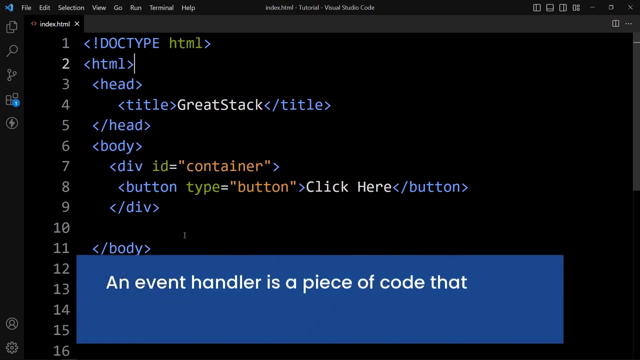 This event model is known as event capturing. when the event starts at the least specific element and flows towards the most specific element, We may respond to these events by creating event handlers. An event handler is a piece of code that will be executed when the event occurs. 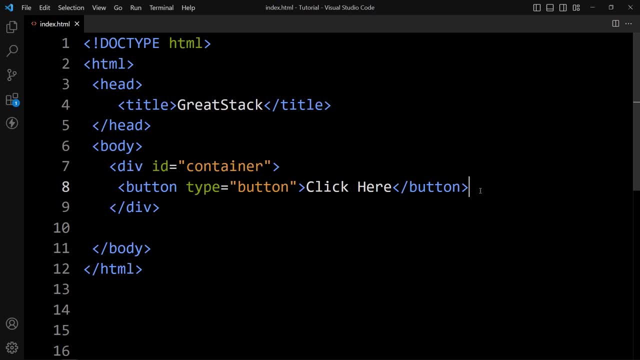 So when we click on this button, we will add some code that will be executed after clicking on this button, So that code is known as event handler and event handler is also known as event listener. So there are three ways to assign event handlers. 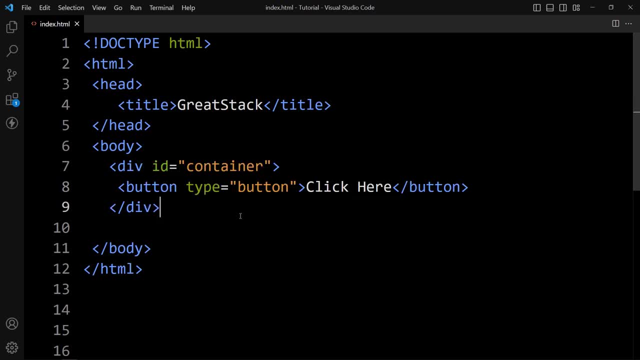 So first one is using HTML attribute. For each event there is event handler and their name typically begins with on. So let's see the example: We have click event and for this click event we have the event handler on click, Like this: 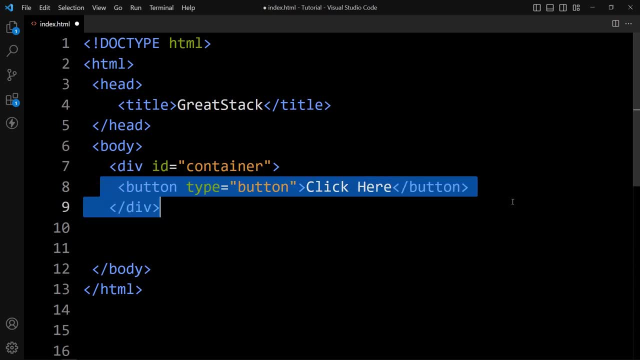 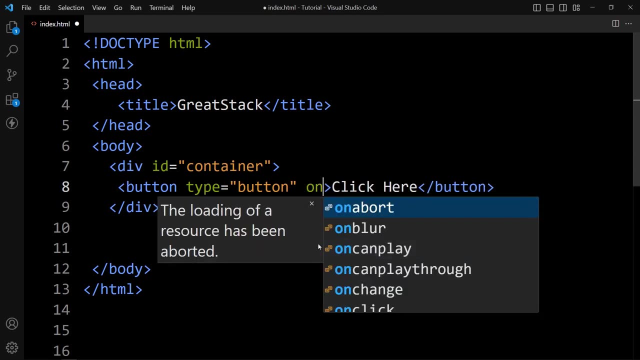 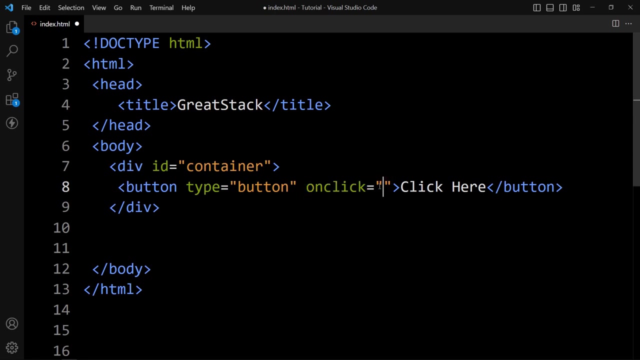 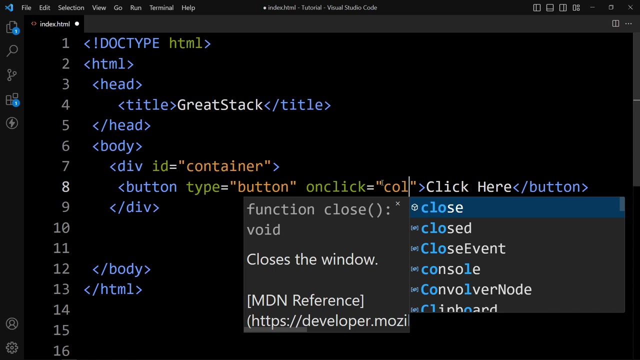 So let's assign this on click in this HTML element as an attribute. So in this HTML element we will add on click. So this is the event handler of the click event And within this code we can write the JavaScript. So let's add a simple JavaScript line: console dot log. 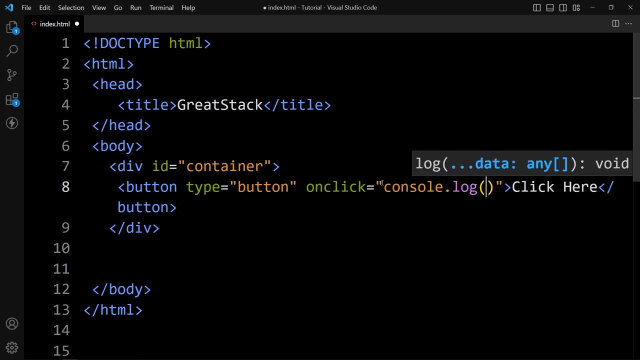 So it will log one message in the console of the browser. In this one let's add some text Here. we cannot add double quote because we have already used, So I'll add single quote. Button clicked. So this button clicked. message will be printed in the console when we click on this button. 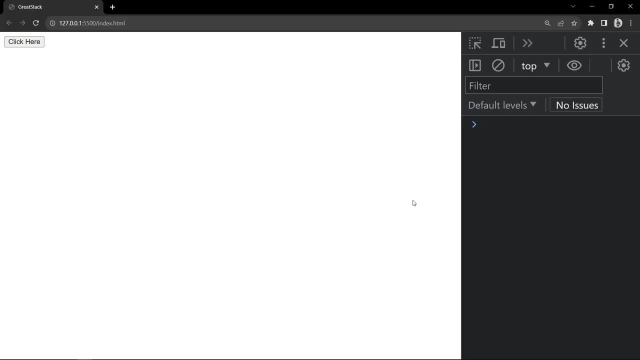 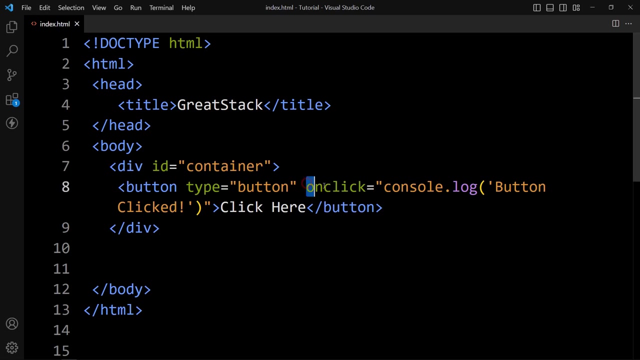 So let's see this on the web page. This console is empty right now And if I click on this button that is here in top left corner, you can see this message Button clicked. This event handler attribute can call one function also. 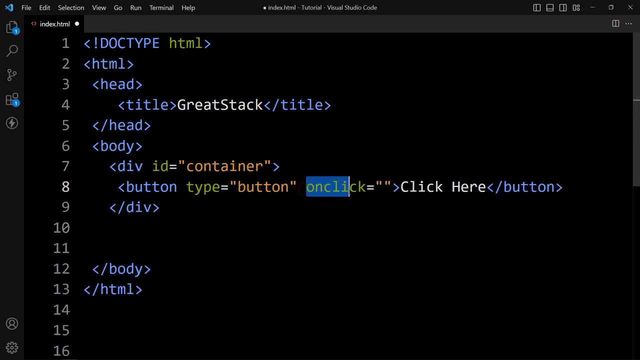 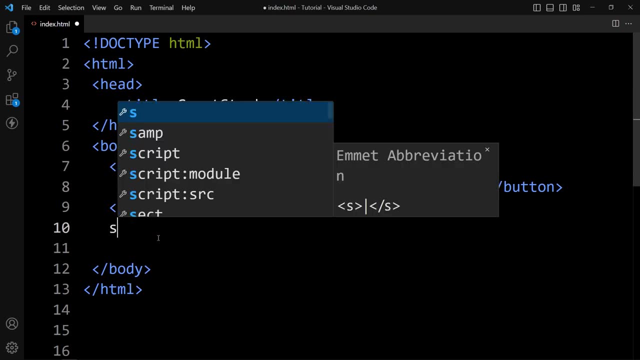 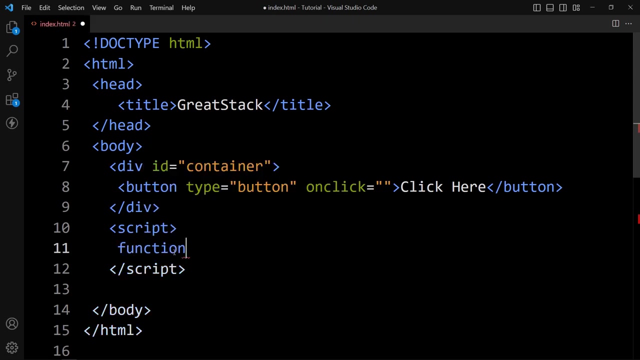 So let me remove this HTML code. We have added event handler, which is on click, and this on click will call one function. So here let's create one function in a script tag. In this script we will add one function with the name display MSG that will display message. 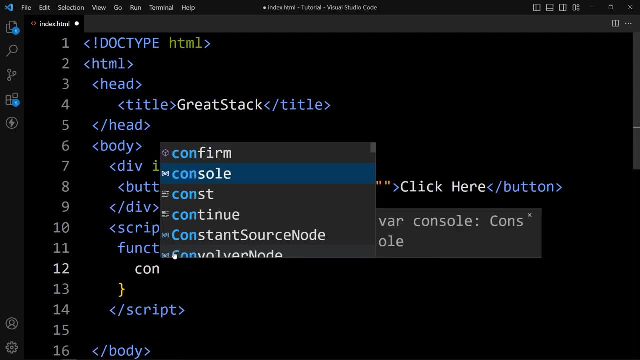 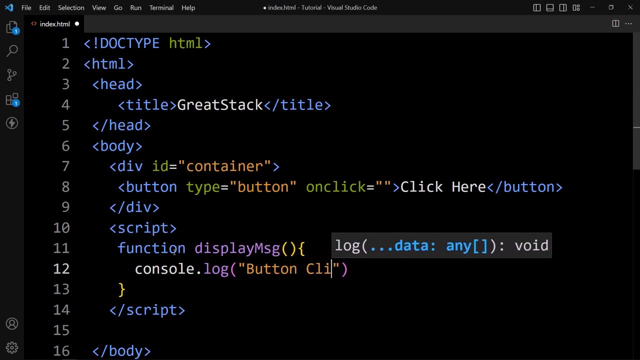 Here we will add console dot. log button clicked. Let's add some more text. Button clicked from fn, which means button clicked from function. Now we will call this function when we click on the button. So in this attribute we will call this function. 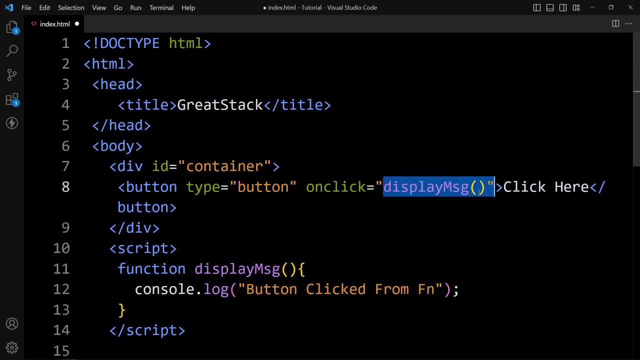 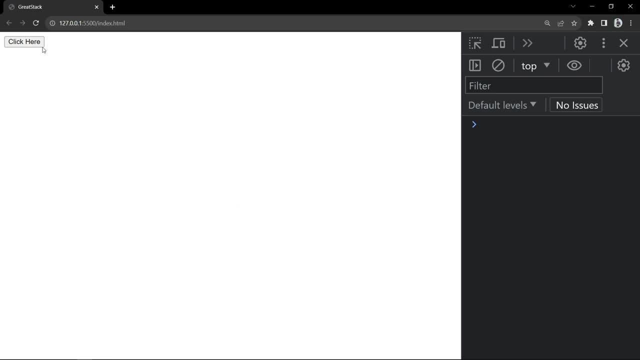 Write this function here. So this is a function call. Now let's come back and you can see this console is empty And if I click on this button again, you can see the message Here. it is saying button clicked from fn. It means button clicked from function. 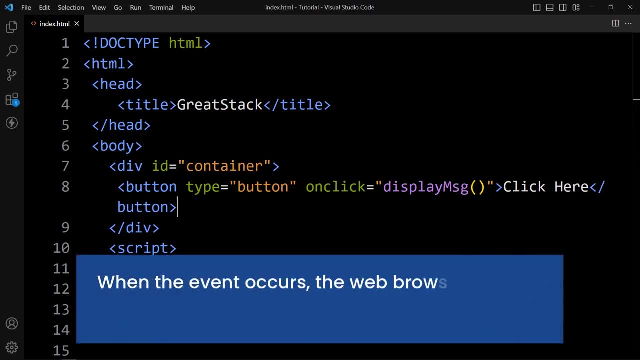 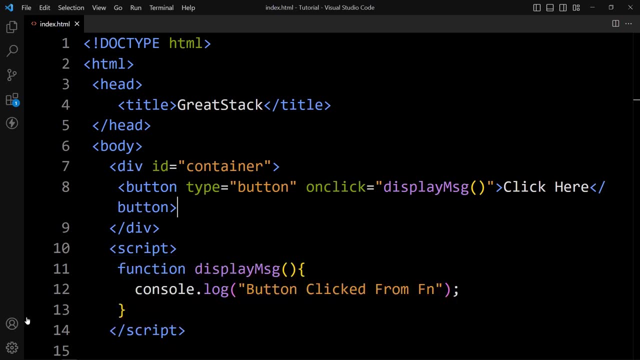 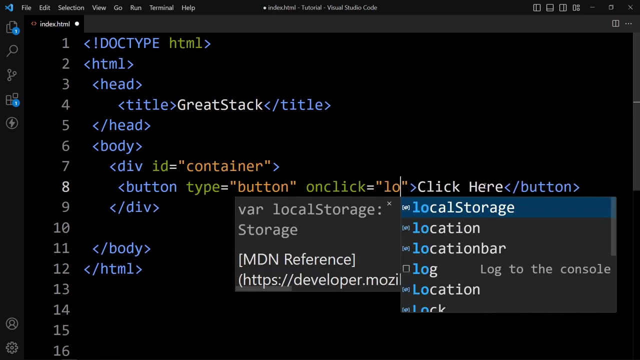 Now just come back. When the event occurs, the web browser passes an event object to the event handler. So to understand this one, let's remove this function here and we will add JavaScript code in this attribute. So here let's add console dot log. 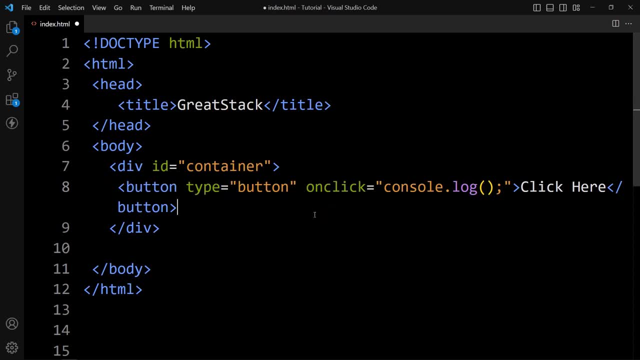 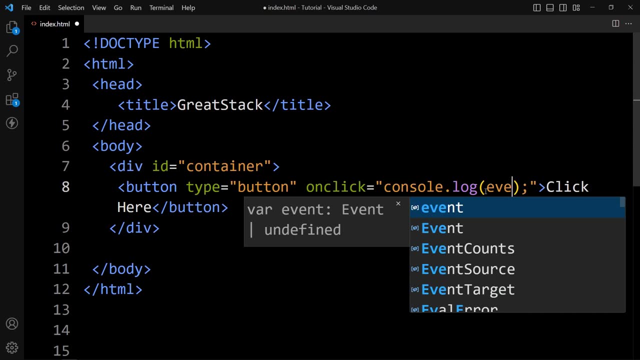 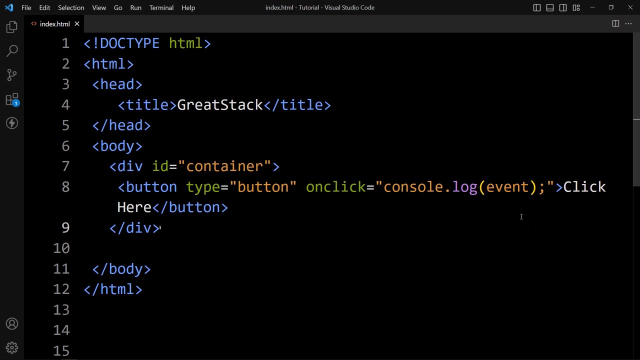 And when we click on the button, the JavaScript will pass the event object. So we can write that event object here: event. Now we can see what is there in this event object. Let's see the output So you can see here. 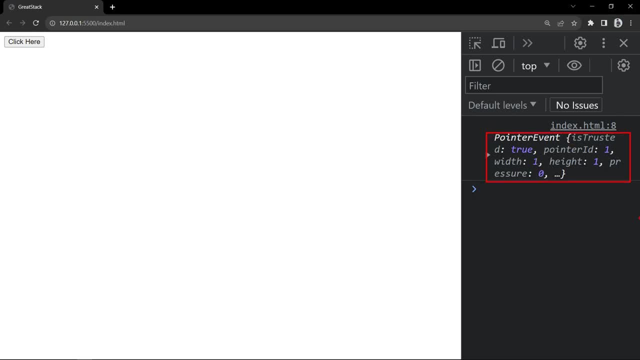 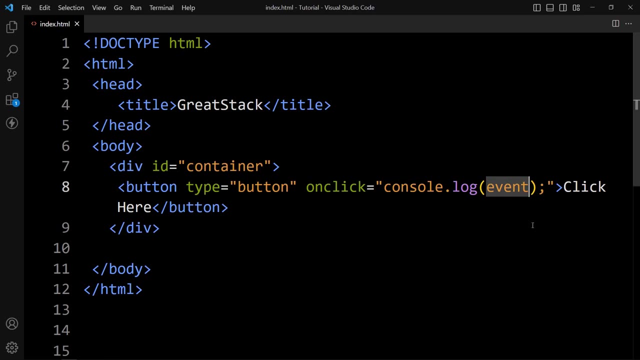 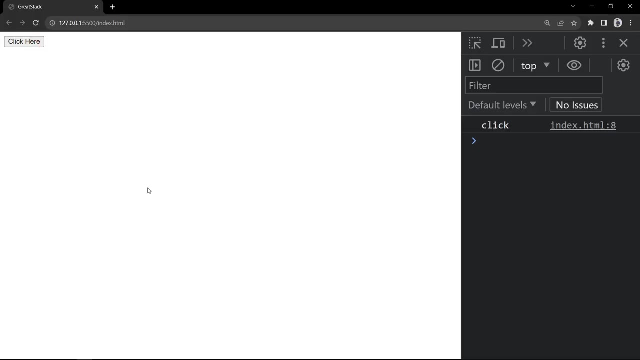 We have one object Now. this event object has some properties that we can access. So from this event we can find the type: event dot type. Let's see. It is displaying the event type. event type is click. Let's come back. 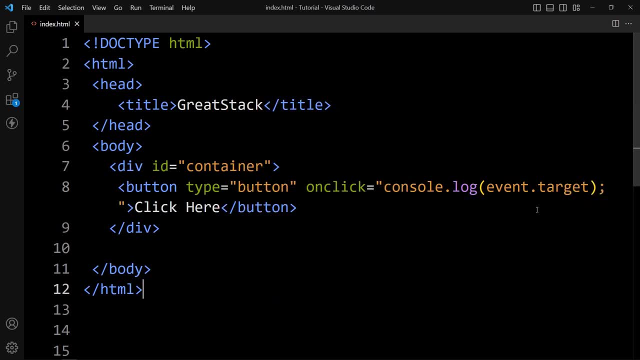 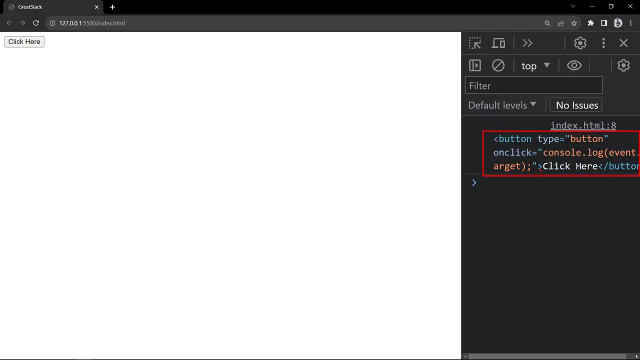 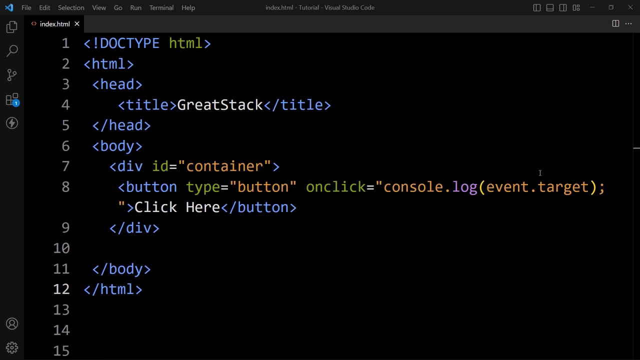 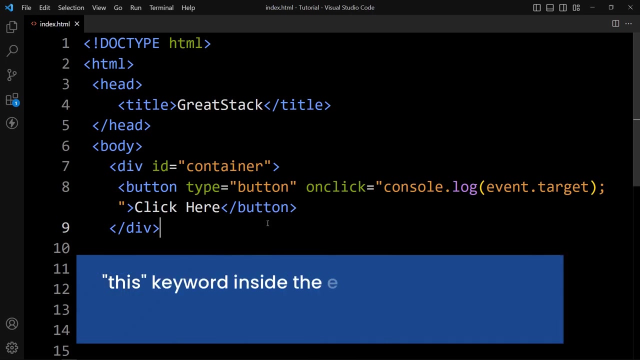 We can add the target, So we will get the target element on which the event occurs. When we clicked on the button, it is displaying the entire button element with all the attributes, So it is giving the target element. We can also use this keyword inside the event handler and this keyword inside the event. 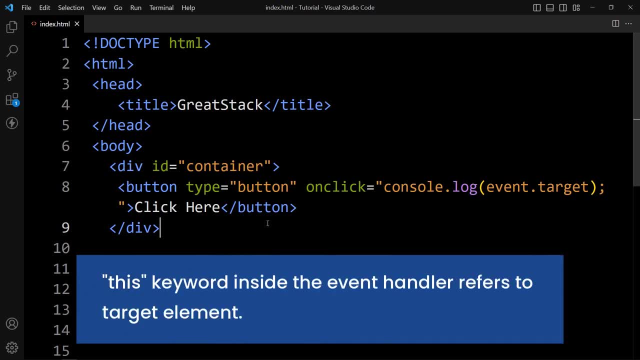 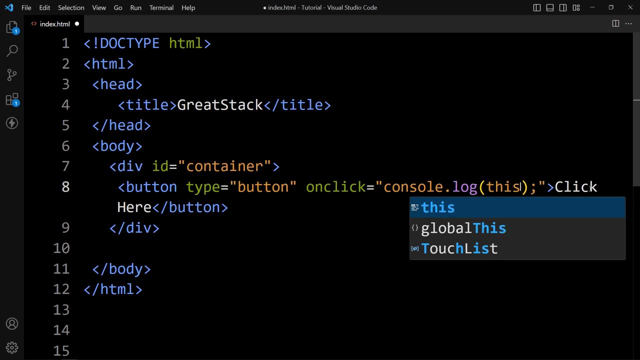 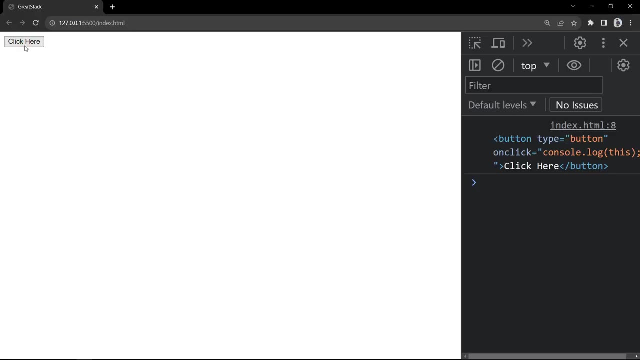 handler refers to the target element. Let's see the example here in this event handler. we will try to print this. This keyword- Let's see This keyword- will refer to the target element. Let's see the output when we click on the button. 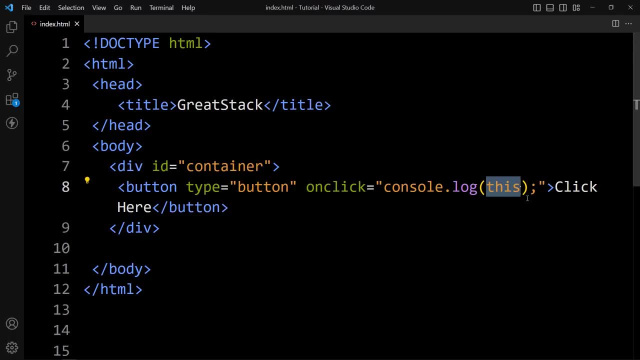 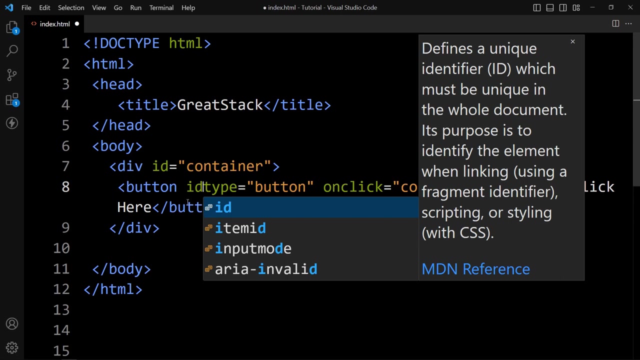 You can see again. we got the target element, which is button. So this keyword inside the event handler refers to the target element. From this keyword we can find the properties of this element. So let's add one ID here. I will add: the ID is equal to btn. 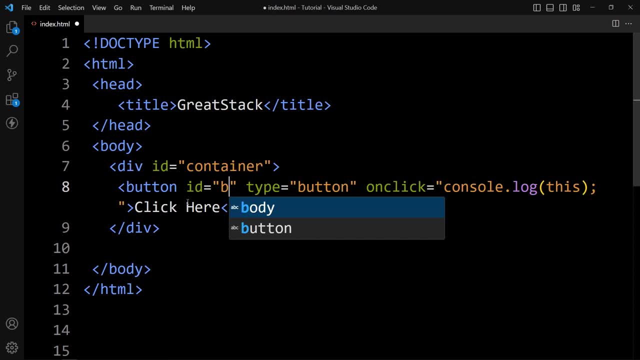 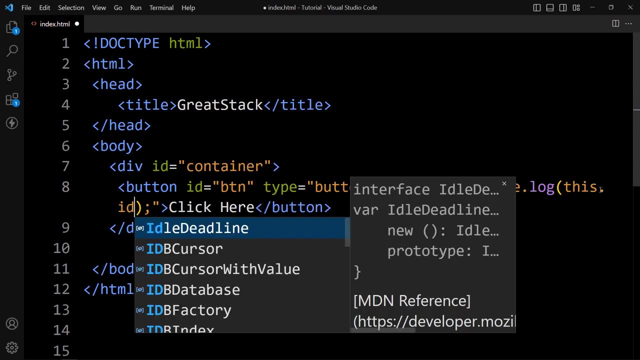 So let's add one ID here. I will add: the ID is equal to btn. So let's add one ID here. I will add: the ID is equal to btn And here we will add this dot ID. So when we will click on the button it should display the ID value. 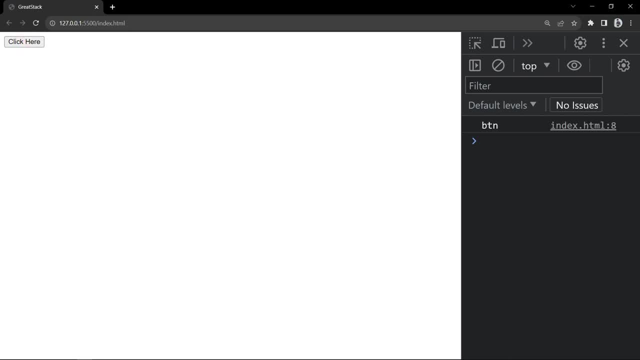 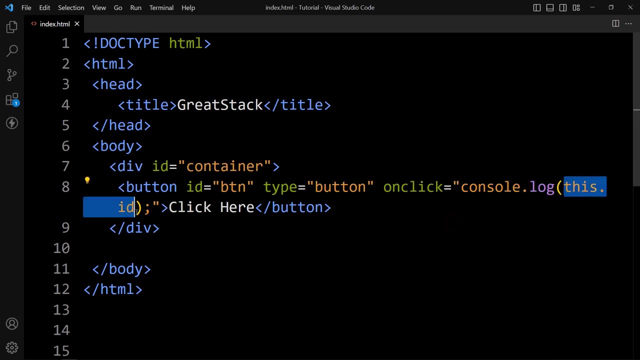 Let's see. If I click on the button, it is displaying btn. Now just come back and instead of this dot ID we can simply add ID from the event handler. We can directly access the elements property Adding console. dot log ID. 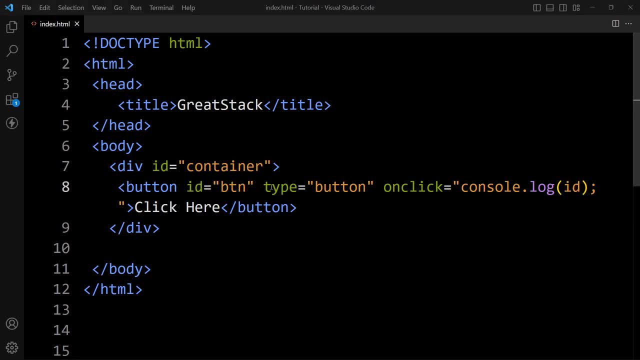 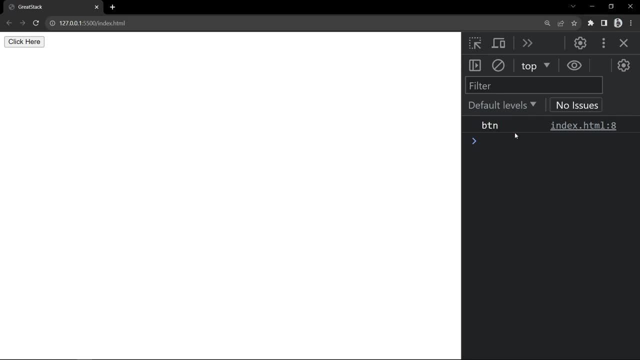 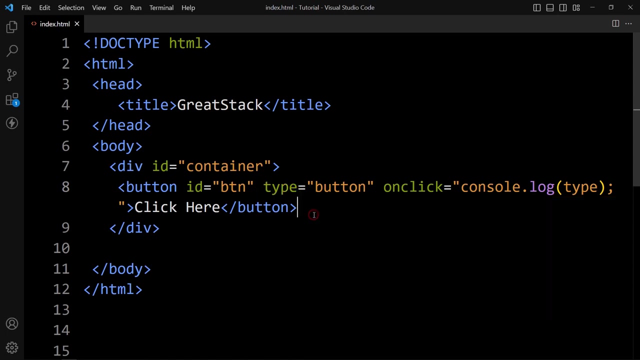 So it should display this ID value. Let's see. If I click on the button, we got the ID value, which is btn. If I type type, which is here, we will get button. It's here. So this was the first method to add the event handler. 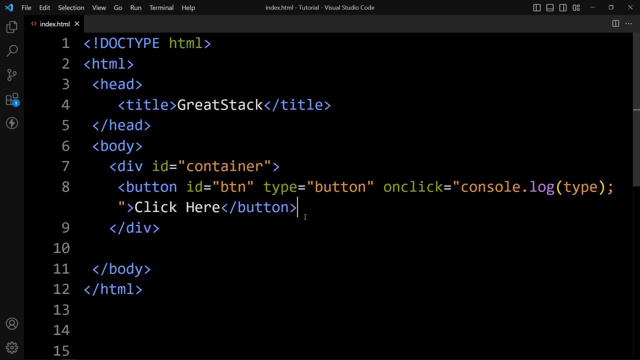 Here in HTML as HTML attributes. Now the second method is adding event handler name in the JavaScript. So let's remove this on. click from here. We have one button. Let's remove this type also. It will be simple. So we have one button with the ID btn. 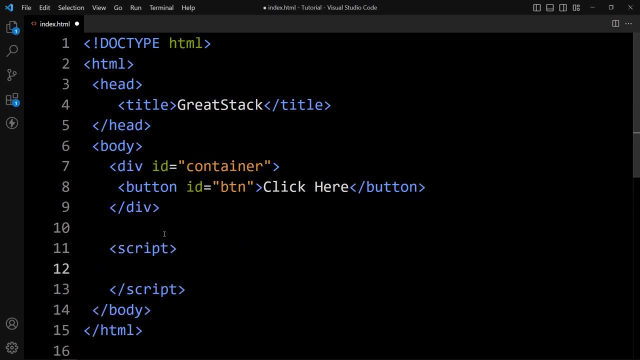 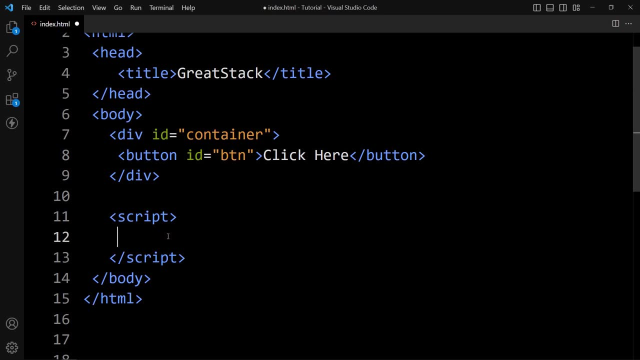 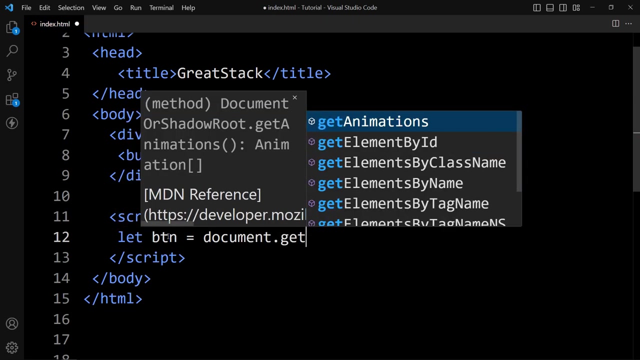 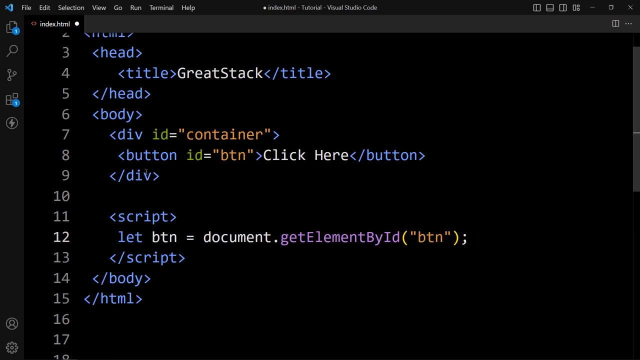 Now we will add the script where we will add the JavaScript. So within this script, first we have to select this button. So let's add let btn is equal to document dot. get element y ID and we will add the ID btn. So we have selected this button element. 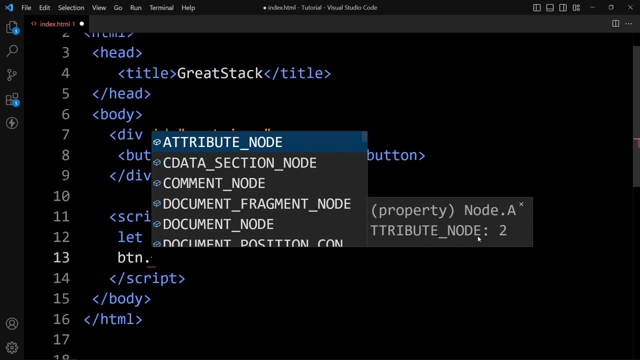 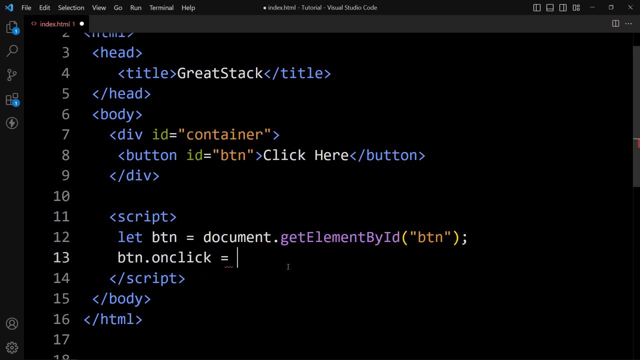 Now on this btn we can add the event handler On click, And now we can add the code that will be executed when we click on the button. So here we will create one function And within this function we will add console dot log. 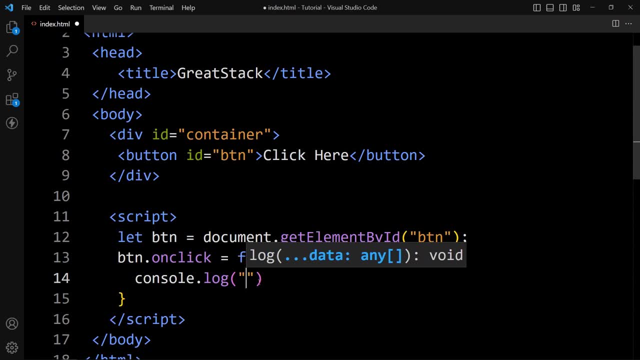 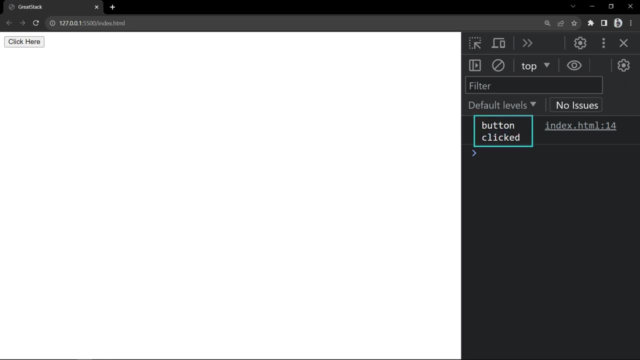 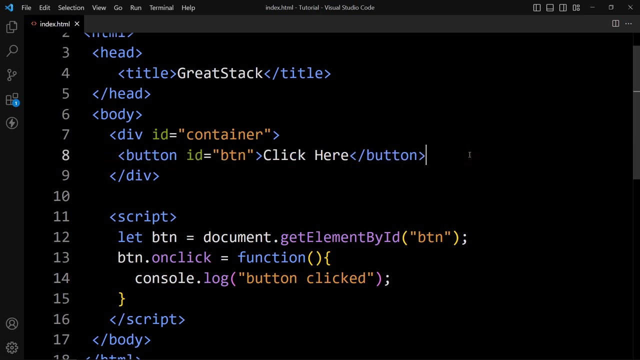 And this will print message: btn clicked. After that, let's come back to the web page. Click on the button and you can see the output in the console. Button clicked. Let's come back. You can see here we have the HTML element and in this one we have added the JavaScript. 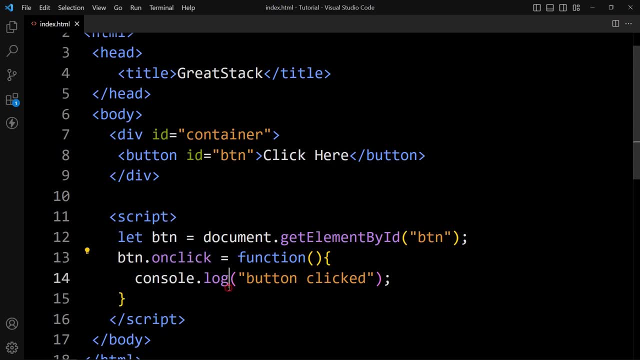 In this JavaScript We have added One click- event handler name and added one function that will display one message. Here also we can write this keyword that will refer to the target element And from this we can find the ID: This dot ID. 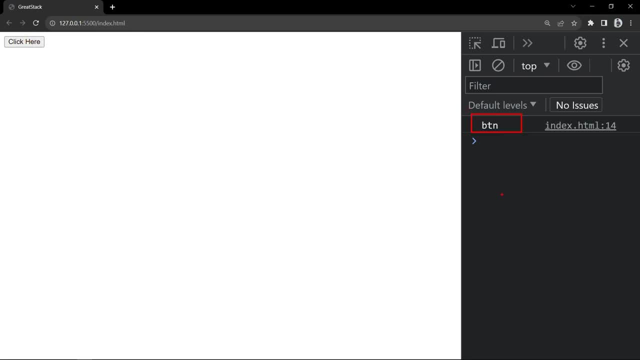 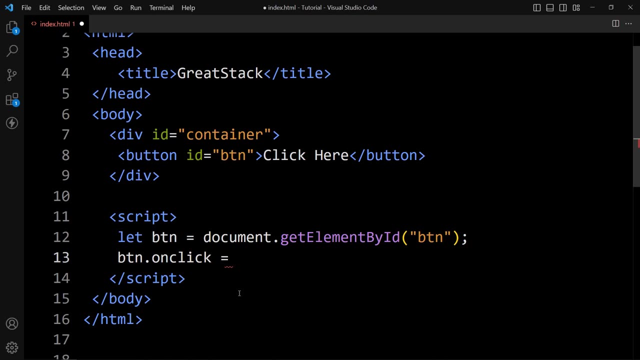 Let's see: It is btn. Now, to remove the event handler, we will simply add element which is btn. I will write btnonclick and assign null. That's it. When we assign null in this event handler, it will remove the event handler. 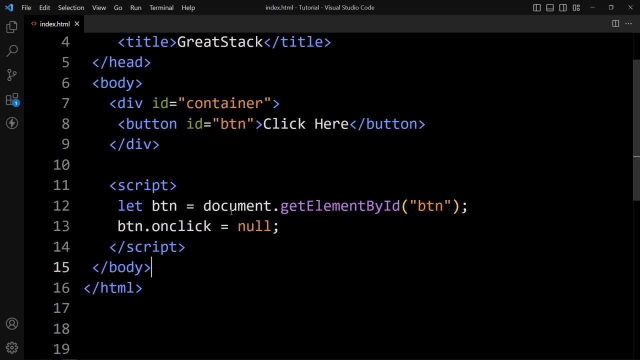 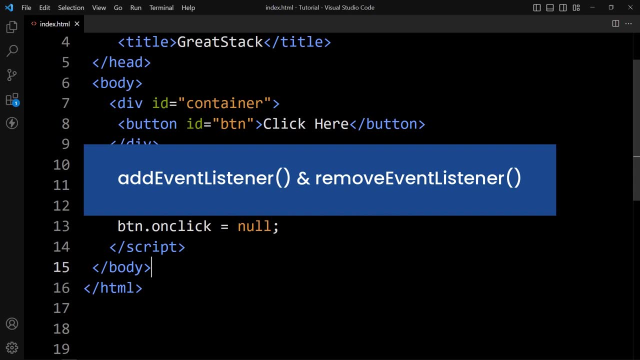 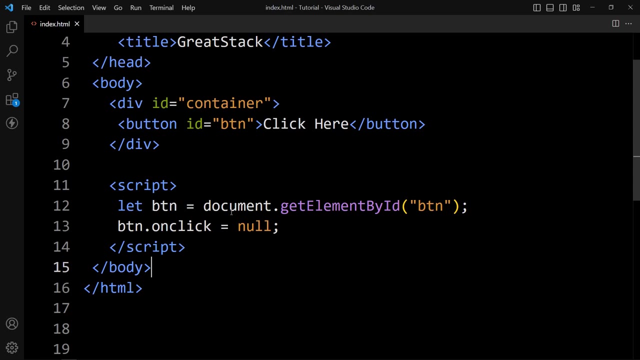 So this was the second method to assign the event handler. Now we will learn the third way of assigning event handler. So in JavaScript we have two methods with the name add event listener and remove event listener. These are two methods that handles the event. 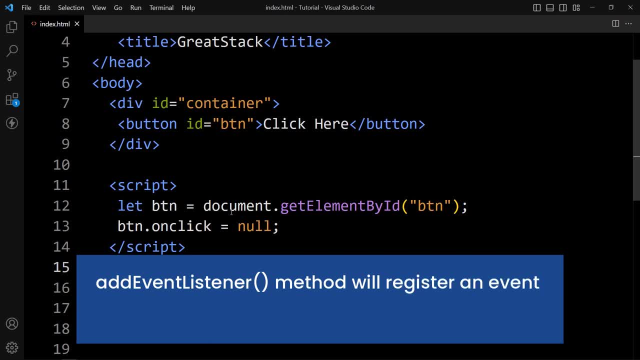 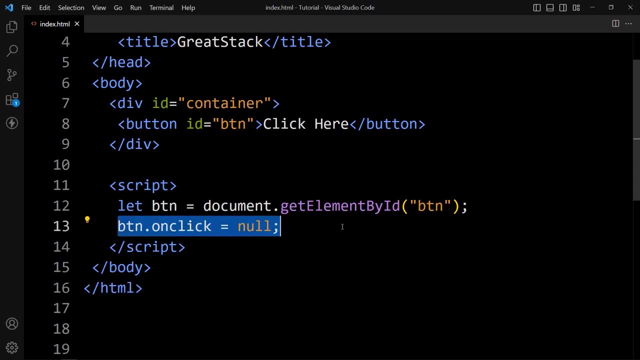 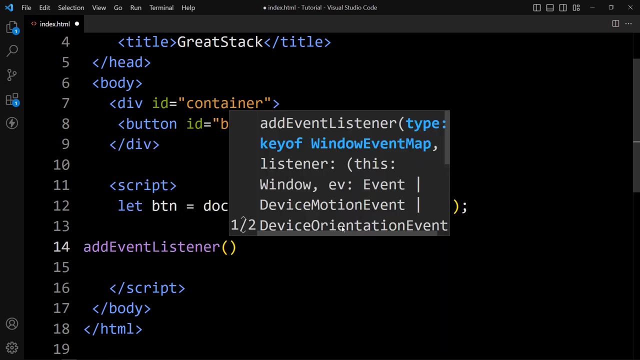 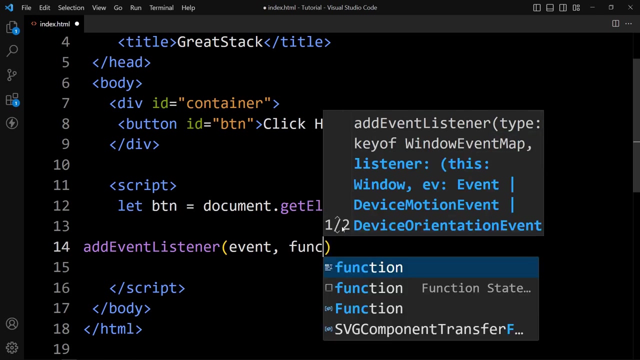 Add event listener. Add event listener, register an event handler and remove event listener will remove an event handler. so let's see the example of add event listener. the add event listener accept three arguments. the first one will be event and the second one will be one function. this function will be executed when the event fires and the 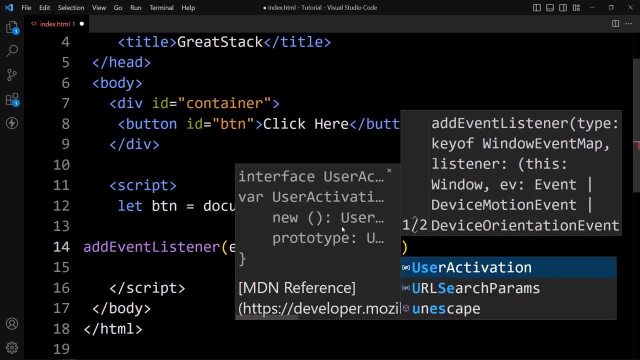 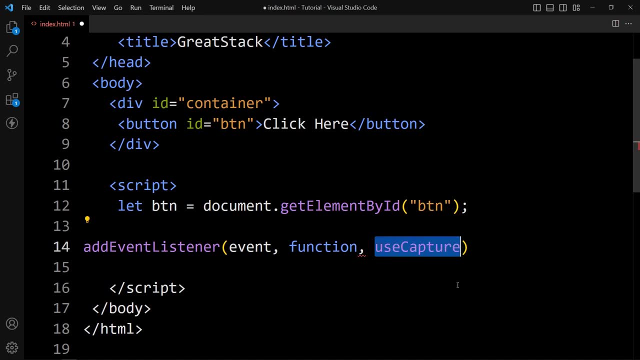 third argument is use capture. so the third option is optional because by default it is false. this use capture is a boolean value. it can be true or false. so by default it will be false and we can remove it. it is related to the event bubbling and event capturing. so let's ignore that third parameter. we will pass. 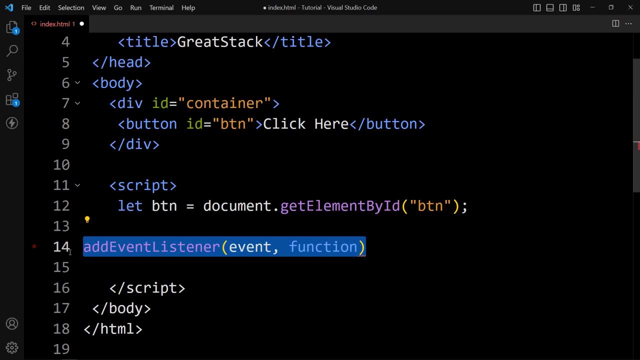 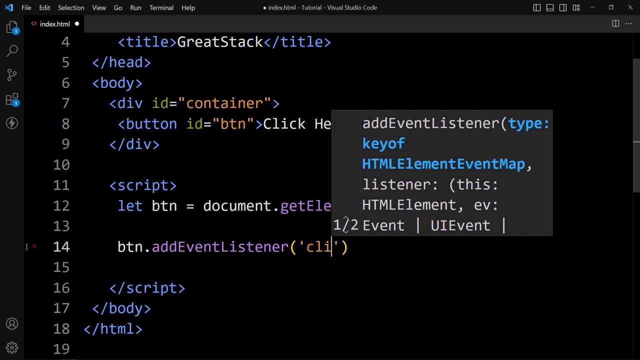 two argument, event and one function. so let's see one example. so let's try to add this: add event listener on this button. remove it. here we'll add btn dot. add event listener and we will pass first argument, which is event. so the event will be click. we are adding the. 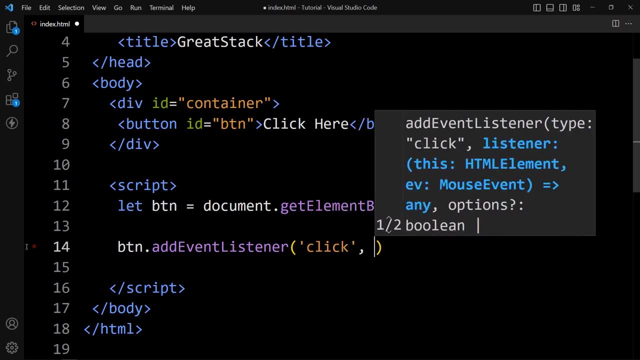 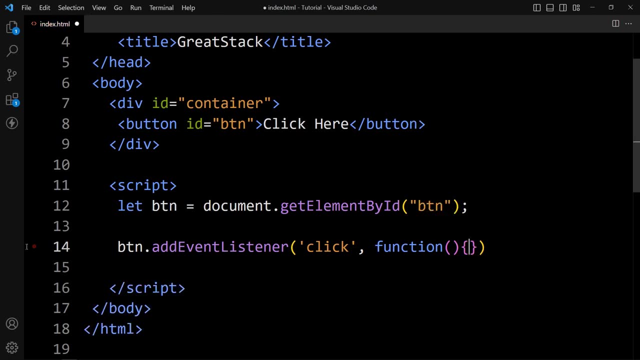 click event, then a comma. here let's define one function. here I'm adding function like this, so this is the function definition. within this curly braces we can add the code that will be executed. so here let's add console dot log and message button clicked. so we have selected the button using get element. 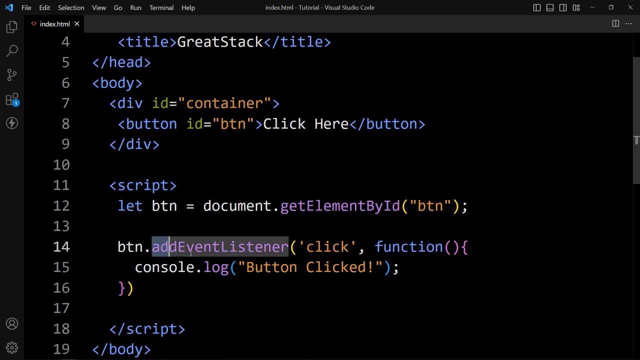 id. then on this button we are adding add event listener method that will assign the event handler. so in this event listener we are adding first parameter and second parameter. first parameter is event, so the event is click, and the second parameter is a function, so we have declared. 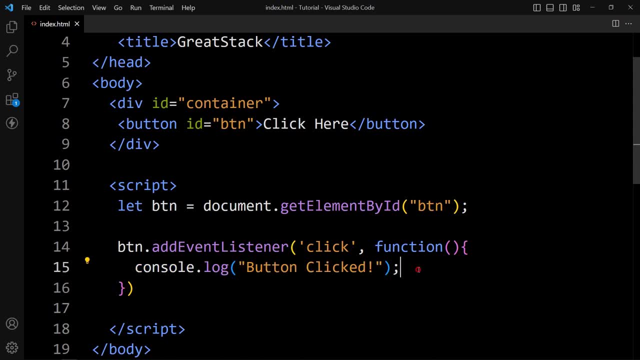 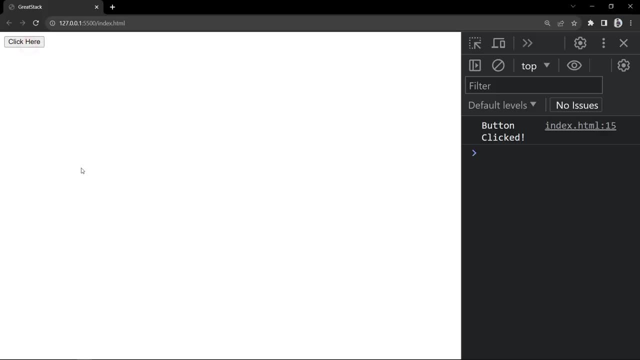 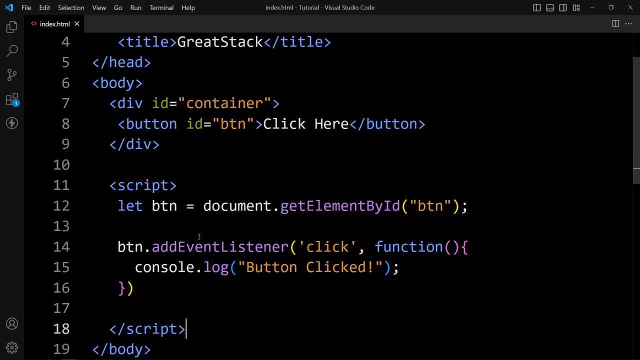 one function here. this function will print one message in the console tab when we will click on the button. let's see this output on web page. click on this button and you can see the message button clicked. as i already said, when the event occurs, the javascript passes the event object. 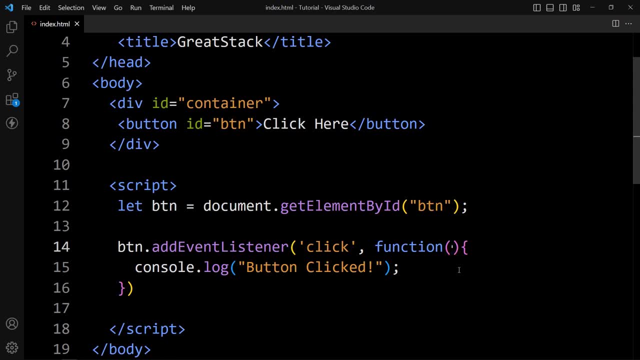 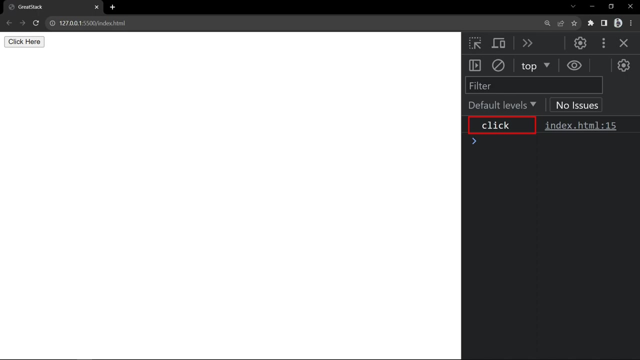 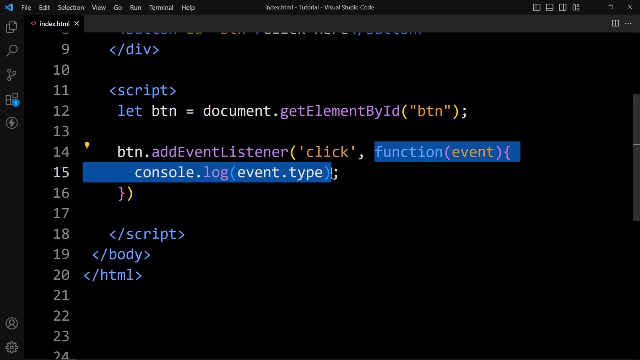 to the event handler, so in this one we can pass the event object and we can find the type from this event: event dot type. let's see the output. if i click on the button, we got event type, which is click. now, instead of adding this anonymous function, we can add the external named function also. 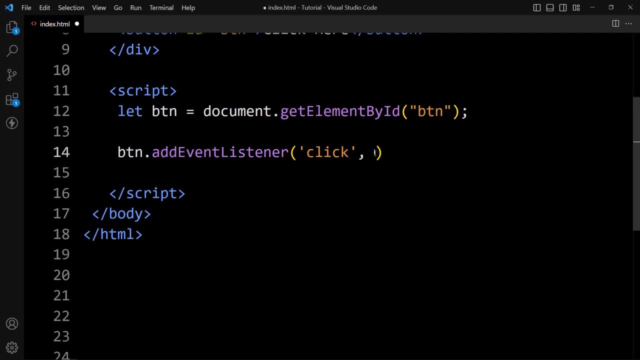 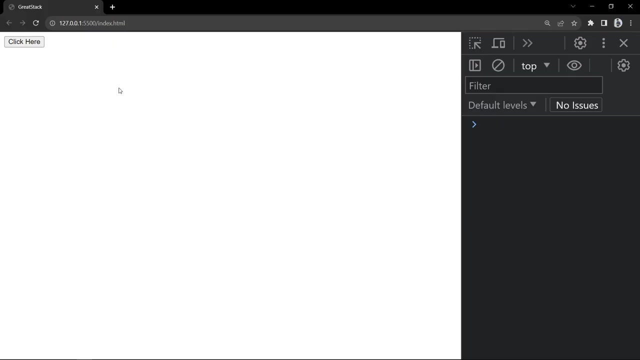 so let's remove it. here we can add our second parameter. before adding that second parameter, let's create one function with the name so display message, and this display message will log one message button clicked. now we can refer this display message function here like this: after adding this, let's come back and if i click on the button again, you can see the message. 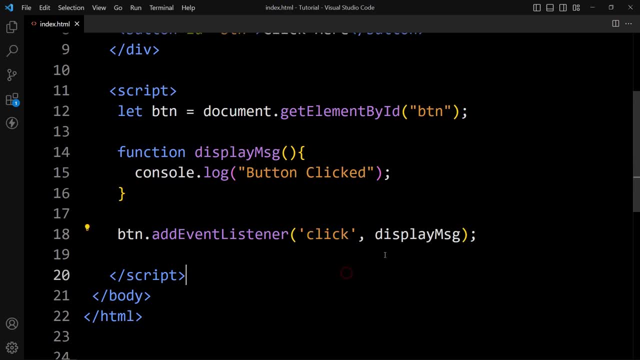 button clicked and we can see the display message function here. like this button clicked so we can add the event name and one function. it can be a anonymous function or it can be a named external function. we can refer to that external name function with the function name. 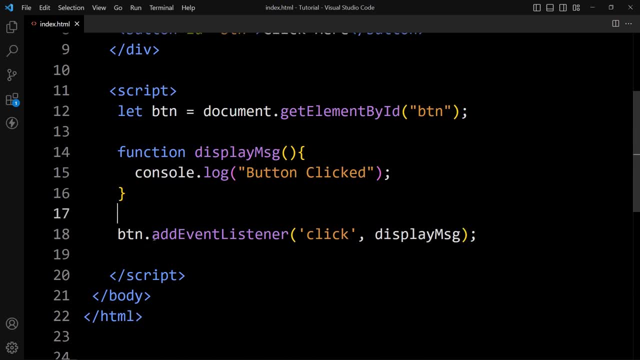 without the parenthesis. so this was add event listener method. now we will learn the remove event listener method. the remove event listener removes an event listener that was added using add event listener. so here we have added the event listener using add event listener method. now we can remove it using 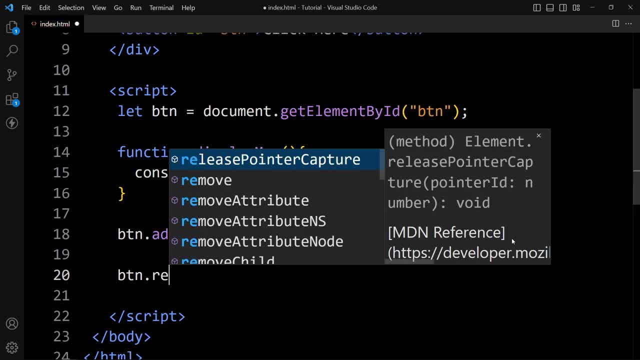 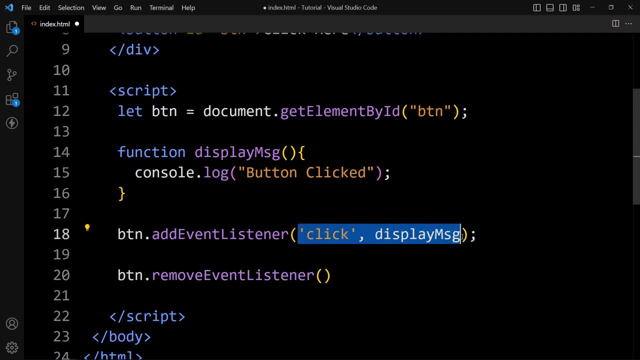 btn dot. remove event listener. again we have to pass the same arguments, just copy and paste it here. so this remove event listener will remove the event listener that was added using this add event listener. you can see here i have added the external named function. if i add one anonymous. 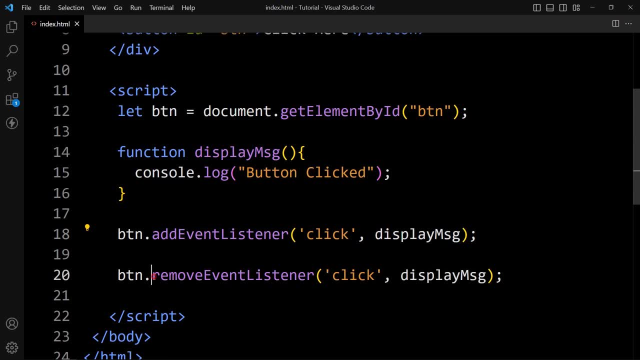 function here, then we cannot remove that event listener using this method, so we have to use the external named function when we want to add the event listener and remove the event listener. now let's know about some of the useful javascript events. so the first one is mouse- move event mouse. 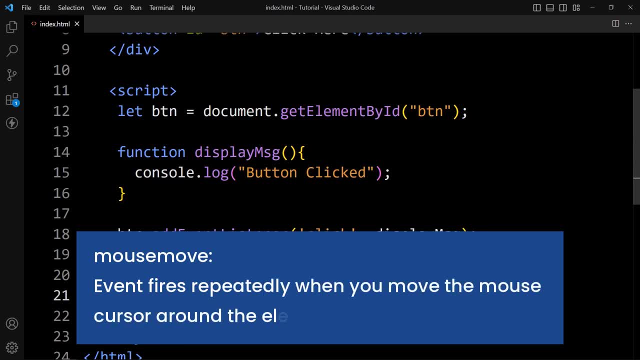 move event fires repeatedly when you move the mouse cursor around the element. and second one is mouse down event: when you press the mouse button on the element, this event will fire. next one is mouse up: when you release the mouse button on the element, then this event will fire. 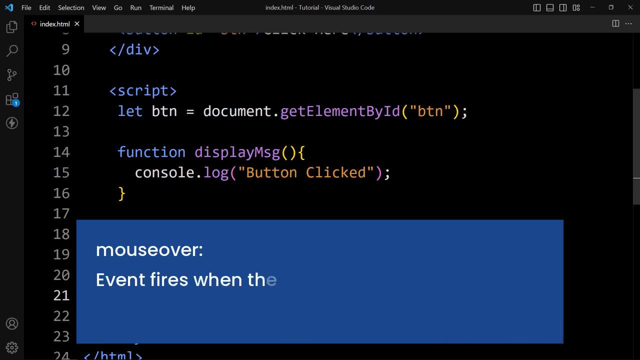 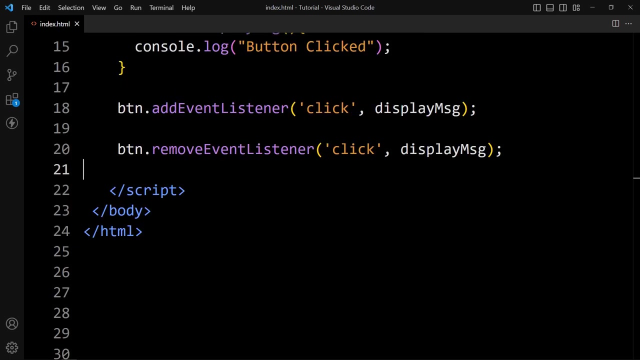 next event is mouse over event. when the mouse cursor move from outside to inside the bound of the element, then mouse over event occurs. next one is mouse out: when the mouse cursor is over an element, then moves to another element, then mouse out event occurs. next one is key down event key. 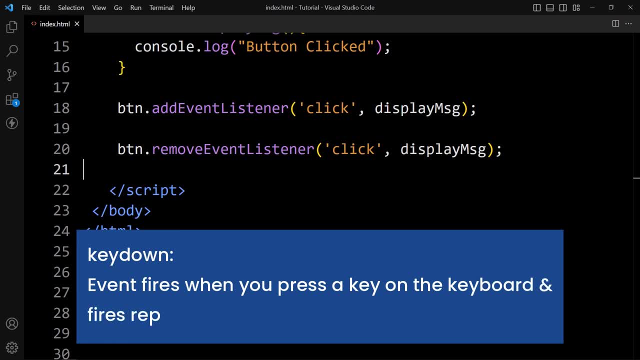 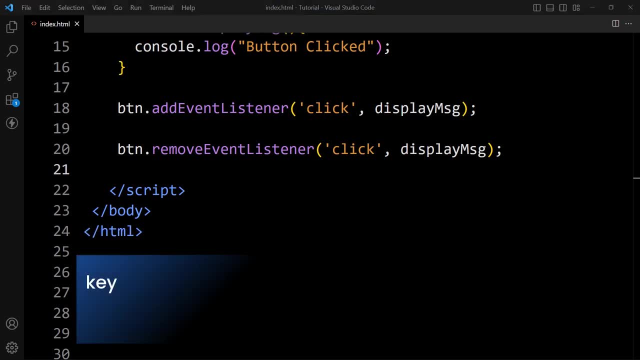 down event fires when you press the key on the keyboard and it fires repeatedly while you are holding down the key. next one is key up and forth whatever things you have to do to allow this effect key up event. this key up event fires when you release a key on keyboard. next one is key press.